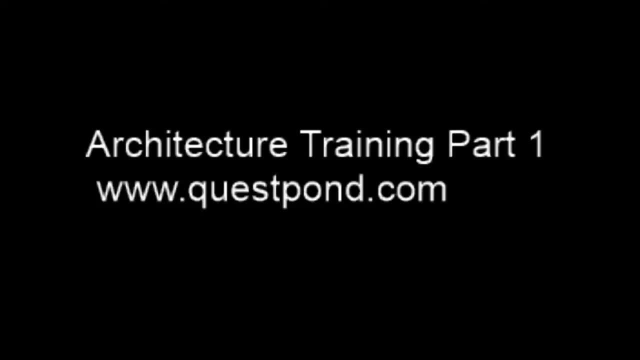 Okay, good evening, I am live. Let me know if you can hear my voice, if you can see my screen. So good evening. Piyush Indarjit, Vinit Sabyashi, Aditya Rahul and lot of people out there. 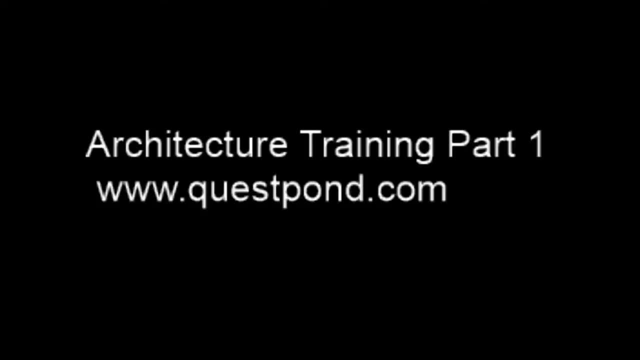 Let me know if you can hear my voice. So today we are talking about architecture. So, inside Questpond, every Tuesday, we have launched this architecture course where I will be going, and it will be a one hour of training every week, which will happen inside Questpond, where we will be talking about architecture, design patterns, UML, how to estimate a project and lots of those small, small architecture patterns like onion architecture, repository pattern and so on. 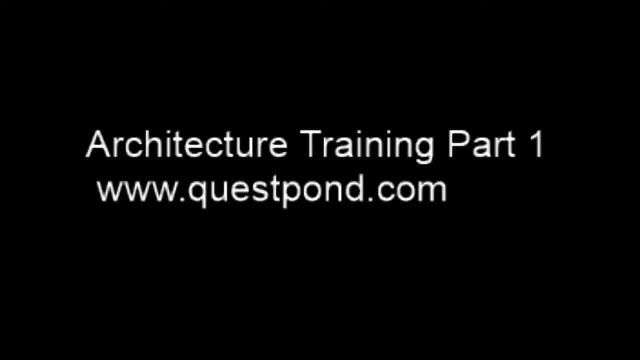 But I thought that why not make the first part of the training free and discuss with people and give a kickstart? So Tuesday in Questpond we are having the architecture training. Thursday we are having MVC Angular training. Saturday we are having AZ20 for Azure training. 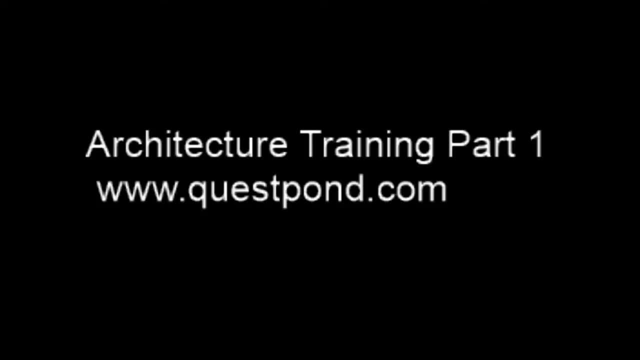 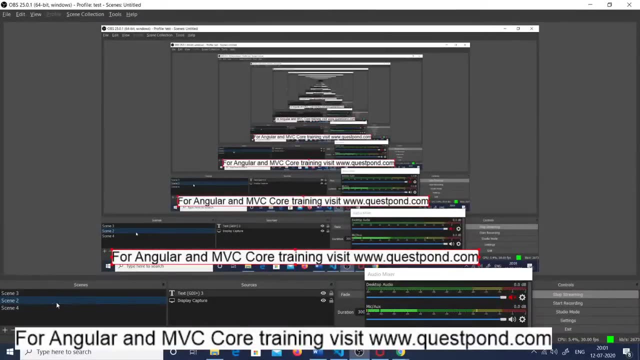 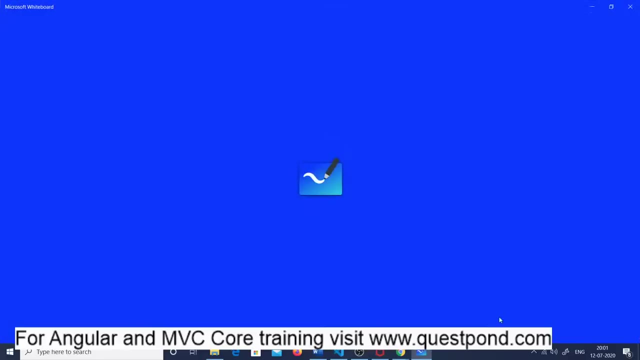 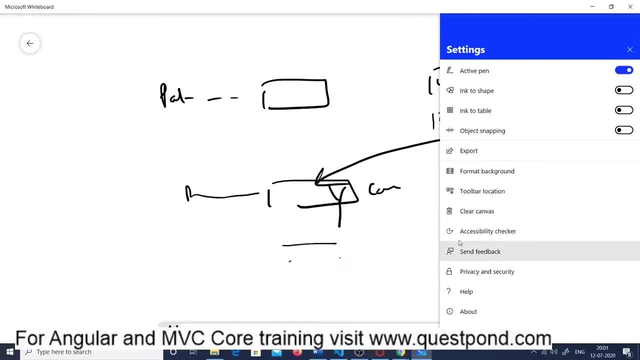 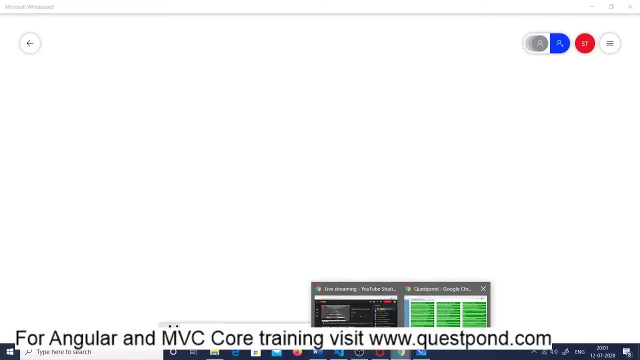 Good evening and let us get started. So first thing, let me go and share my screen and so I am going to go and just on my screen out here, and so, first thing, I am sorry for that zoom which comes out. So first thing, when someone says that he wants to become an architect, right. so first thing, guys, very quickly, you know, inside Questpond, people who are Questpond members, you know, do go ahead and see the design pattern series. we have learn design pattern step by step. 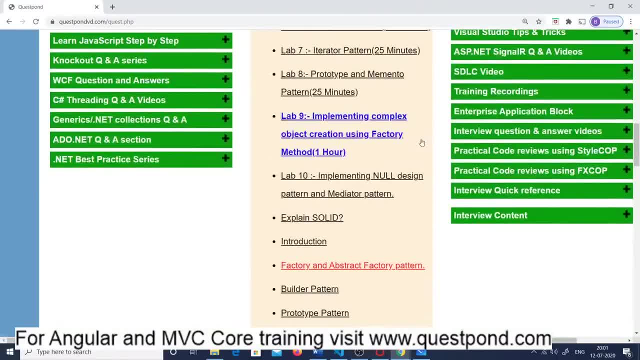 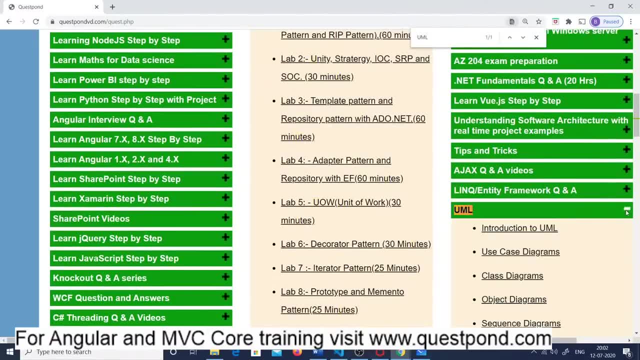 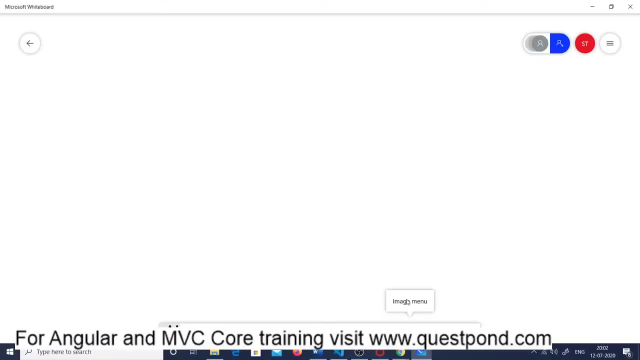 We have the architecture series right and we have completed almost all the patterns. We have the UML series. Go and see unified modeling language, how to do it, and so on. right coming to like: what does it take to make an architect? someone says, okay, you want to become. 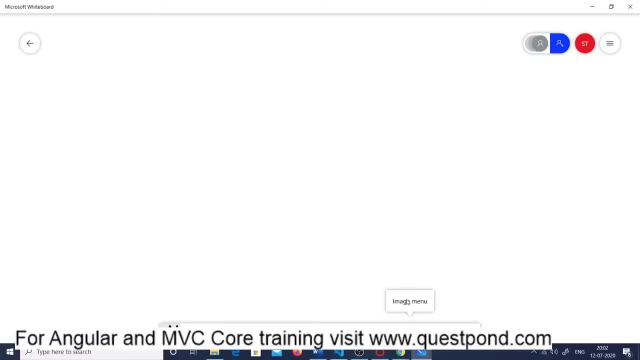 an architect, so lot of people will say that, okay, so learn like lot of design patterns, is it? learn lot of architecture pattern, is it? or like you should know how to do UML, right, or must be? you should know something else, right? so you will see that you know lot of. 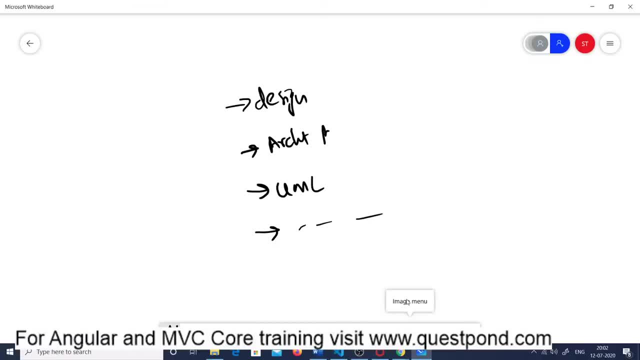 people have different ways of looking at an architect. that why is a person an architect? but here it is very quickly. first thing. the reality is that in our software industry there isn't any real definition of a software architect. frankly, I know that lot of people say that he is a solution architect and he is an enterprise architect. the way a project 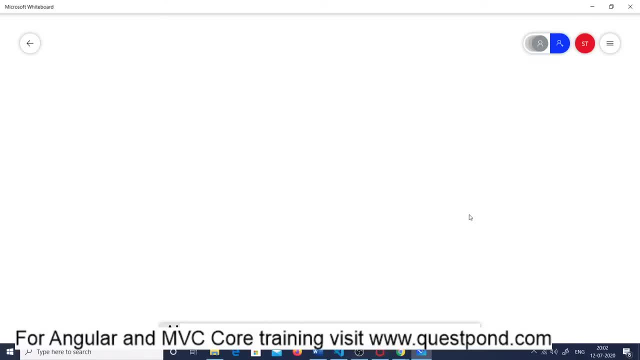 manager's rules are fixed. if you look at a project manager's rules, you will find that the job role is fixed: he has to do estimation or he has to do projects. if you look at project manager's rules, you will find that he has to do estimation or he has to do projects. 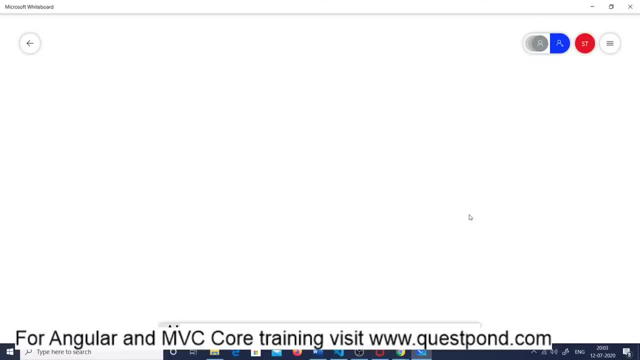 management. he has to allocate resources, he has to do people management. things are pretty much clear right out there and even you have so many certifications out there which, like you know, the pmi and so on, which really makes that thing very streamlined. but believe me that when you say that, 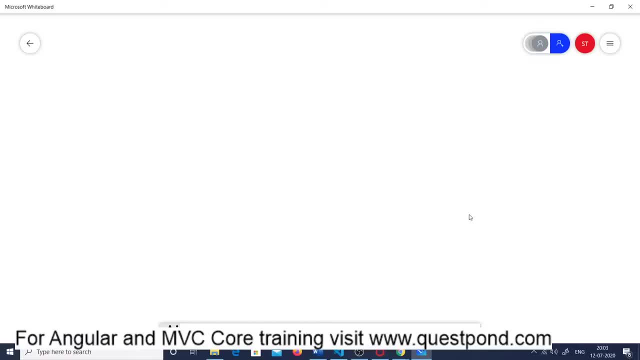 a person is an architect company. people are completely confused. i have seen- i am talking about india, because i have been working most of my time in india- in india, you will find that a person is an architect. he is also coding. you know like it's so strange, you know. so it's not that the 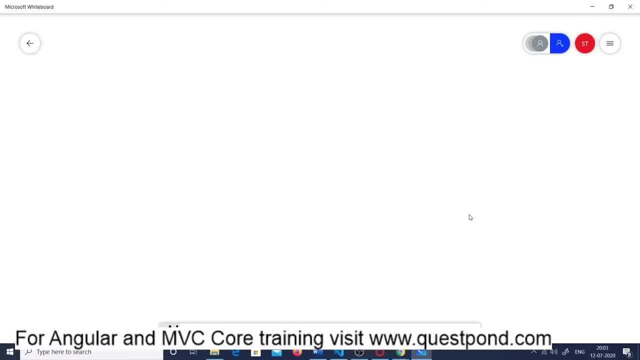 architect should not code. but the point is that, you know, architect has a different kind of role in our organization, right? so the question, but first thing comes out here is that: what does it make to make an architect right? the first thing is, when you say a person is an architect, right? 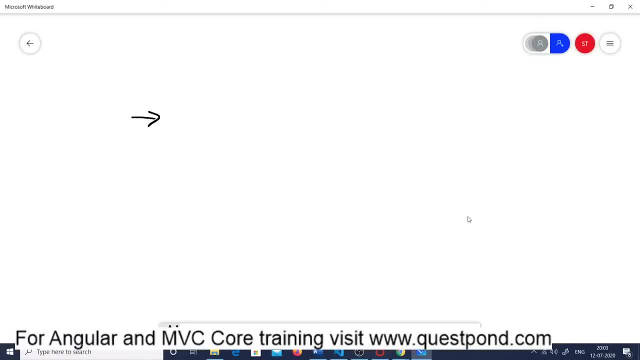 one important delivery of an architect is: you know, if you, if you say that, okay, this is my project, right, he should be able to give a proper you technical roadmap, a proper technical roadmap of how the project will be structured, what kind of components the project will have, what kind of. if you say that the performance has to be, 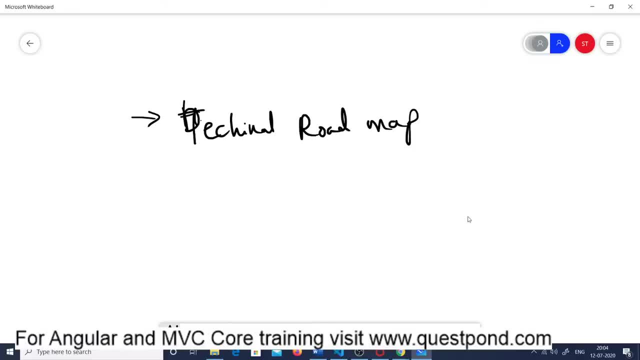 awesome. then what should be the thought process, right? what kind of database we have to select, even the selection of the stack, right? so when you say that a person is an architect, the first expectation, if it's a new project, the first expectation is that he should write a. 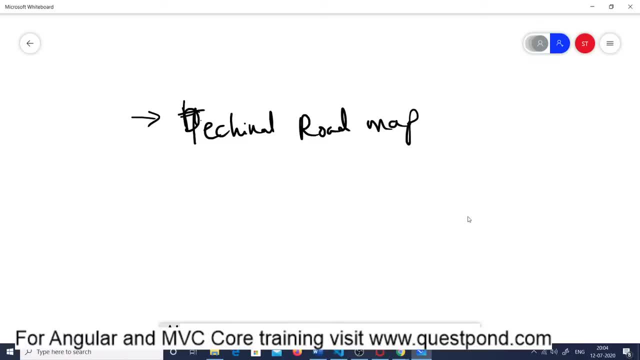 technical document, or he should actually give a roadmap to all the developers that how the project will be structured. that is what at least i expect from an architect. and when i say a roadmap means not only in terms of classes and objects and database design, but in terms of also infrastructure. 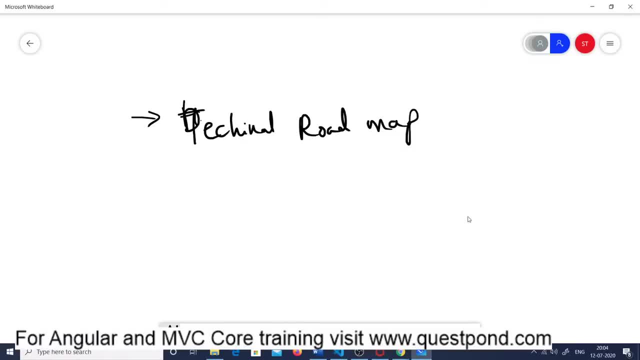 in terms of that, how to meet the requirement right now. if you say a person who has to give a technical roadmap to you know, in a design document, right, the first thing is that, how should he start thinking right, what should be his thought process? so i think that the first thing, i'll just give you an 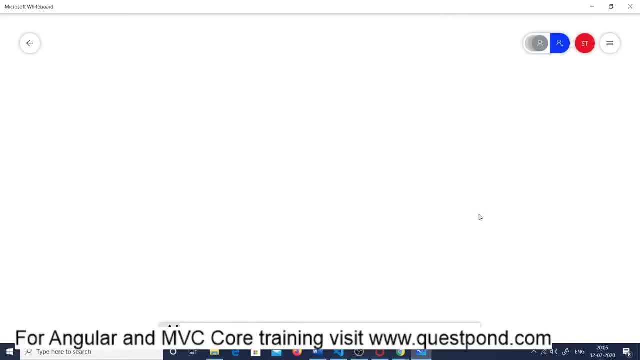 idea that what i feel an architect should be doing is, first thing, is his object-oriented programming principles. you know, should not be cleared, you know, from the point of view of, just just like you know, theoretical, you know, but it should be cleared from the point of view it should. 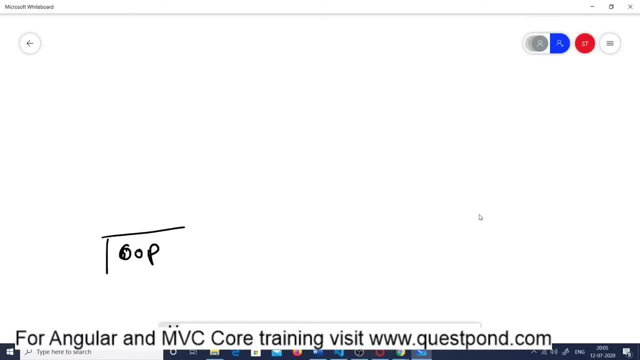 be clear from the point of view of, uh, even applying in an in application, right? so first, i think, object-oriented programming, definitely. i look, look at his database design. it should be very crisp and clear if you say that you have to. you are looking for such kind of a. 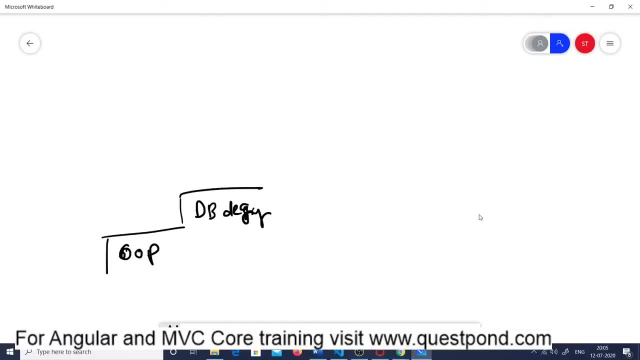 structure. he should know normalization, he should know denormalization and so on. right, definitely, i look at design patterns as one of the tools. again, right, i'm not saying that he has to know every design pattern, uh, with every word out there, set by gang of four, but he should have an. 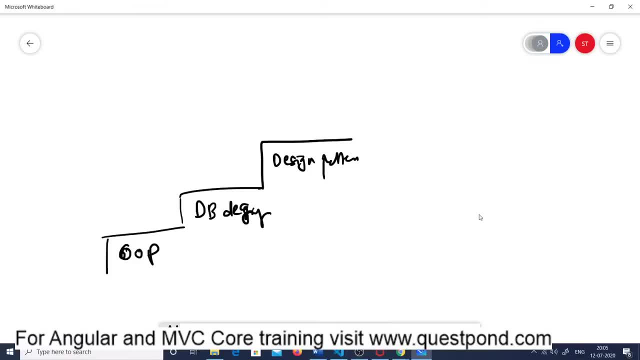 idea that, okay, this is the place i will apply mediator pattern, this is the place i will apply singleton pattern, not definitions. again i'm saying: but he should really know that it should just come naturally. so if i look at an architect, the design pattern should actually pop up naturally saying that, okay, this is the problem. 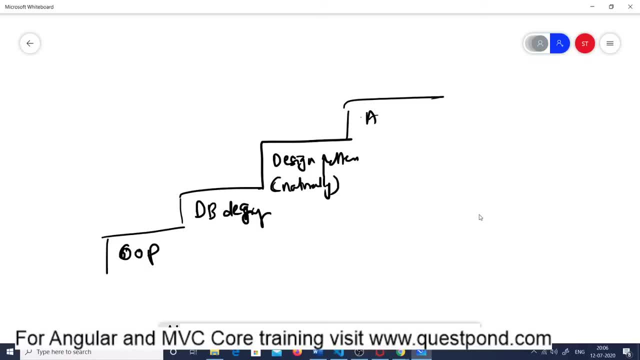 must be. this is a solution out there, right. architecture patterns: definitely, he should be very well versed with the different kind of architects, architectures, that is, that is available right from your simple mvc to multi-layer and, and you know, the service-oriented architecture, the rest kind of architecture, right? so that's again i i feel so, one of the things you know. 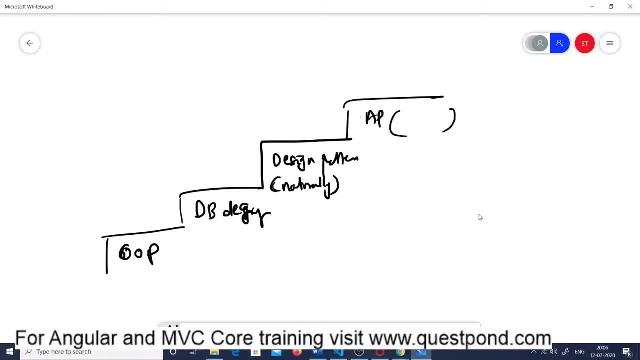 which i also feel is that he should also know how to do proper estimation. these are, like i will say, not technical skills, but, as an architect, sometimes you know we go and visit with those pre-sales person, pre-sale people or we are talking with the project manager- he should know how to do, how you should do estimation, how you should calculate. 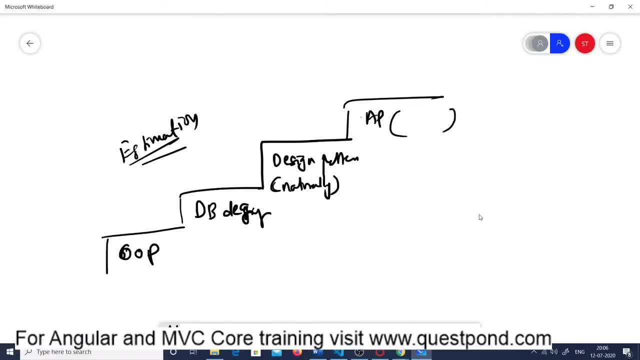 the mandate. so if somebody say this is the screen to be made and these kind of requirements are there, then how do i go and calculate mandates from it? right? so when i say estimation in terms of- again like when i say estimation, it should not be estimation, which is a guesswork. so i have seen a lot of developers out there, if you ask him. okay, if i 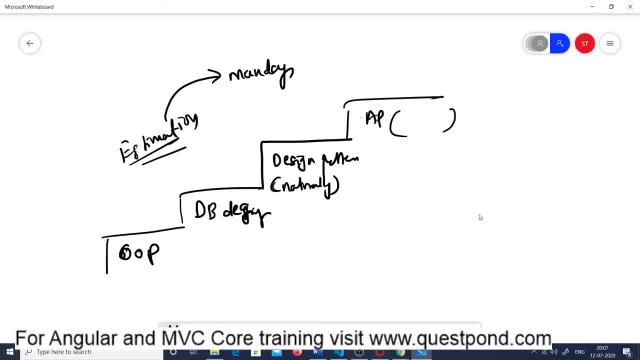 want to make this screen. he will like say, okay, it can be six days, but you know what, if you, if let us say i have to make that in this way, then it can be 12 days. so not that kind of estimation. so estimation should be really scientific. so must be, he should be used, he should use some proper. 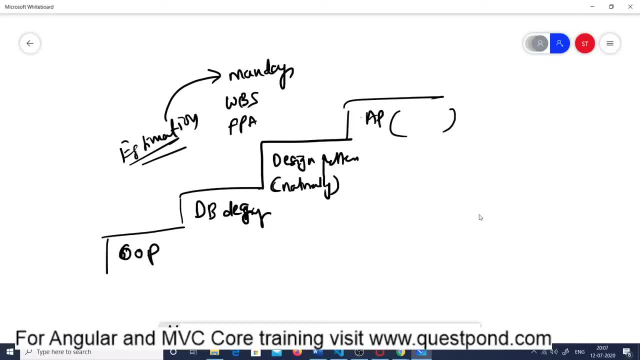 methodology like wbs, or must be function point or must be agile stories. i don't know story points, you know. so that should be a problem, proper, quantifiable kind of estimation way. he should also know right. he should be able to express himself unified modeling language, so when he goes and he talks with a developer. 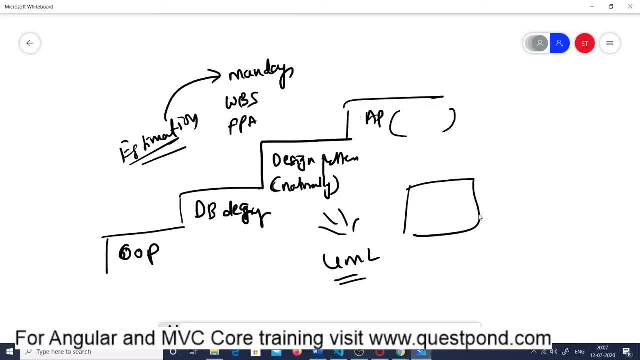 out there. it should not be like saying that, okay, think about that, this is a class. so you can't just draw a rectangle out there and say it's a class, must be. you should draw a proper class diagram. you should say, okay, this is a customer class, this goes and inherits. 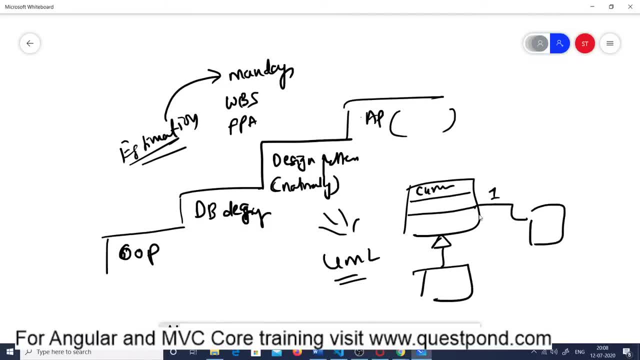 this. this goes and has a one-to-many relationship to class diagrams, sequence diagrams, writing use cases at a basic level, right, how to? so i feel that when i look at an architect right out there who is really a person who can deliver a project, right i, i feel that it's not only 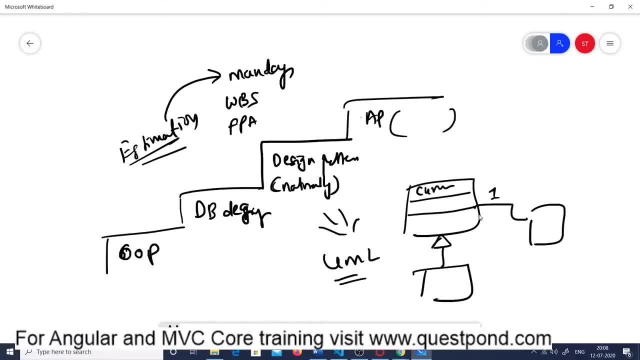 technical, but also a lot of non-technical things which should also come out there. right, and also- yes, you know nowadays this- cloud and infrastructure. i'll just put all this into one basket: the cloud, the infrastructure. right, and using this, he should create that technical roadmap and not only create a technical. 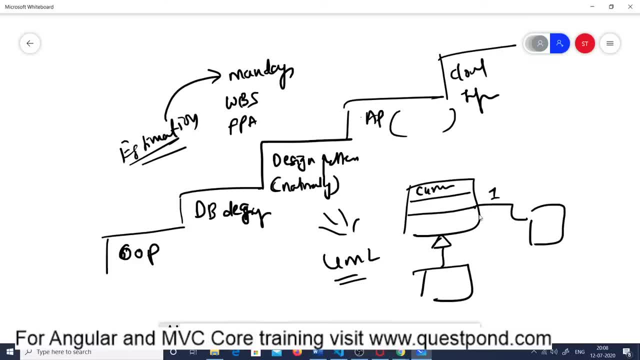 roadmap. now remember, i've seen a lot of architects out there who create a technical document which no one can understand. he starts stuffing adapter pattern and factory pattern and then you have a junior down out there who has just passed out from the college, who just knows cloud application, and you tell him: hey, like this is factory pattern implemented. it is. 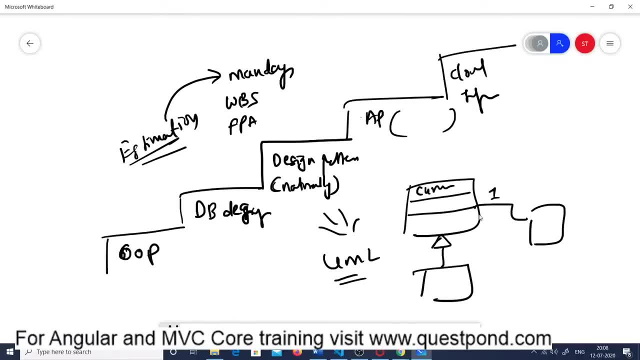 not possible. so he should be able to also communicate to his developer. your, our developers are our army. if you, if your commands are not understood, understood to them right, how do you expect the project to be delivered right? so i feel that an architect should you know, really have. 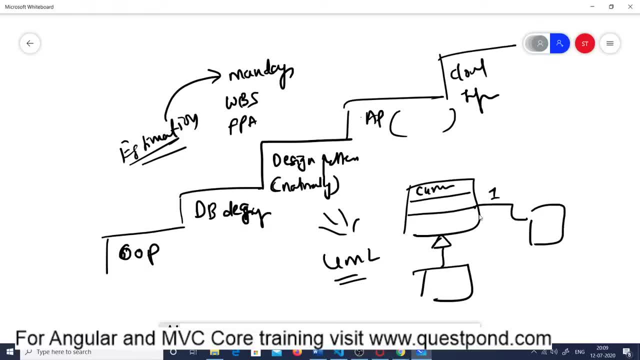 and you know, have this multi-skill kind of one thing, and that's what makes a person architect right. so that's the first point which i want to highlight out here in this course. now the second thing which i really want to make a point out here is the the most important thing. 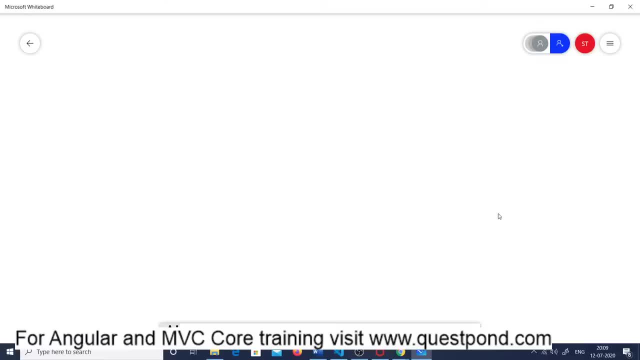 an architect should really do is when he starts designing his, his system, he should definitely map it with the real world. so if you have a requirement out there, your design should exactly match with it. means your domain should drive the design architect out there. you know should not try to implement his own thought process, for example. 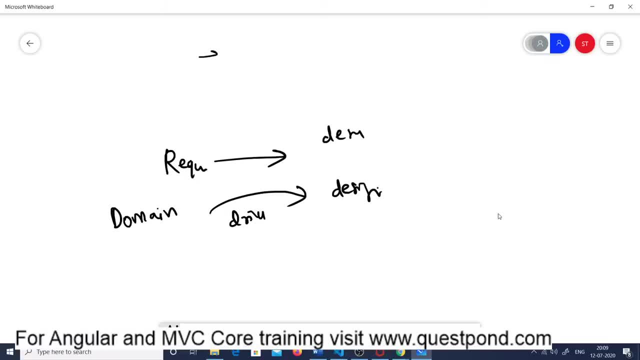 if a customer says that i need to create a project, you know where we have. let's say, a patient has only one problem. let's say, assume in that project the patient has clearly said the hospital or the healthcare company has clearly said you that, hey, like I need to create. 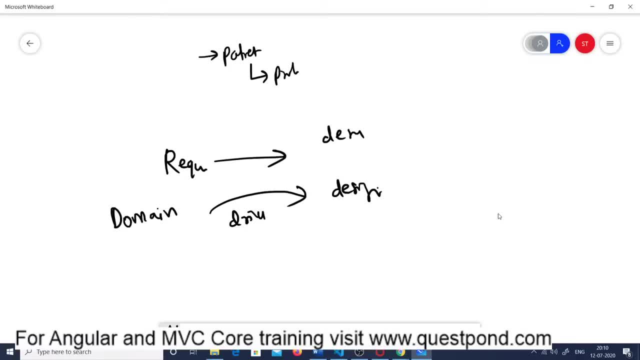 one patient entry screen and in that the patient should, I should, be able to enter only one problem. but then what the architect does is he says: no, like I will be flexible with you, I will go and I will create two tables. I will do one to many the customer did not ask for. 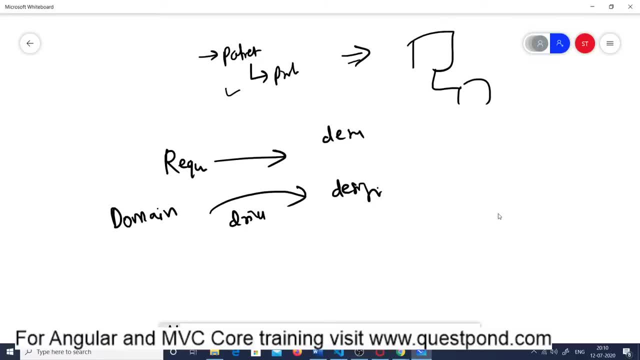 it. but you created this right. you created this because you thought that you know, this is, this is your own thought process, so this is termed as over architecting. you know when and you know, and it's very but natural that we get carried away with it, for example, even. 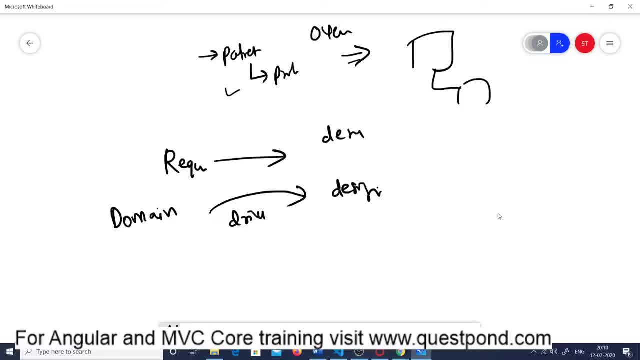 when I was a team lead. right, somebody is to give me a requirement. he never said that this has to be needed, but I just created a logger. I just started logging things. you know, like he never said he want to log things, but I created it, you know, because I felt that you 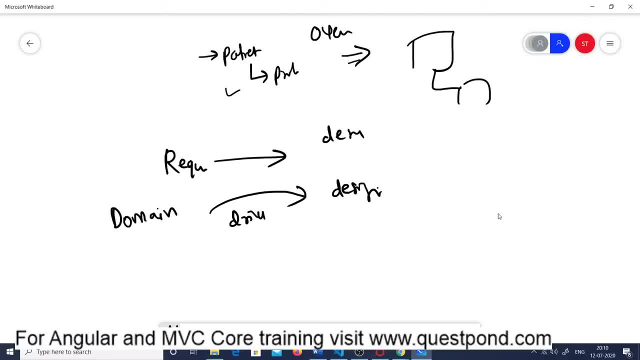 know that's the need of the customer, right. so look at the requirement of the customer and that domain should drive your design. this is termed as the domain driven development, DDD. I feel in an architect the first thing which should really really go inside it is that I am creating applications for my customer. so if my customer says he just needs one address, 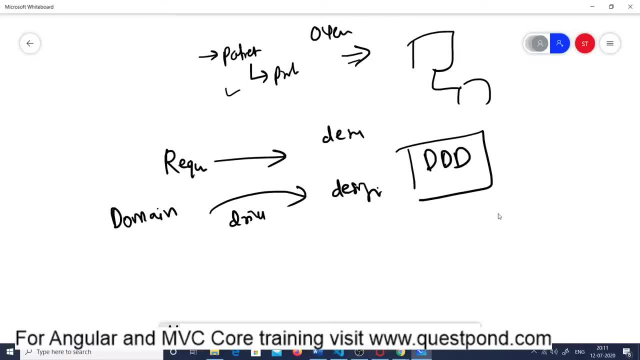 I shouldn't try to create multiple address kind of design right, domain driven development. domain driven development is a thought process you know, wherein Whatever is given in the domain, you just design, as it is nothing less, nothing more. now what happens with that right? so so means, in other words, in a domain, if someone says: 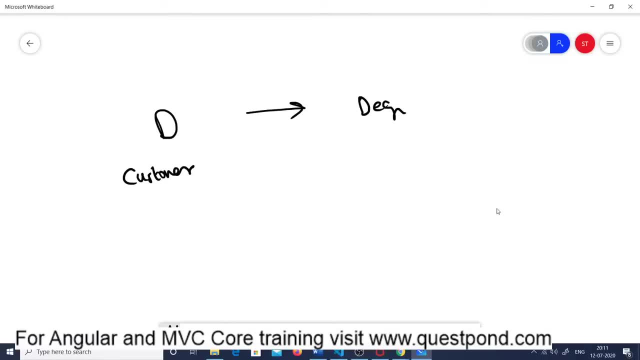 that this name, this is a customer, and customer travels from London, Bombay, London, assume. so if he travels from London, he goes to Bombay. so this is an, let's say, London. back again, this is an itinerary. assume right now, when you start designing out here, you should say: 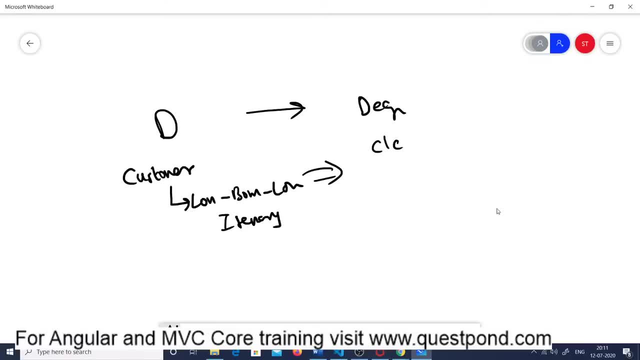 okay, I will go and create exactly like that. so class customer. I have a customer here. I have a class customer out here. he has used the word itinerary. you will suddenly find people changing this word itinerary to path. don't do that. if he has used the word itinerary. 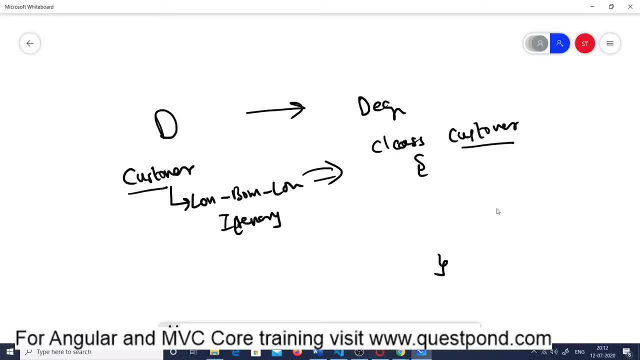 you also use the word itinerary, right. so over here, you know, don't try to like, say okay, like. let me create a class here called as path. Now this is called as not following the ubiquitous language. ubiquitous language, that is the first. what do you say? the first thing in in domain driven development. so I'm just going to go and 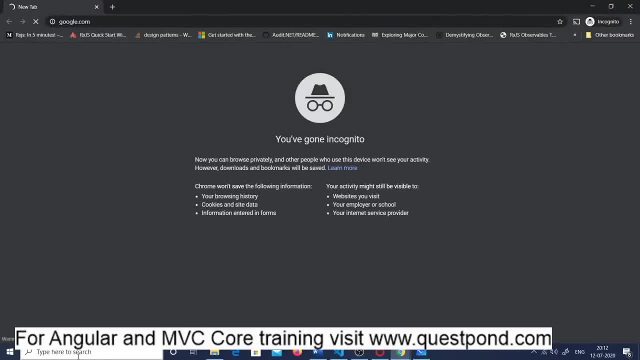 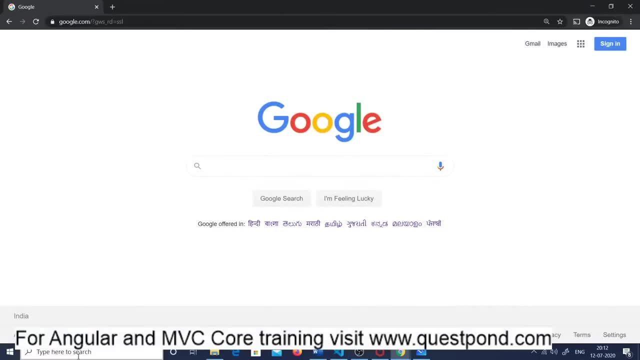 Google out there, you know, so that you can also go and check out. so, domain driven development, which was created by Eric Evans and which is created by Eric Evans, and it's one of the ways of looking at starting your architecture right. so in DDD, you know, we have 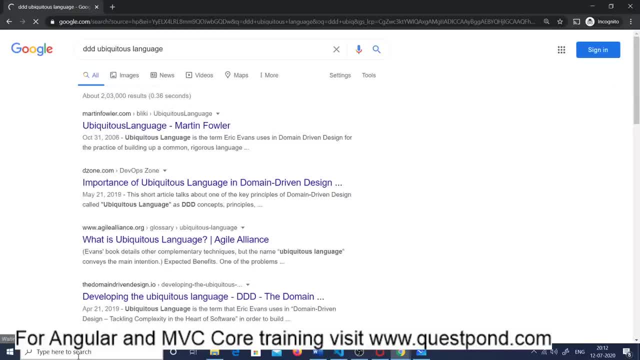 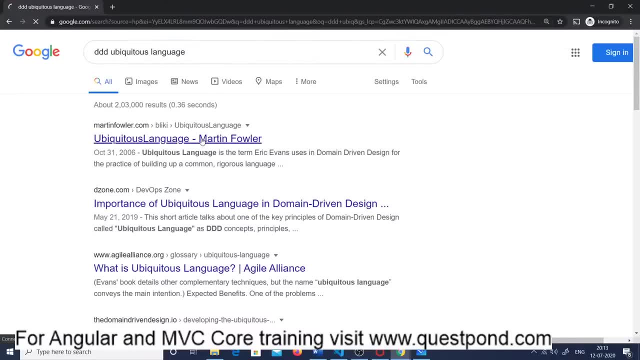 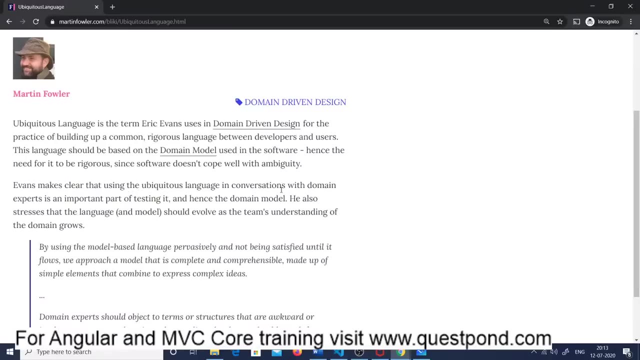 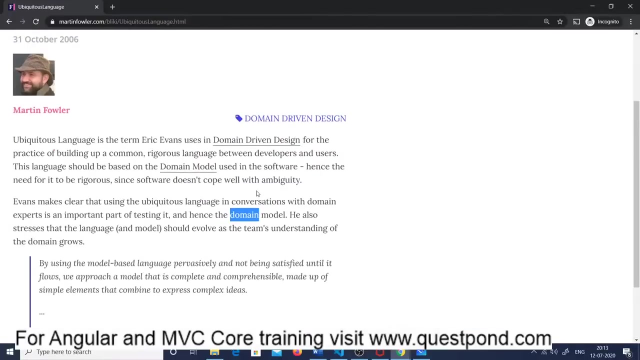 this ubiquitous language. that's it, ubiquitous language. ubiquitous language must be. I can take up any article out there. I can take up the article from Martin. so it's a language wherein in the conversation, whenever you do on conversation, we just follow the domain model as it is right. so must be the small paragraph. you can have a look at it a lot. 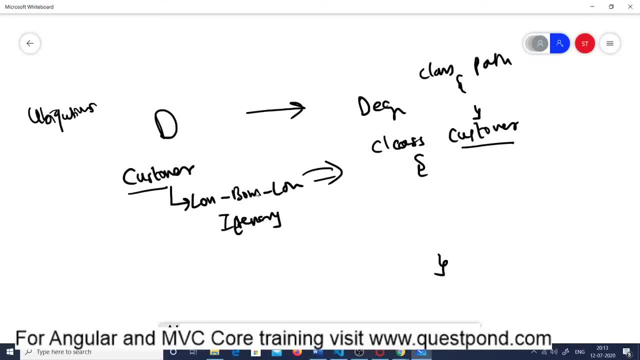 of people would say that, Shiv, I think we are following all this. no, we are not following. I can say that very clearly in in when you sit in a conversation with a customer, I have I've seen people putting their own thought process into it. right point number one follow. 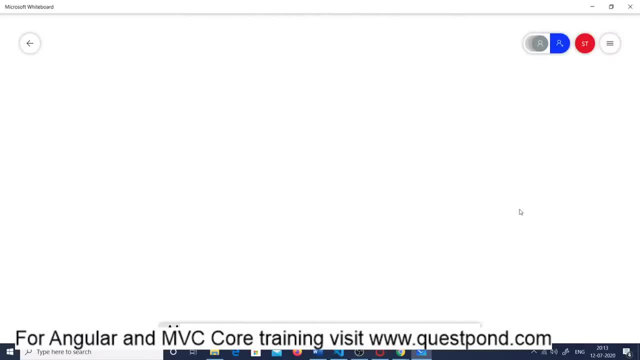 domain driven development. let me start here, slow, slow. I will then go towards source code as well. if you have any questions, you can put down on the chat. right, remember, every Tuesday, one, one hour you have to be with me. I have a very big course out there. fifty design: 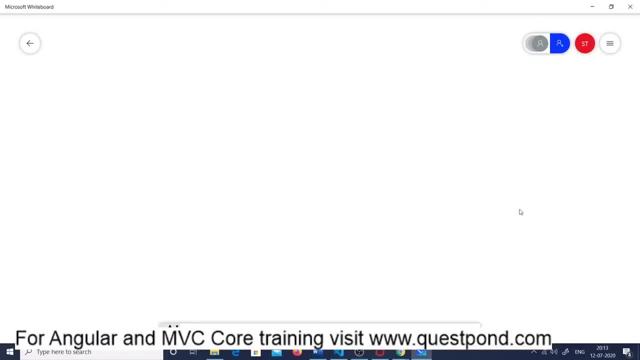 patterns: twenty architecture patterns estimation. so this is a marathon which I'm going to run every Tuesday on questpond right. so first thing in your head it should be DDD. whatever the customer wants, I will give him exactly like that, right if you try to give him something. 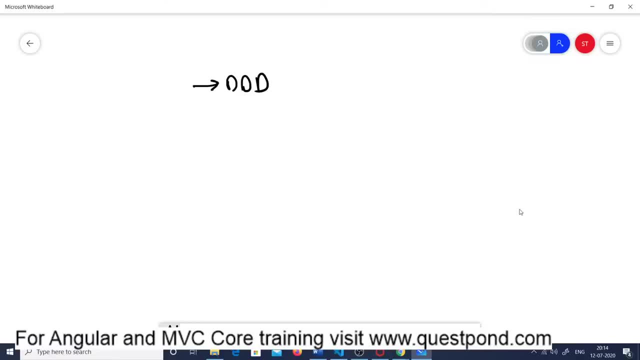 more, your estimation rises, your project goes under loss. if you try to give something less, the other customer will be unhappy. give him exactly what he wants. if I try to do that, if I try to follow my domain, it's very easy. so when my domain changes, my design can also. 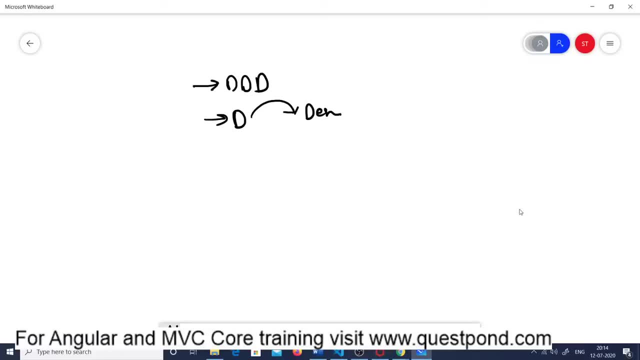 change easily. right, because I am with the domain, right. 2. You can stick to ubiquitous language. let's not introduce our own vocabulary, let us not introduce synonyms. if he has said patient, don't make it TBL, patient, don't make it CLS, patient name: the same class, same thing, exactly like that, right, ubiquitous language, right? so? 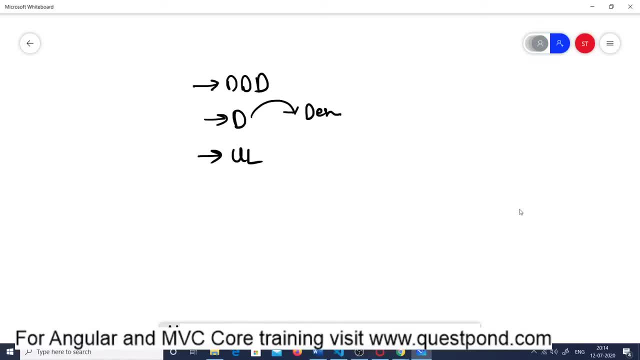 guys any question. this is just a start out here, but I would like to go and see some questions out there. so first I started with just a gist of an architect: that an architect should- a real architect should- be able to do that right, You know, should have multi skill kind of thing right with technology. he should also have 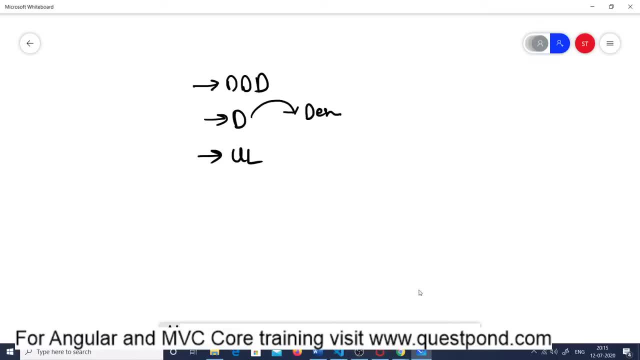 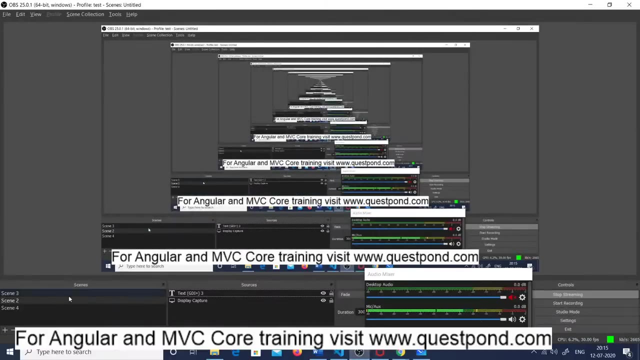 no estimation. he should know this, these things. and then I started with saying that the first thing you should know is that how to connect the design with the requirement, and how it can be done by following domain driven design. follow as it is, follow ubiquitous language, right, let us go back to some questions. if you have any questions, you can put down in. 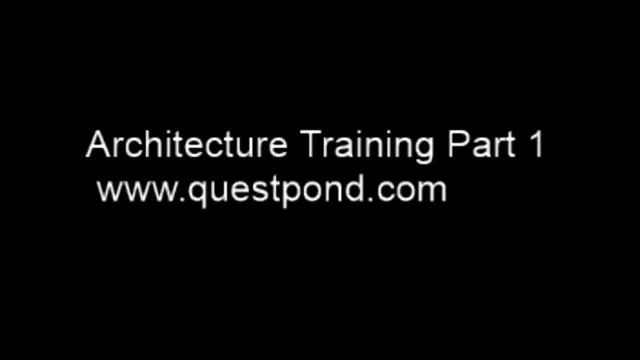 the chat. I am more than happy to answer 3. You know? 4. Very interesting, right? so I can see here Rishikesh has put a very good question out here. customer wants to prepare a pick then start using as a product. right, in this case? 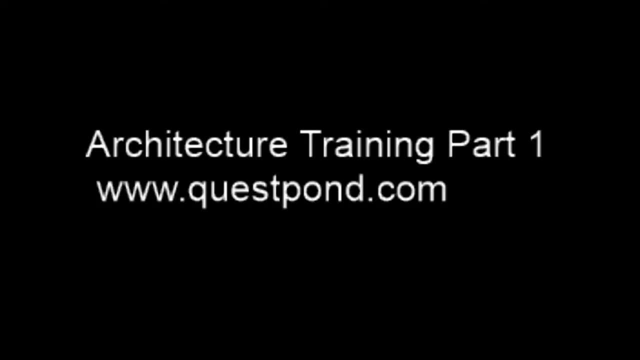 how to architect a pick to a product. so what you are saying is that the customer has given you a UI design and says that he like this UI design. I need to go and, you know, make it as a product. the first thing is, if he gives you a UI design, it is good, that means that. 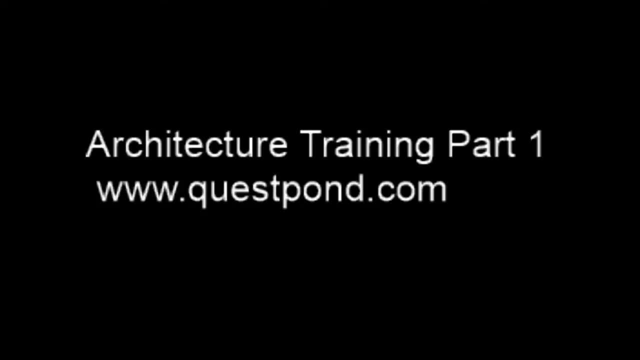 he is trying to be very specific. remember, guys, lot of people you know what. I have seen seniors out there saying that: oh, no, no, no, no, you don't create the ui first. don't go first write the text. no, you don't have to write the text, you. it's okay if he's giving nitty-gritty of. 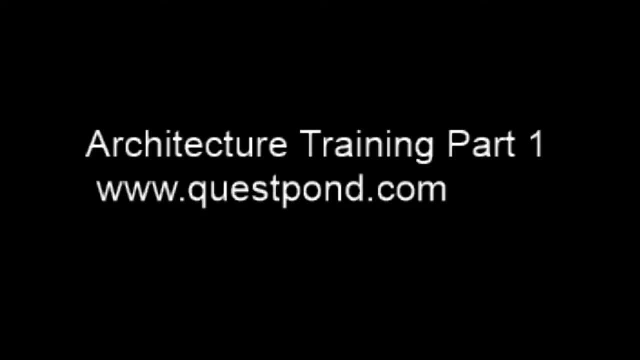 i'm sorry nitty-gritty of of of the looks. if he's giving you screenshots, if he's giving you a prototype, awesome, he's hitting the nail actually right. but the point is that that ui has to be converted into classes, that ui has to be converted into a table design you need to think about should. 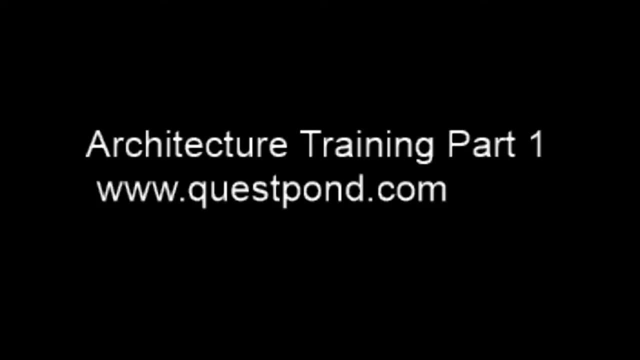 i use azure or not, so lots of things goes in the back end. so i feel so, rishikesh. the first thing is that he has to prepare a basic high level document what kind of classes i will have. and while he's doing it, right use cases must be. he can start first with a basic use case, at least that this ui. 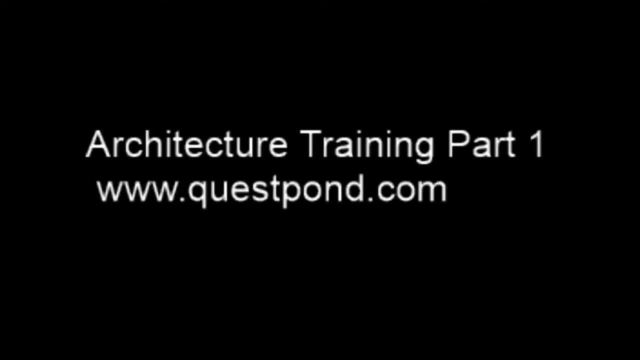 will do what? so some basic text document and then start designing the system? can't we judge customer customer requirements? can't i educate the customer? increase of not so significant requirement? so here's a very good question from mandar. but remember it's a double sword. what mandala is saying is that can't i educate the customer. see, it is good if the customer 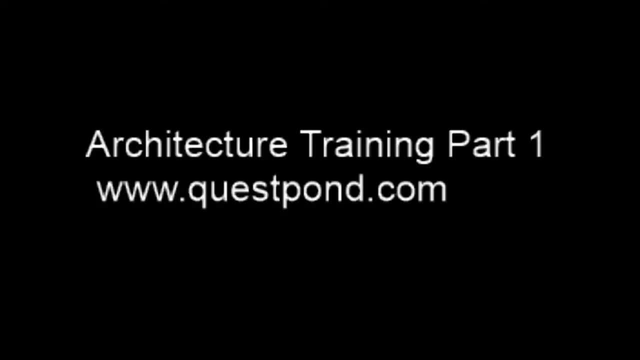 is is understanding. it is good, but remember that when we customer knows his, his domain very well, until you are also a part of the domain he knows, like, for example, if a person is into health care, he knows that what is a patient, you know what are the diagnosis, we can tell him that, okay, this is. 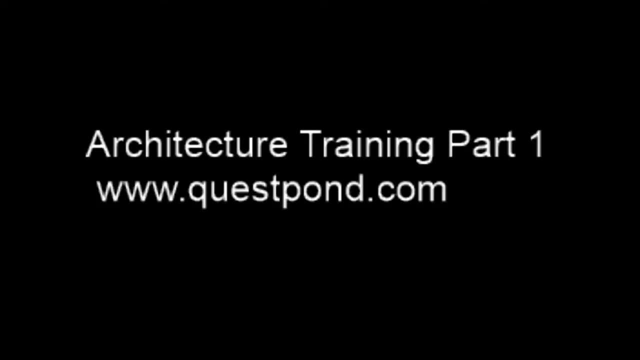 the way to do it, but the the requirement should actually come from him. what exactly he wants, right? the design is the other part and whenever the requirement comes, you just follow the requirement if you are into the domain, if you also know the domain very well. but that takes a bit. 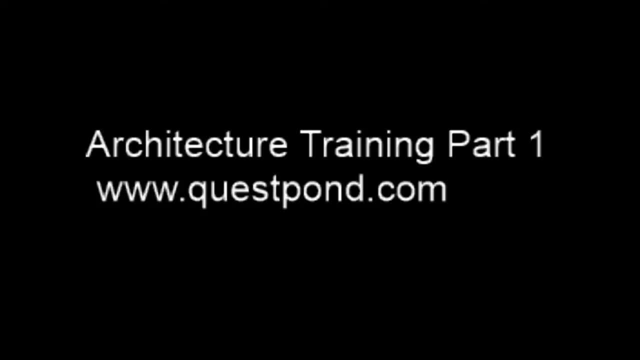 time you have to be with the domain, right then it is a different thing. but i would suggest, um, if it is an internal project, i'm going to say let me again classify. i'm so sorry. i'm trying to uh talk something more out here. what i have seen is that the architect role changes, you know, with the type. 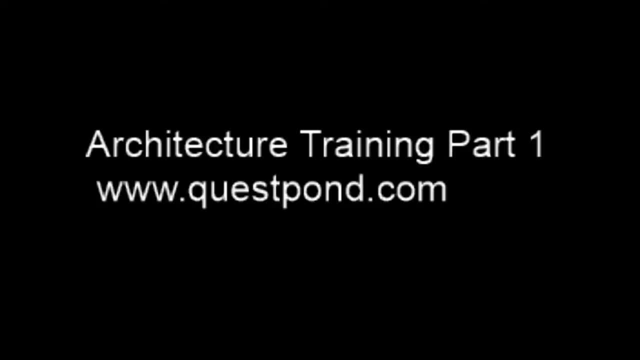 of company. for example, if you are working in a it company where the person who is at the client, who end your IT company, it's like a pure IT based software, at that time you know, educating the customer. I won't suggest that. but if you are working in house, where you are working in hand, 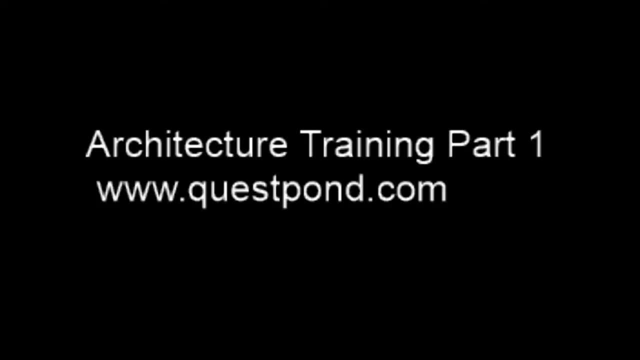 to hand with the customer where you don't have any kind of legal document signed. you know it's all like debit and credit, so you know it's just cost accounting about the project. yes, in those cases, in non-IT companies, you know where the customer and the developer are sitting together. 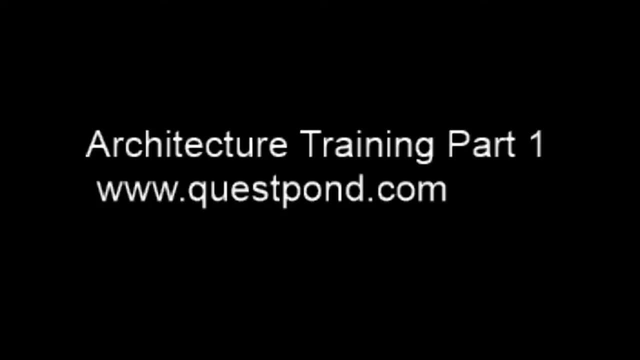 it's a great place. you know where the developer can give suggestions. you have the IT, because the IT works for the, you know for the non-IT out there, right? so I think it's a different scenario out there. what's the difference between an enterprise architect? okay, let's look at it. proof of concept. 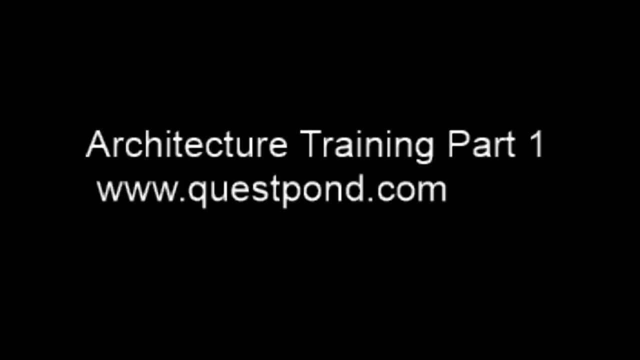 of product right. what is the actual name of Ubiquitous language, if not TBL? patient, so Jalaj? what I mean to say is that if somebody said that this is a patient, why we should use the word TBL? that's the actual name of Ubiquitous language. if not TBL patient, so Jalaj. what I mean to say is: 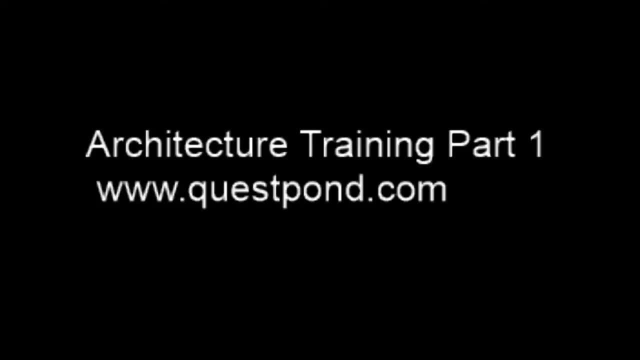 that's the only question I'm saying why we should say CLS patient, just keep it patient. if you look at today's entity framework, core and code first, they are going the same route. they are saying that this is our class and this exactly should be the table. so gone are those days. you know where? 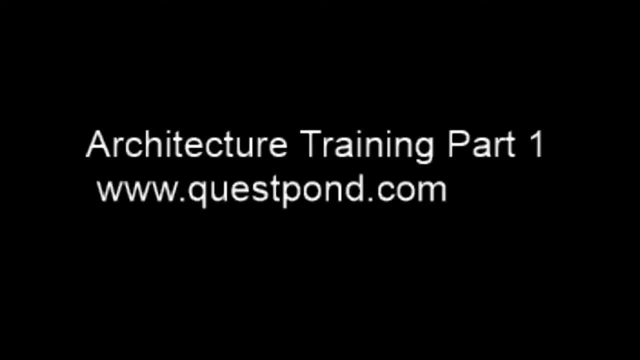 I say that I have to have TBL underscore and SP underscore. right? there were different reasons of creating SP underscore. remember SP underscore, where people is to create those naming convention. there were different reason for it. those reasons actually don't exist today, right? so give a thought. 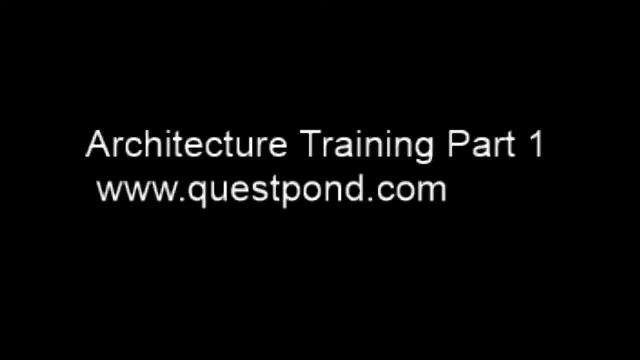 on this again. as I'm saying that why we should have TBL underscore and why we should have TBL underscore where people is to create those naming convention, there were different reasons for it: those we should have TBL underscore and why we should have TBL underscore where people is to create those. 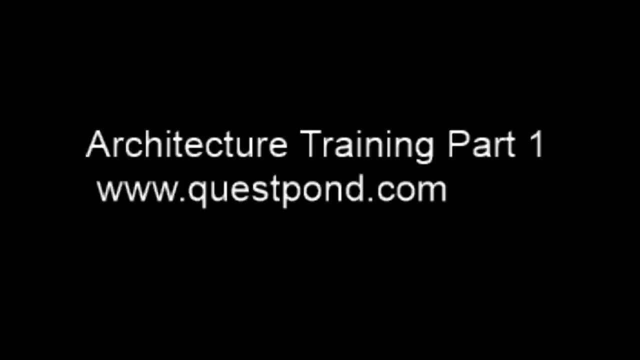 because if we have TBL in our company, the payment director is going to have a lot of work. we should have TBL underscore. we should have TBL underscore. and why do we work with TBL's? I mean, what I think, as an architect, must be: depending on your working condition. it probably won't be the won't be the. 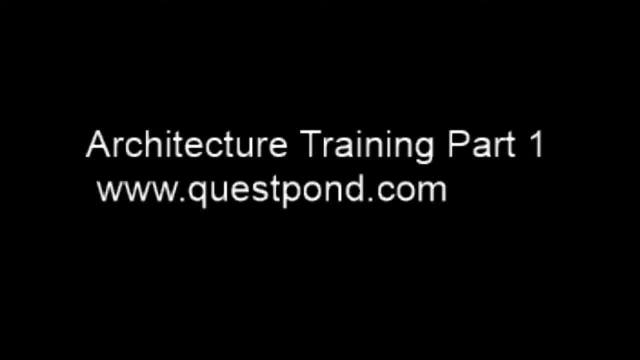 zap fit right, but I feel that we should go ahead with the requirement acities. okay, let me go and look at other questions. I'll come to the enterprise architect, solution architect and infrastructure architect- right, so we'll have a different session on this, you know. so how much relation should. 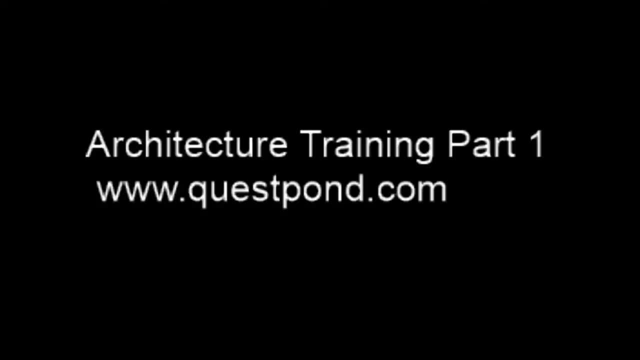 maintain between the model class, view model class and details. okay, so I can see a lot of things out here. let me answer one question. this is a tough one, okay, I've seen a lot of questions about this. let me answer one question here. is there any tool for estimation from shubhashankar sarkar? so here. 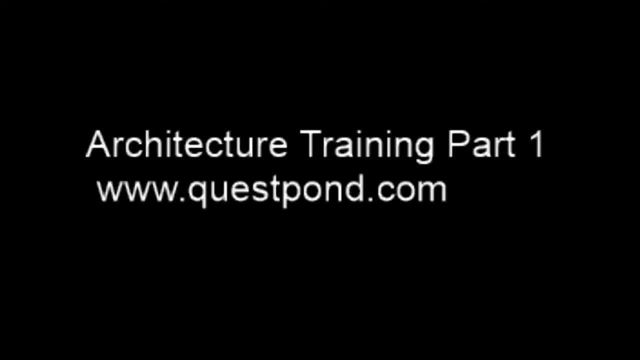 it is shubhashankar. i feel that whatever companies i have worked as an architect, any tool does not work, actually excel sheet. that's why i've seen in a lot of companies you know there is a qa. the qa creates a nice excel sheet. he puts his own mandates, all his costing. so i would suggest 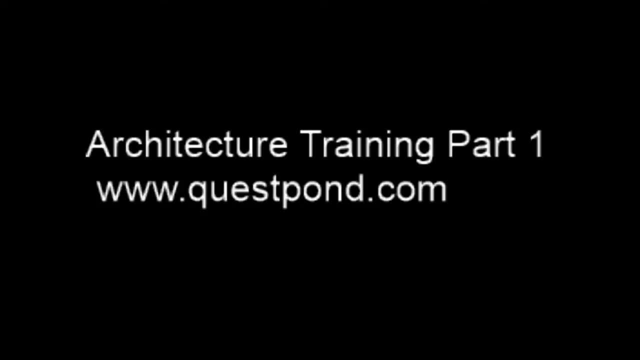 for estimation. create one excel sheet. you can check your things properly, you can put down your notes, right. so i know that there are a lot of tools out there, but i find that those tools you know become more of a hurdle, you know, rather than helping out. so use a function point excel sheet. 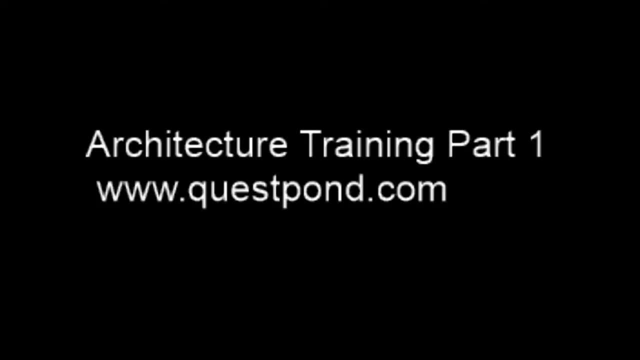 if you want, use a wbs excel sheet and do estimation, right, uh, so, uh, okay, yes, right, so okay, i can see jalaj, i'll come back to that. so first thing, jalaj, let me, when i say that this patient, right, i'm talking more at the class level, at the model level, to be very strict. 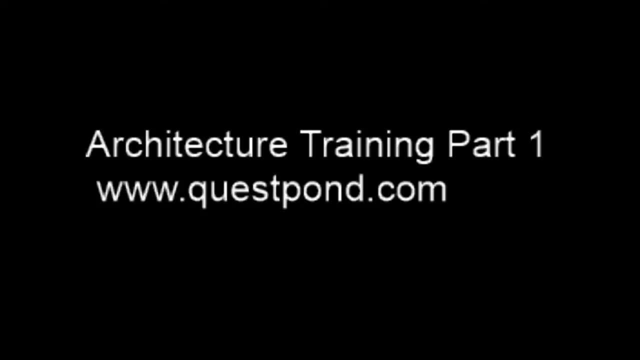 so in the class level i won't. i don't want to give it like cls patient or you know patient underscore something. if you feel you know from the rdbms level you need to have tbl, it is okay. but nowadays when i look at sql server i can create folders, i can. 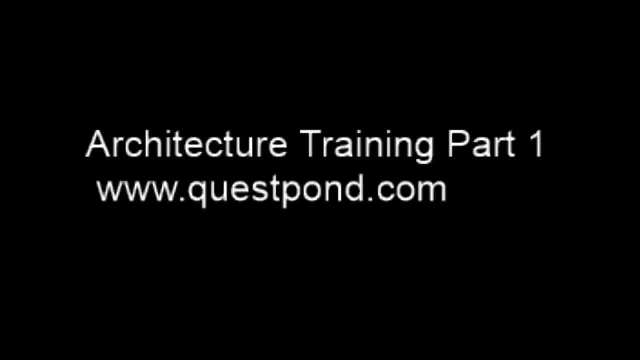 group them into folders and all those things are available, right, okay, all right, fine. so there is a question from basant kumar, questpond support. please help basant kumar. he is asking. basant kumar, you can send a mail if you're not going to reply. 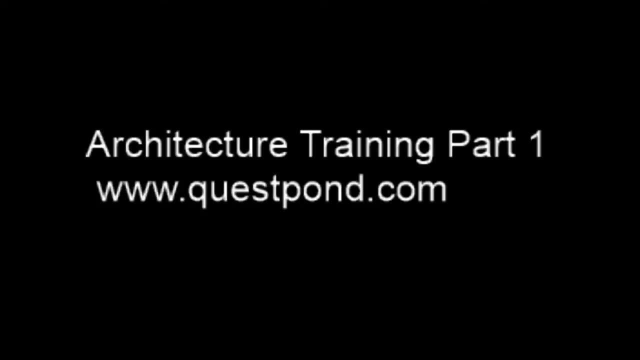 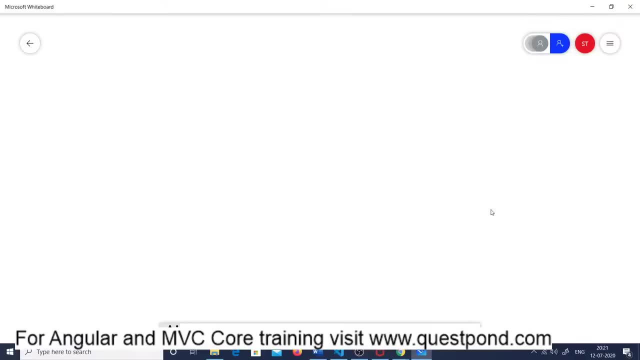 they will reply it out here. okay, let me go back out here, uh, and let me again go back to our things. you know, so, okay, so now you thought about domain driven design, right? the first thing is, uh, domain driven design says that when you start designing your classes, right, so assume that. 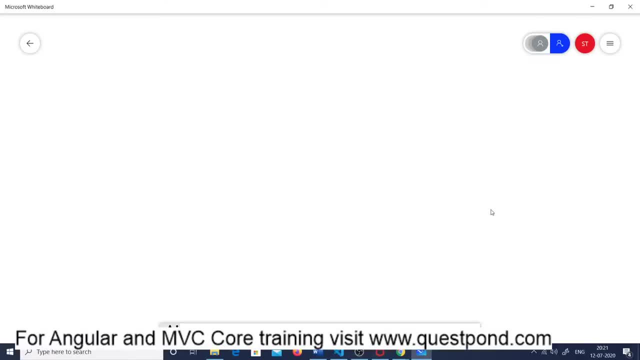 you have got the requirement and you want to go and start designing your classes, right? so, uh, you have some requirement out there and for that you have to go and start designing your classes from there. you will actually design your classes now. you will see that as a natural thought process. 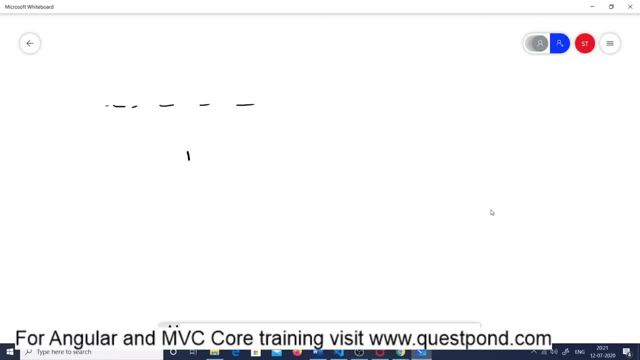 you know, what developers do is that whenever they create a class, it is actually a noun. so, for example, if someone says like i want to go and create an application which is a customer application, the customer application will have an address. so customer becomes some class, the address becomes some class, right and so on. so we normally see that you know it's, it's not that. 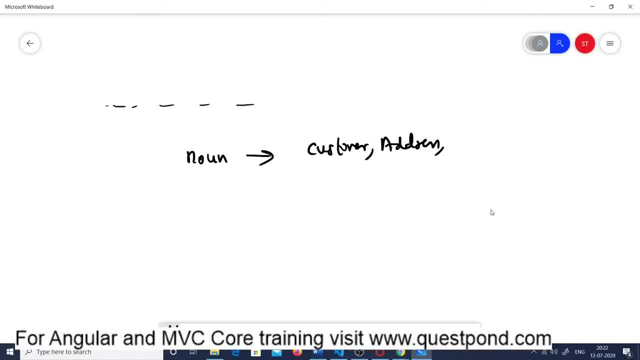 the architect does it very explicitly, but in general, at the back end, you do not see that you end. he knows that these, these can become classes, right. so from the nouns you know, some things are classes, you know. so now these type of classes, which comes from the noun, are termed. 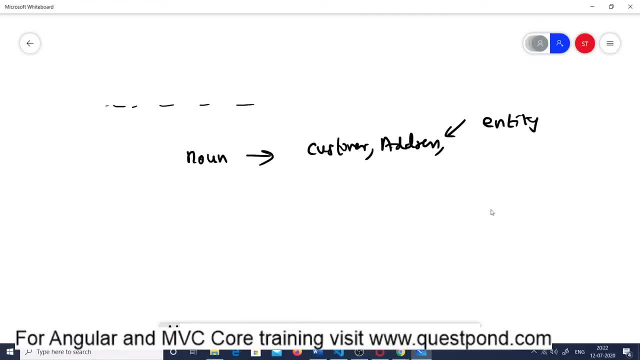 as entity classes. entity classes means one in entity classes, in entity objects. these are actually domain objects. these are something in the real world out there. you see a real world customer, you have an address, you have, you know taxes, so these kind of things you know actually become an entity. an entity means something that is existing in the real world. 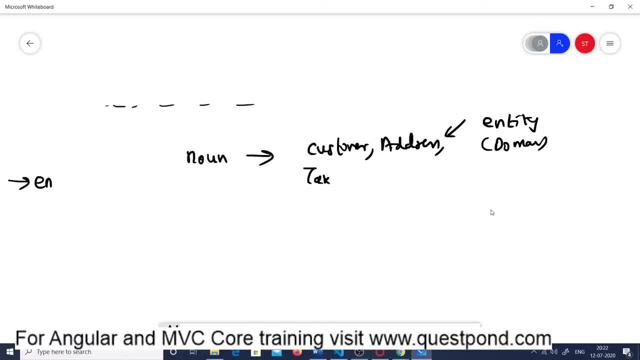 out there, right? so first kind of class which you will see as an architect is an entity class. remember, this has to go just in your back of your mind, because what developers think is that everything is class- okay, class utility, class, data access layer and class customer. but they have a difference and if you don't understand that difference, 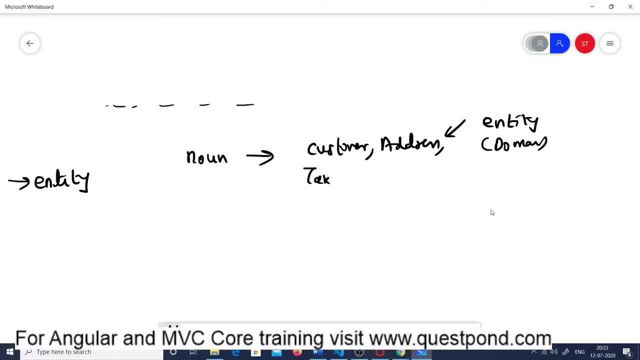 well then you have a class. and if you don't understand that difference, well then you right, layering will be a problem. so, for example, if somebody thinks utility is a class and a customer is a class and currency is a class, but all of these three classes, they really 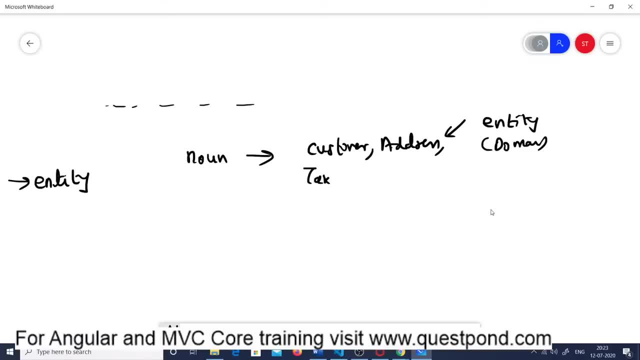 lie into different, different buckets, right, so let us try to identify. so one is this. second, you have classes you know which are more technical classes. technical classes like utility data access layers must be, validation can be possible- or http- you have made something right- so logger classes. you know these classes. 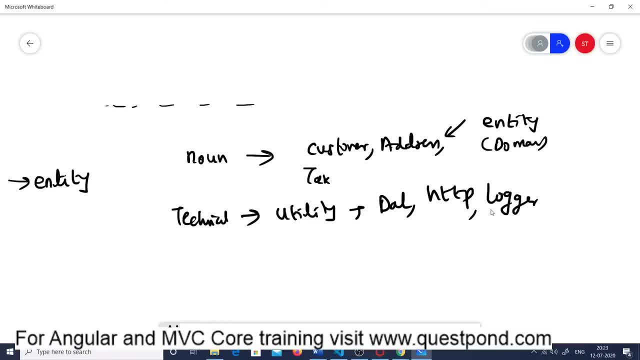 they can be used by everyone. so in other words, if you have an, let's say if you have a customer class and an address class, so the logger can be used in the customer class, probably to log. it can be used somewhere else. the http can use address. so this utility, this, this. 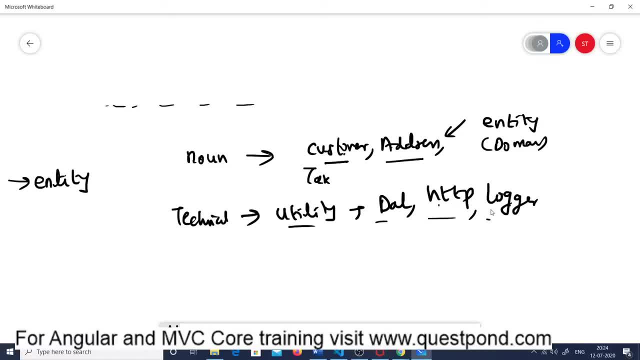 layer out here. this technical layer out here you can think about it is how do you say it? it is used across the layers. right, it is used across the layers. so these kind of classes are termed as services service class. remember a lot of people out there, if you know developers. 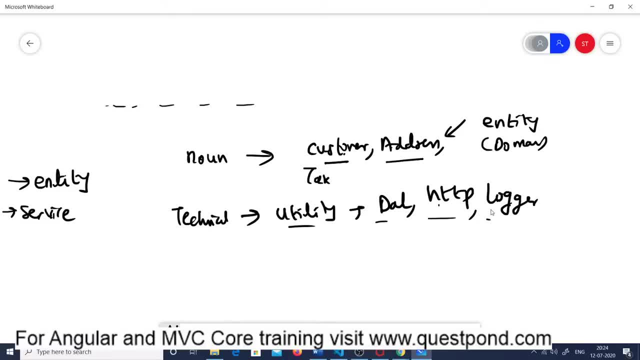 out there. they don't even know the categorization of the classes. so what happens is, when they create the layers, they mix everything together, right? so remember entity classes, which represents your real world. service classes. you know which represents your technical component, right component. you know which is the technical part of it and i'll tell you why this differentiation. 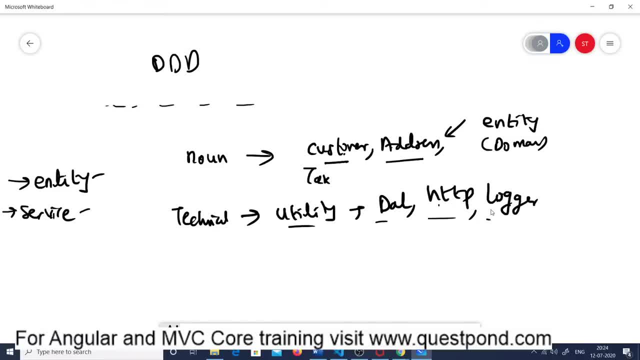 is made. remember, now also, i'm talking about domain driven development. this thought process at this moment, which i'm talking out here, is domain driven design, right, the next thing? so entity and then a service. now there are some other classes- with all respect to eric, you know, i'm not a fan of these classes, you know- but they exist actually and those are. 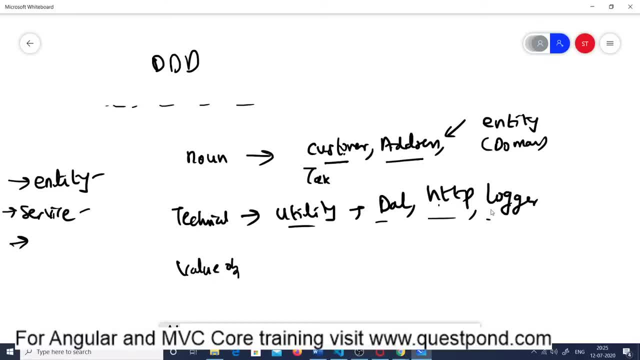 so one is a domain, another one is the value, objects. right again, i'm telling you, you know, i am a human. so as an architect, i have my own likings and i have my own dislikes, i have my own best practices, which i have created, and with those, 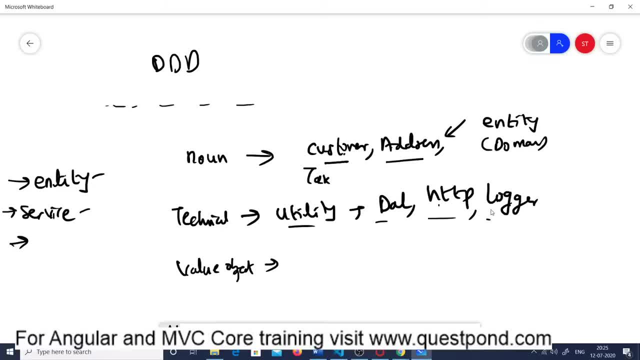 best practices. i had my own success and my failure right. so what i find about this value object is that i have used it very less and my my thought process about a value object is that it is too complex to create right. but what is a value object and value object? 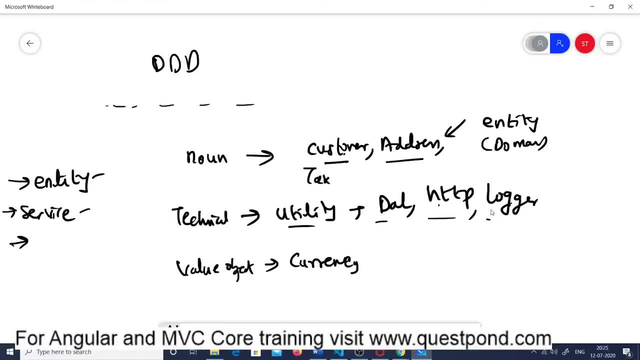 is like currency, like date, for example. you want to compare two dates, right. so when you are comparing two dates, this 12 12 2010 is equal to december 12 2010. now, if you see here the comparison is on the base of value. definitely this. if 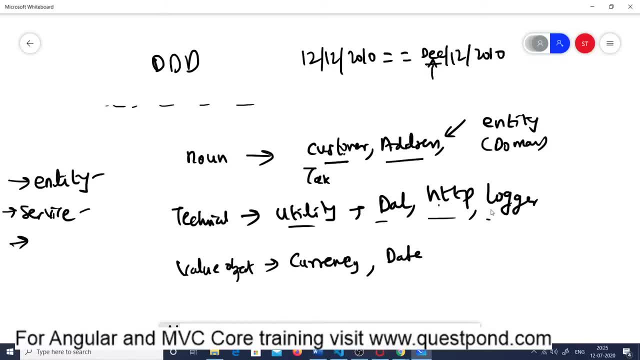 i try to go and compare it string wise. it will not right, but this december is equal to this 12. if i say mmddyy right, one dollar is equal to 70 rupees. i don't know what it is, but like whatever, it is right. 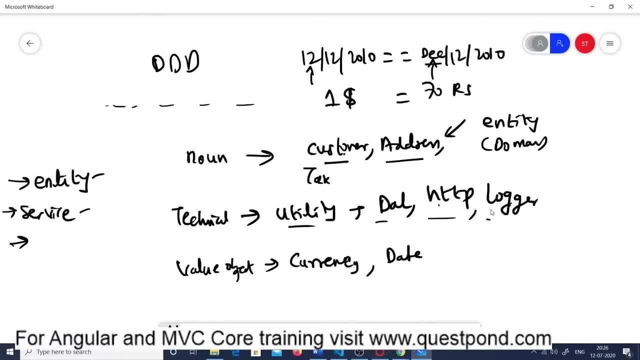 now, here they are checking on the base of value. there is no human out there, it is no customer, it is no address, but it is value objects, right? so again, like there are value object which are compared on the base of value, right so value objects. and again i have said 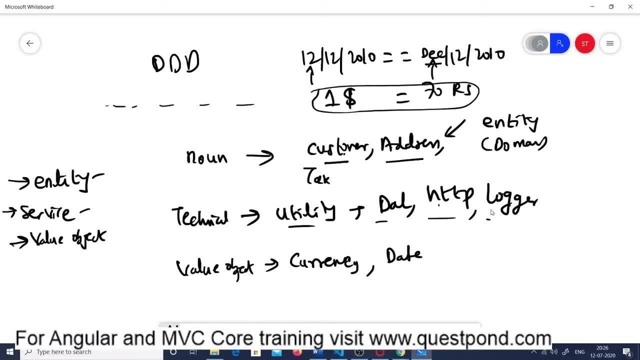 that these kind of objects are difficult to create. you need a different kind of maturity all together probably for these kind of things. but entity and services at least you should be able to classify right. so there are three kinds of classes at type of classes. so when you go and start designing your system somewhere in your back, 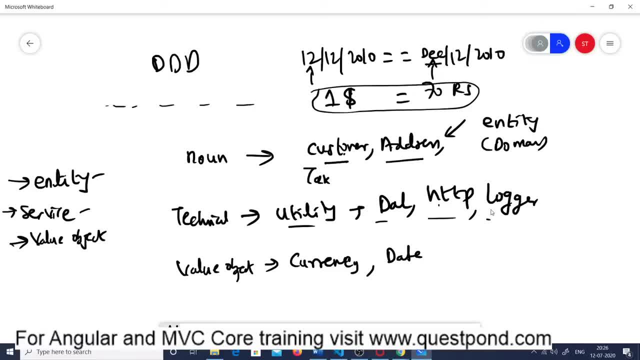 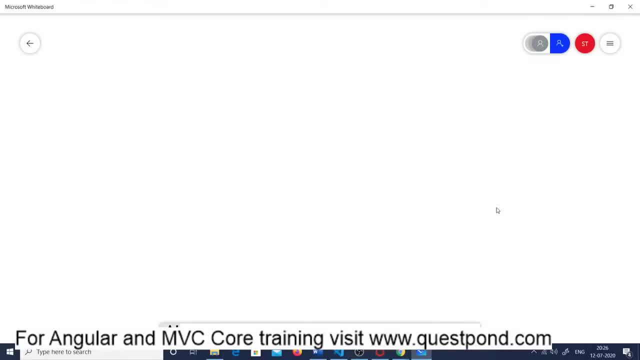 head. you should have like entity class, is this a service class? is this a value object, right? so that means, as someone was asking out here: hey, like what is the onion architecture? i saw that message out there, right? so in this domain driven design, the onion architecture is a byproduct of domain driven design. i feel that really this ddd, which is which has the 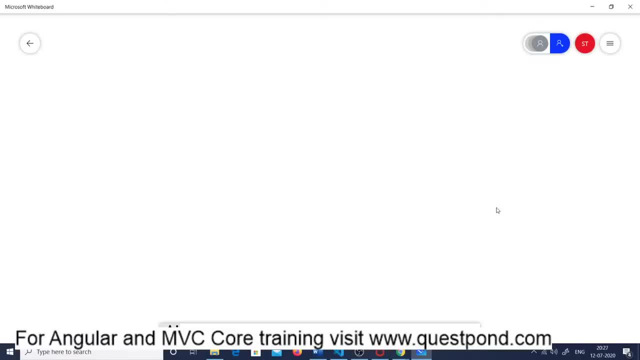 thought process which is by eric. it's a very simple thought process, but i feel that it it, it. it brings in a lot of things together. it strings in the old design pattern of gang of four. it brings in things like repository pattern. it also spawns up, you know, like onion. 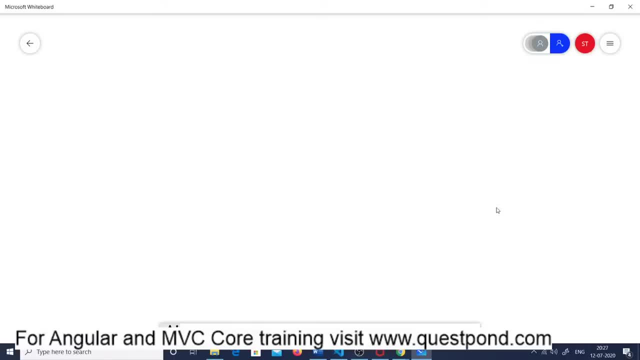 architecture and other things. so i've, i've, i've found that when you start working in a ddd way- right, when i say working in a ddd it means your, your internal culture is ddd- then you will suddenly find that automatically you are doing inversion of control automatically. 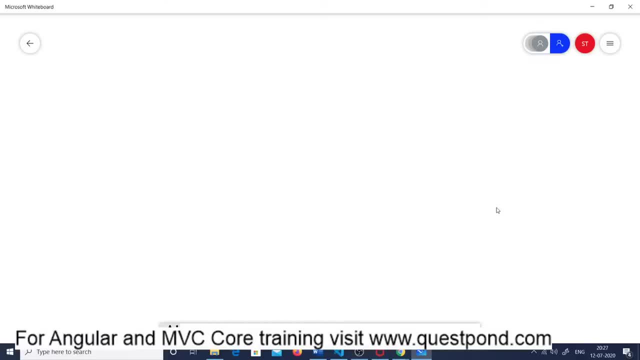 you are doing dependency injection. i'll come to that right. so now, in this domain, driven development. so you have as the b as the thing and you know that this entity logic never changes. so, for example, if you say there is a travel domain out there and if you say london, bombay, london, london, 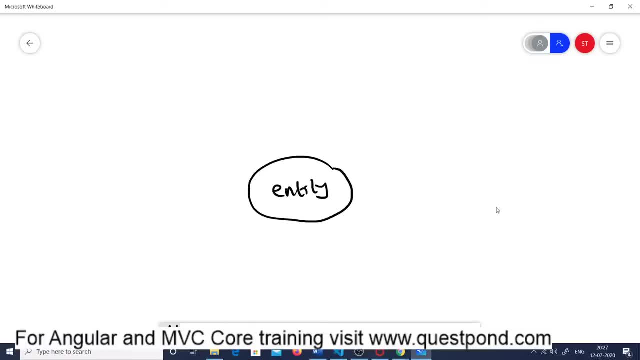 was always london, bombay was always bombay. when you are saying airline, that was always seats, there were already all, always passengers. it is doing it is there for so many years and it is the same like this. there is a bank, the bank has checks, checks as deposit. it has. 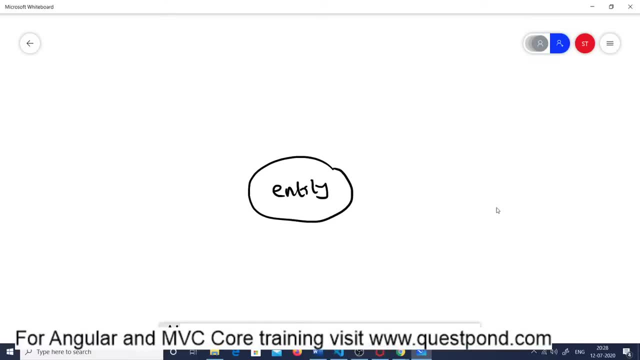 credit all same. you have patient, patient has diagnosed. if you look at it in a general way, the business as such has not changed. definitely they have changed in terms of technology, but the internal, the way the business functions is, does not change right. but what i changed is technology. so, for example, i can have a bank application. let's talk about it. so let's. 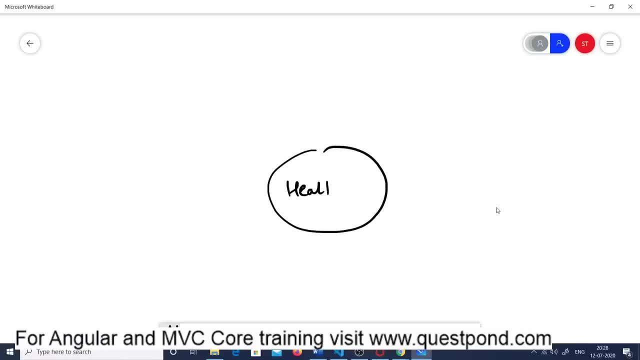 say, we have a bank application or, let us say, an healthcare application out here, the healthcare domain is here, the domain has not changed, but the technology has changed right, and what was happening is we were creating this domain out here- healthcare domain, or the domain objects of healthcare, and we were trying to use the technical objects, for example. i was trying 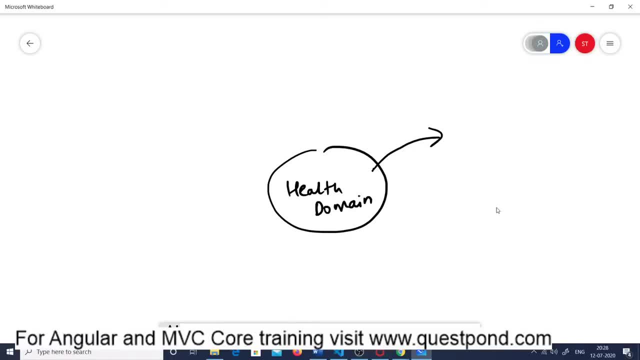 probably here. let us say this: in this healthcare domain, i have created patient objects, i have created doctor, i have created medications, i have created problems, i have created diagnosis right. these are all the classes i have identified. these classes were using classes like service classes. remember, these are entity classes, so service classes means data access layer. 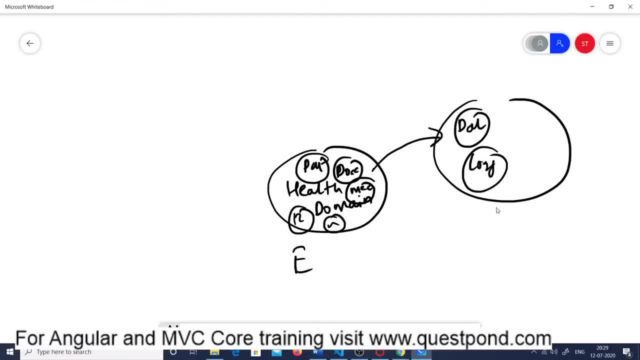 patient was calling the data access layer and we were trying to use the technical objects as a logger utility. if there is a error now, what happens because of this? when these guys change this is technical component, service classes. these are services. these things change like hell. today, data access layer is atonet. they become link you and then they become. 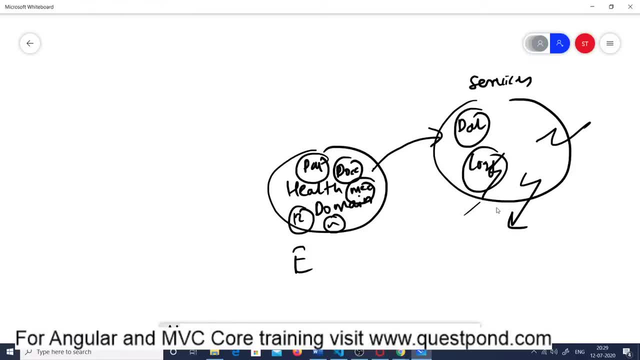 entity framework core, and then they become something else. what will you do? right, you have logger you, somebody likes log4net and somebody likes something else. right now, what happens when this change? he also changes because he is dependent on it, on him. you can see the arrow? this arrow says that he is dependent on him and because of this. 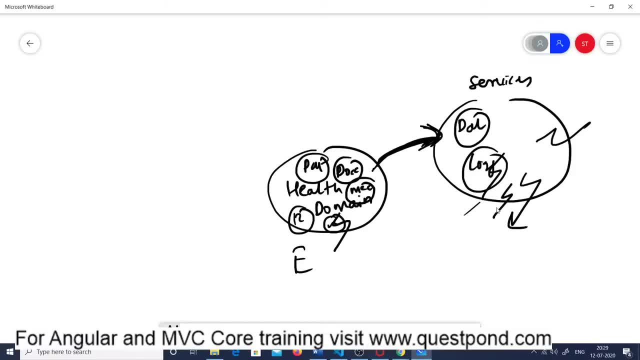 this problem is happening if i invert it, if i invert it, if i say no, like these guys will call him now. that makes lot of sense. it's a very small arrow here and there, like in your life, if you think about if i am dependent on someone and if that arrow changes, like 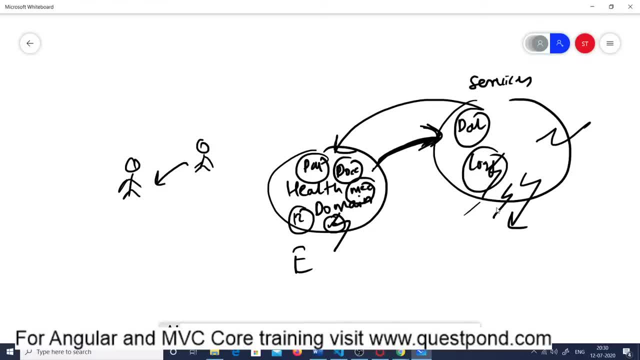 that he is dependent on me. that means that if he changes, nothing will happen to me and i am dependent on him, right? so if this service objects start using the model right or the domain, then any changes which happens here it does not affect him, right? so if you look, 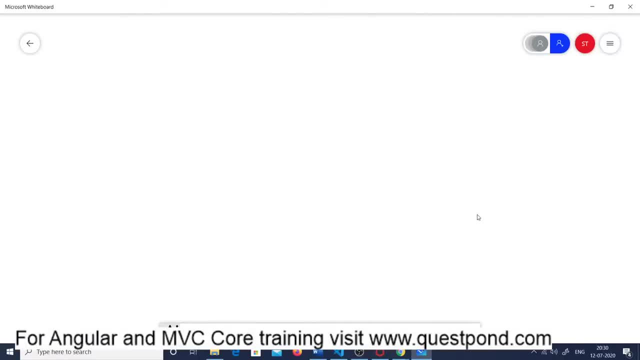 at the domain driven design and that's what this onion architecture thought. remember: all these are just buzzwords. please understand. these are all buzzwords, so don't try to don't try to get too much carried away with it. you know, stay with your coding, stay with your. 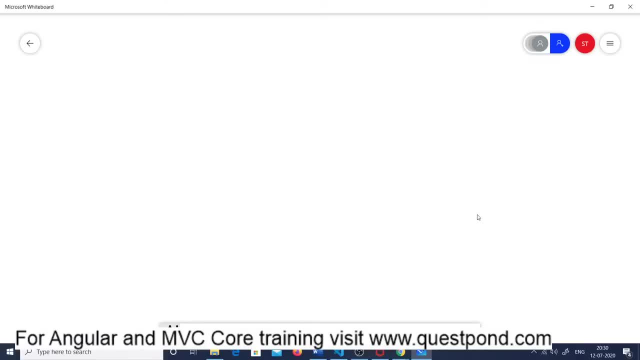 neatness of your code and try to stick to your core principles. so here it is. if you look at the onion architecture, you can see that. if you look at the domain driven design architecture, what it says is that in in between, the first thing, what we are, what we are talking. 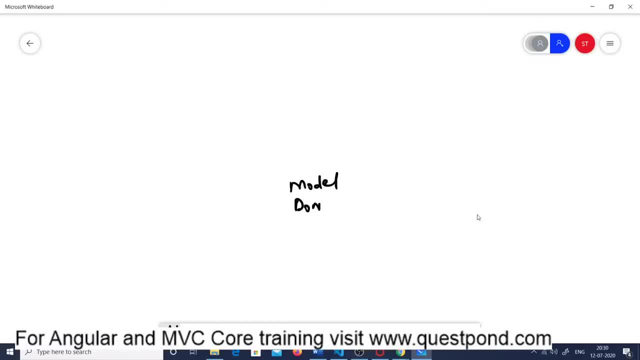 about. here is the model, the domain in the center. this never changed, but around it changed technical. so what did what did change? for example, there can be technology layer, like services people- i know that they create application layer and so on- then ui layers- i don't know. 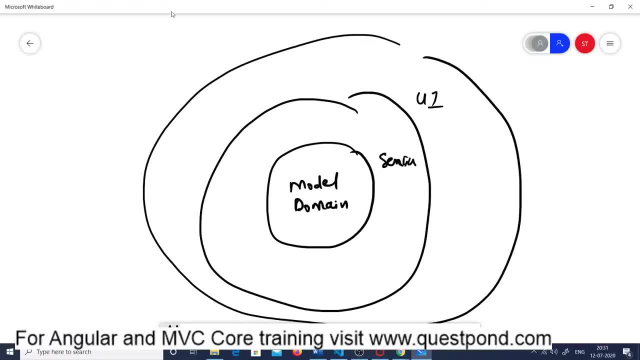 like and something more technical, right? so now, by this onion, what it means is that the service will refer these guys will refer this project. so there is a ui project which will add a reference of model. service project will add a reference of model, but model will never add a reference of it's your. the onion architecture goes in this way: where in everybody. 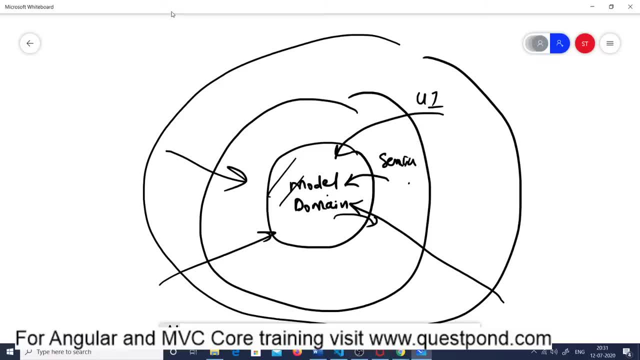 uses the model, but the model does not reference it. anyone right. inversion of control. invert your control in your life also when you have problems. if you say i am dependent on this, so if you try to become self-sustaining, and if you invert the control, saying that no now. i'll do it myself. i don't want you right in that model. i've back again, uh, all large kinds of idea avez i had having at my bros. there are two�ENDER indigenous people, there's a landing and there's no weekend-term. I do any kind of course drivenson, more modern or foreign or 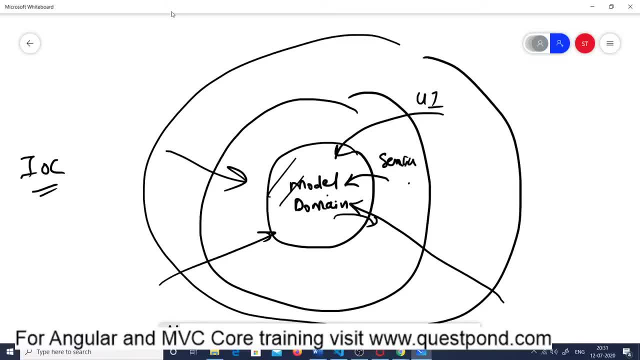 you know when you're just kind of working, you're talking. you know when you're just working, right. in that case you are now independent of him. any changes happens to that person does not affect you. inversion of control: where things were like this, it is now inverted right. all are like. 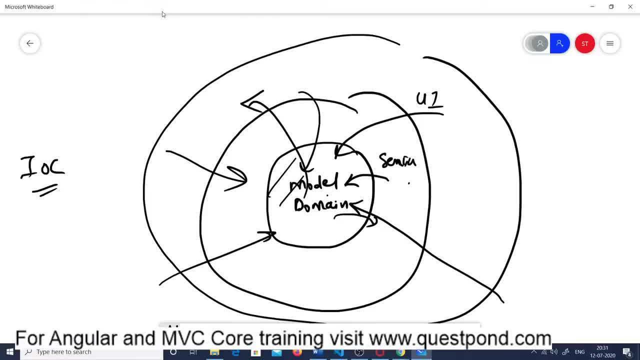 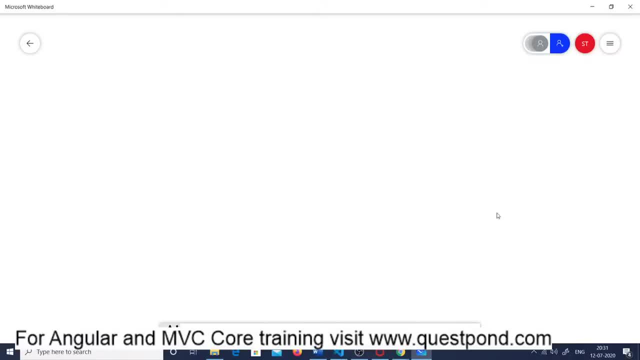 buzzwords out there. so somebody asked about onion architecture. right, so three kind of classes coming back again, just going back to the main screen out there. three kind of classes out there, domain layer entity- i'm sorry, let me use the word of entity- classes you can have, uh, your service classes, i'm sorry, and you have. 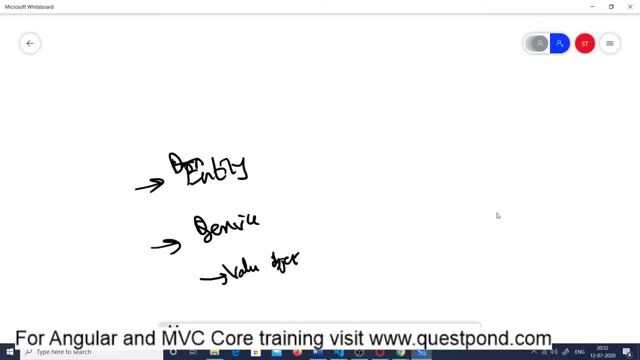 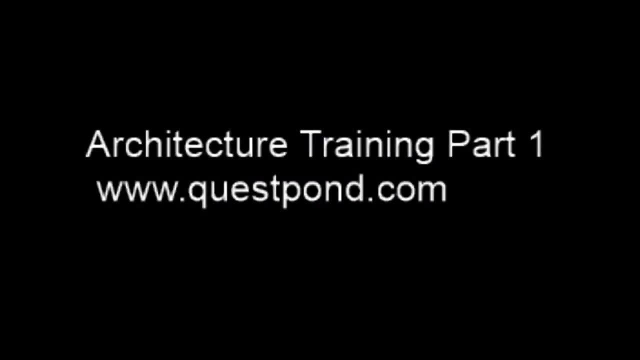 value: object: right, good, so any questions guys on these three kinds of classes, what they are? right, let us first start with this and slow, slow, we will move towards other things. any, if you have any questions, you can put down on the chat. there is a question, uh. 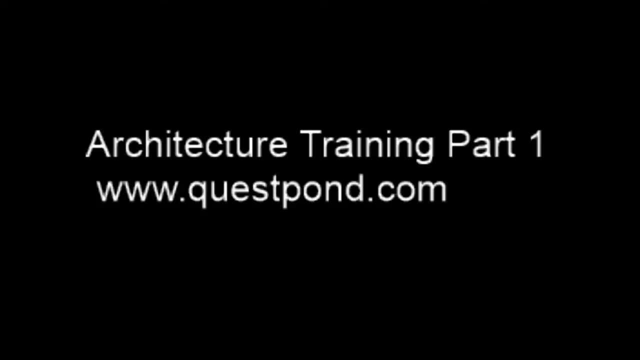 quest font. please take care, you know i can see, oh my god, what the spams are. what do you get by spanning spamming out here? right, it's a technical class. so utility class is a static class and shared class that provide common functionality. yes, absolutely, person. 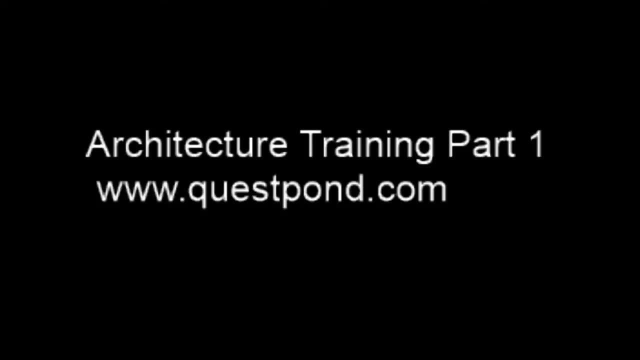 it's a it's a static class. you can, if you want, you can create a utility as a static class and because it is shared across project. that's why i said it is on service, like a car service. if, if there is a car service, out that the car service is for everyone, for poor, the rich, or i can understand the 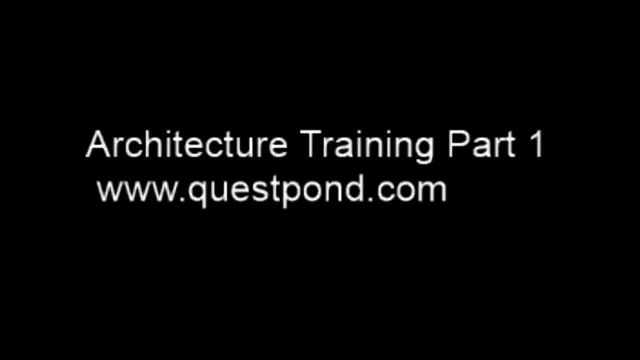 but let's say hotel service. you know it's for the poor, for the rich, everyone out there, right? so we go out there. it's commonplace, right? remember, all these words have come from us, only from our real world. so the way we walk, the way we talk, so the, the software, software. 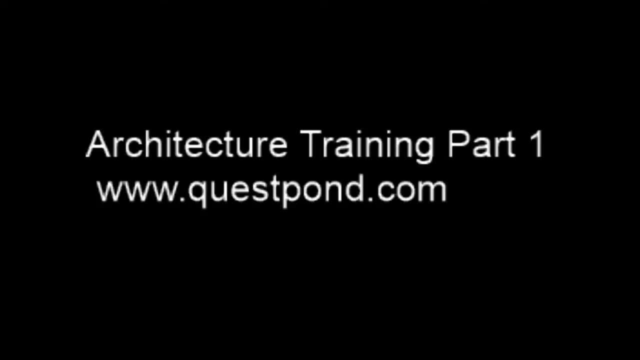 development is not, not nothing coming from space out there, right? so all the words are somewhere connected with the real world. so, absolutely, person. normally, uh, people tend to create the utility class and logger classes as static. uh, rishikesh, we have stored procedures. classes reduces the development time, for you need to make a proof of concept. stored procedure. 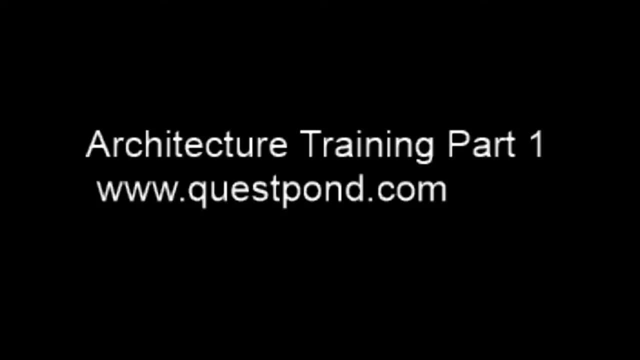 specific classes reduces the development time to get get the less number of man hours. uh, stored procedure specific. i did not get it. rishikesh, if you can tailor the question again. subarji's question here. can you explain inversion of control? uh, see, inversion of control, as i've 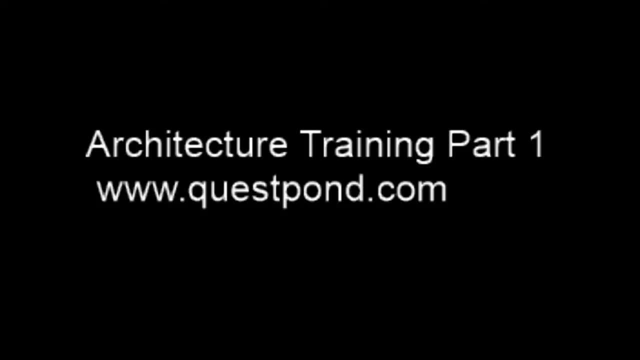 said: subarjit, you know if one class is using another class. okay, i'll just explain in short again. i've already talked it. let's say class one is there, it uses class two. if class two changes, class one also changes. if you invert it, if class two starts using class one, if you have that flexibility, 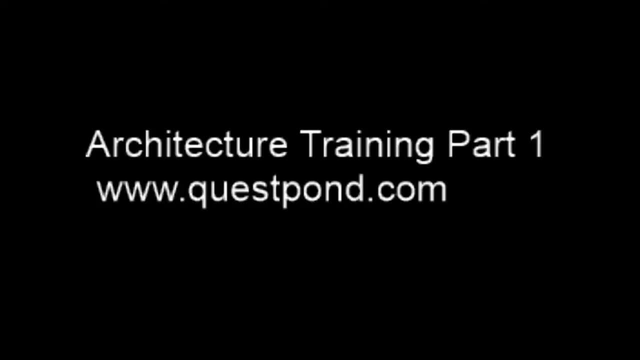 then probably you know your changes can be less right. so inversion of control says that rather than many people depending on one person which is changing, it is that that changing person who is keeping on changing again. he is dependent on others because he is changing right, so better he be dependent on other rather than other people depending on him, that's. 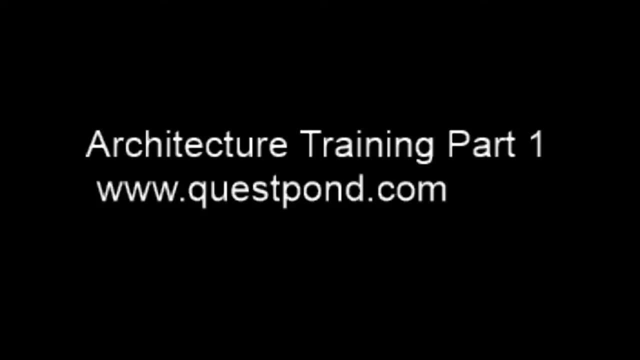 what this is. uh, should, um, okay, each service class can contain configuration. yes, definitely, like. see, remember, all the classes can have configuration, that is not a problem. i'm just saying the type of the class out there is gdd following soi architecture. no, very good question here from. 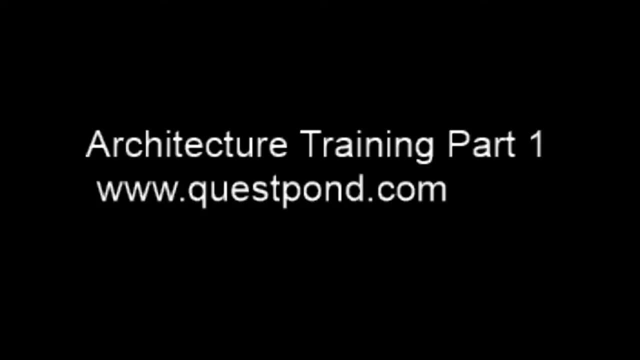 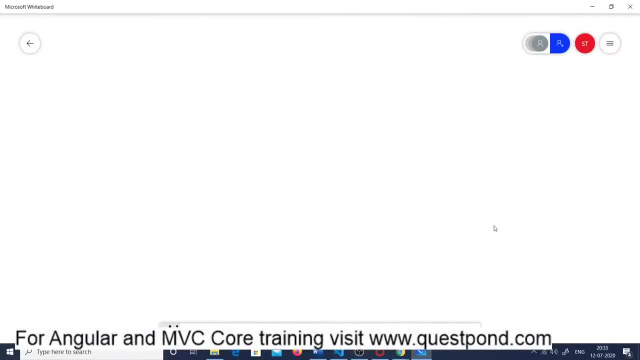 sham pramanik here, that's so let me just talk about this. is gdd following soa, remember, guys? you know, i think i think in every class i talk about this. there are two, three things out here, like: one is you have a design pattern, one is you have an architectural pattern. 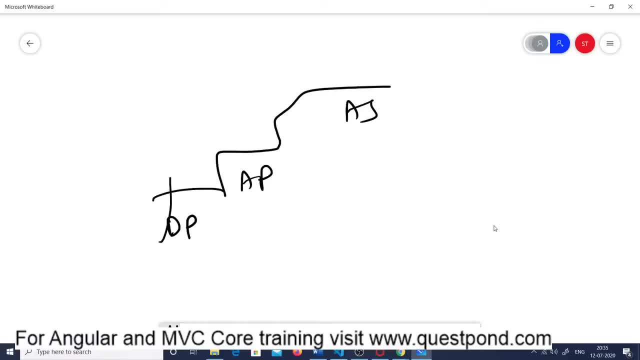 one is: you have an architectural style, please. like you know, in every class i've talked about it. so service oriented is an architecture style, it stands here. rain is an architecture style, it stands here, or whatever you know. so these are architectural styles: architecture, patterncontroller, view and model. 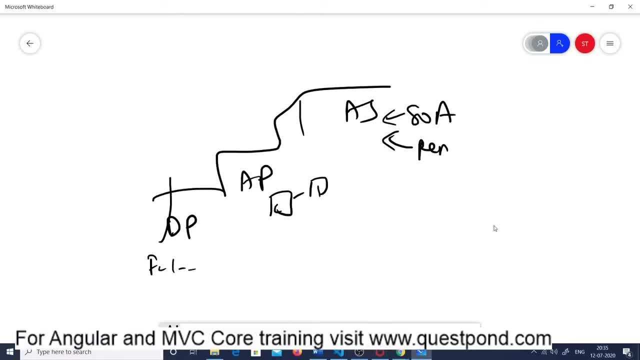 it stands here: design pattern- factory patternsingleton pattern. it stands here: must be down. if you want to comprehensive, go for algorithms. right, i think you know there is a special directing right definition for each one of the category. Now, when I am talking about domain driven development, 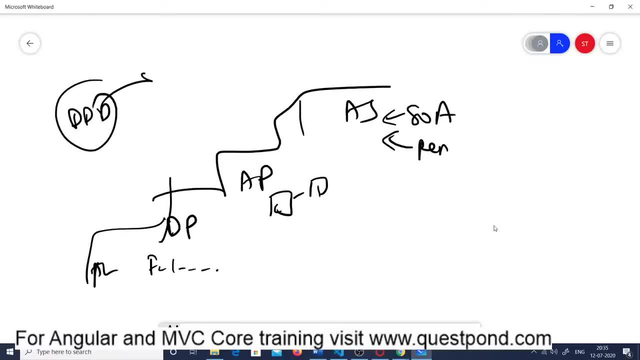 out here. it is an approach. it is from none of these. it is an approach where the human have to think in that way. he has to think in terms of mapping with the real world. it has nothing to do with directly with what you call definitely. the output is a software. 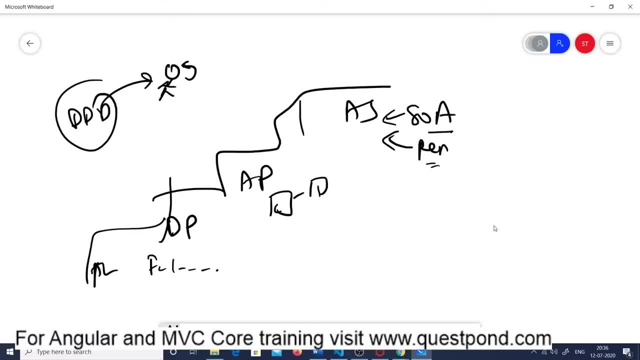 but it is not running with SOA. This service oriented architecture is an architecture style. architecture style means what it is, just a principle. for example, REST is a architecture style which says: follow HTTP protocol. service oriented is an architecture style which says: you know, between two systems you will communicate using XML or some kind of common messaging. 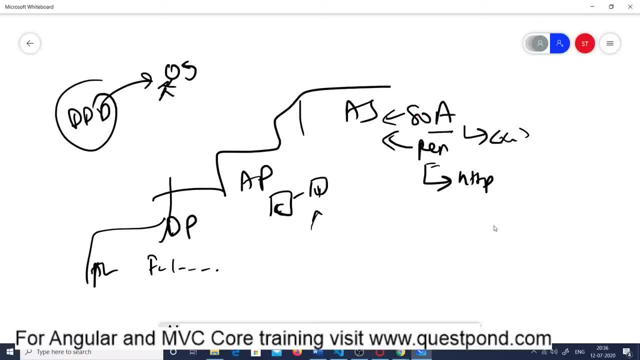 then you have architecture pattern. where is a controller view and model? let us divide a project into controller views and model view will have the UI model, will have the business logic controller will tie up them together. right design pattern here. where here you have actual code. so if you say you want to create a singleton pattern, you will say: 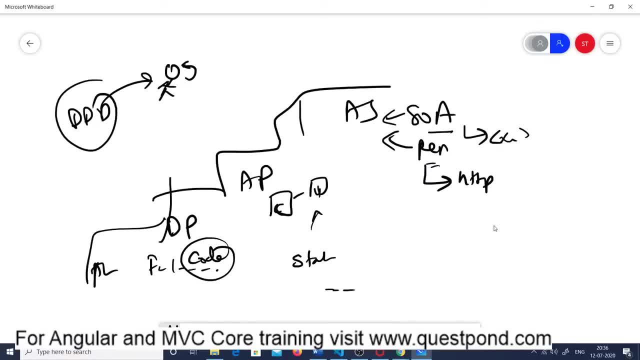 okay, use the static keyword Make the construction Sector private. then do this. implement lazy loading right. so you know some kind of code. when you go into algorithm you exactly know the code. right must be. so I think you know there are different levels. so you can't compare this DDD with SOA out here. SOA is an architecture. 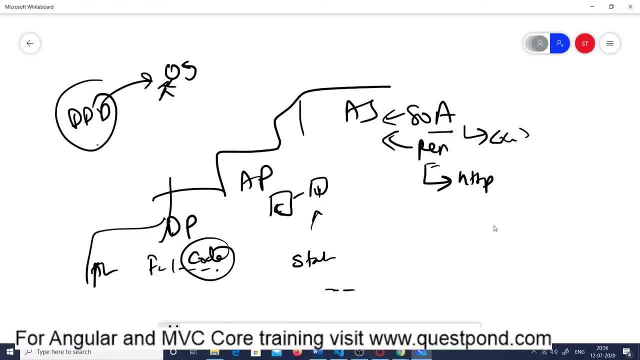 style. an architecture style means it is just one line. we should do it like this and how you should do it. let's say, if I want to implement SOA in Microsoft, I will use WCF. must be or must be in Java, I will use an API, a Java API. so it depends, you know like I will use a Java. 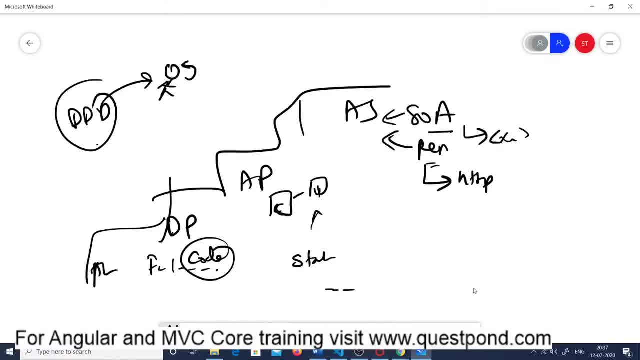 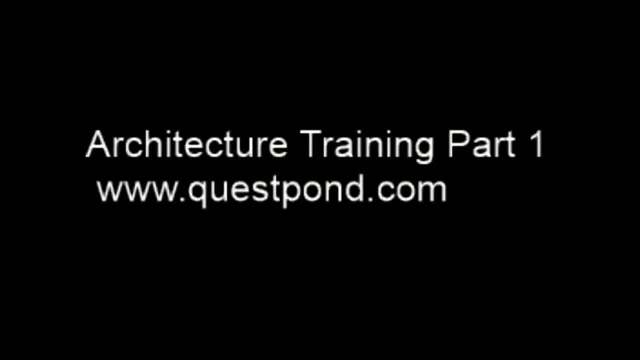 API. so it depends, you know, like, how the technology is, but the point is that it is an architecture style. okay, let me go back out there and let's see the questions. I am sorry. sometimes, you know, I can, I can stray away, because when the question comes up I feel that there should. 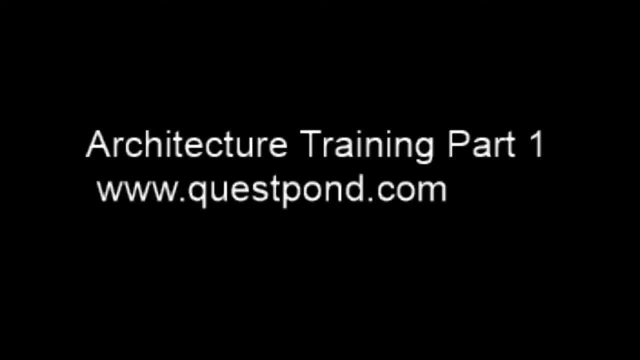 be justice done to the answer? so must be. I sometimes sway away from my agenda. should DDD be restricted to only one domain customer? so let me, okay. I am so sorry. I let me, let me. I have a lot of questions. should DDD restricted to only one domain as a software may be using? 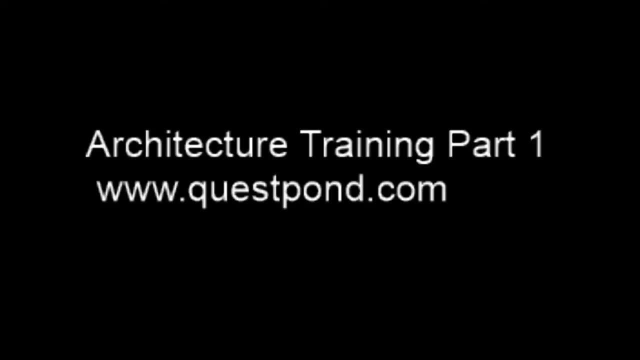 beyond domain boundaries? yes, it should. it's not like domain customer, it's like definitely across boundaries. yes, domain boundaries. I don't know if you are talking about bounded context, I am not sure. but different domain boundaries, absolutely right. but even if you have different domain boundaries, please understand that for that domain you will have domain. 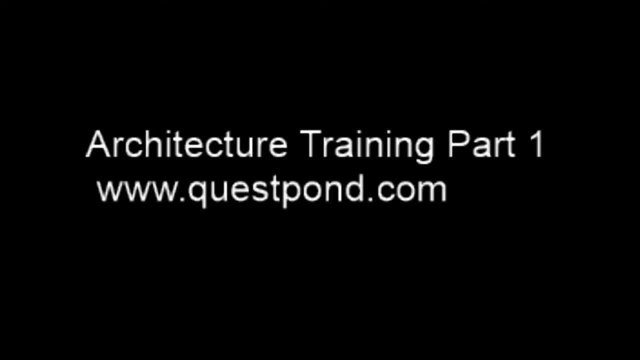 classes again, right, what is the difference between three tier and entire and component? so, Ravi, you can send me a message for this. I will take this question later on because all of these things are synonyms. remember, in our architecture world there are a lot of synonyms: entity, domain, model, three tier and entire must be just the numbers are out. 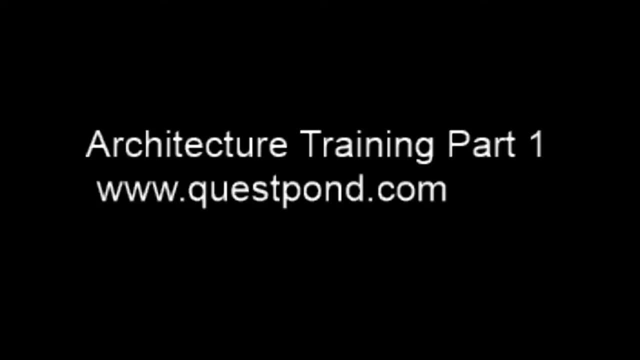 there, right? so some of the things will find synonyms: inversion of control, and when I look at some of those things like dependency injection, I sometimes, you know, find that these are coming from different countries at different times. so must be, must be, it's a UK based English. 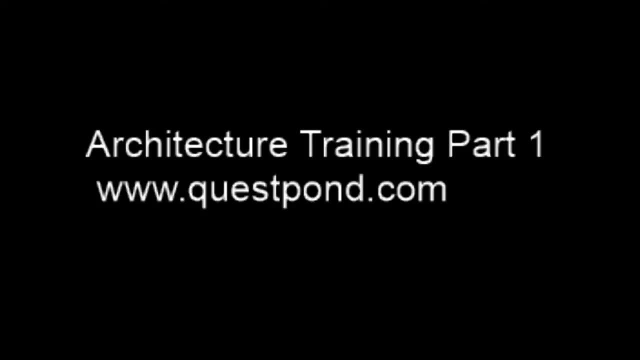 okay, Okay. she talked about inversion of control and then somebody from asia- must be a professor- said: oh, like dependency injection. so sometimes, you know, you find that these words come from different architects who belong to different countries and, depending on their vocabulary, but they all, you will find that they are coming into some kind of synonym out there, right? 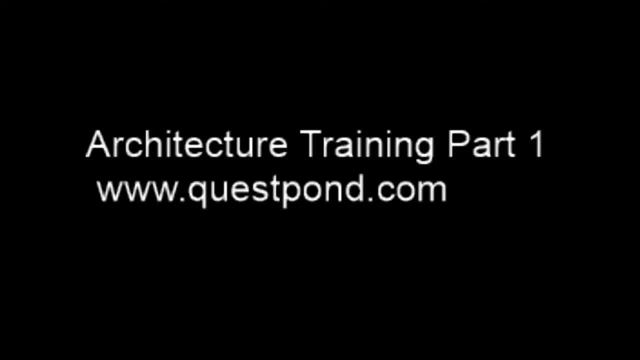 so must be. you can send a separate message to me. i will try to answer it, but here i will avoid this question. uh, how do we consider data transfer? object which has read write properties, dto. data which has read right a dto. i will consider it as a service object. 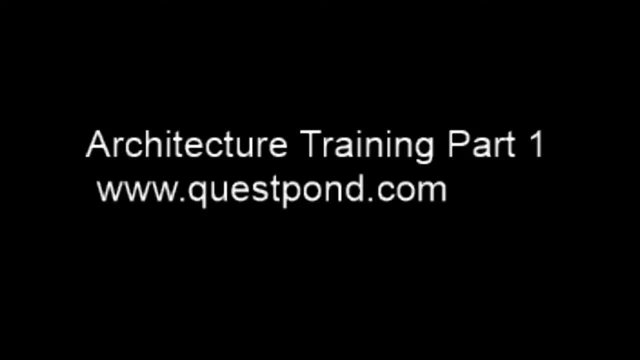 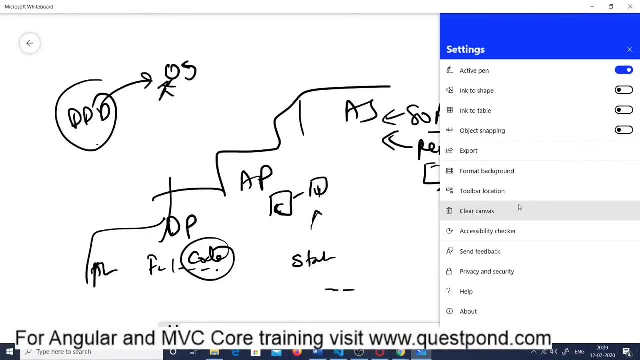 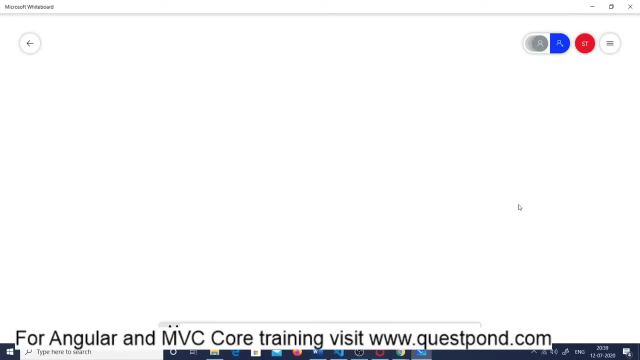 very good question from rajesh thakkar out here. very good question, let me. let me talk about it. uh nicely, uh talked right and remember again. i would like to repeat one thing: do not over learn. for example, today i'm talking about like services and model and domain and 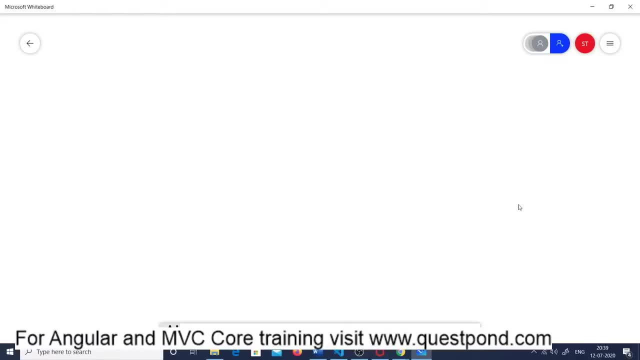 value of data transfer and data transfer of data transfer, of data transfer, of data transfer objects. when you start designing your application, don't ask, don't start thinking: oh, is this a service, oh, is this a domain, okay, is that a value object? don't get too much finicky. 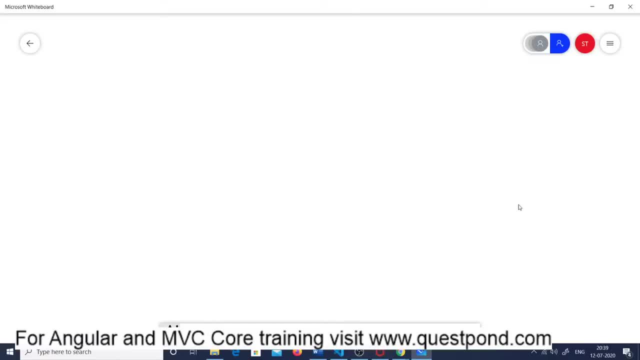 about it. let your naturality come out. focus on your customer, try to give him in his budget, try to give him whatever best you can. you don't take a stress, you don't give customer the stress and just try to see that what best can be done. right so, but yeah, definitely what? 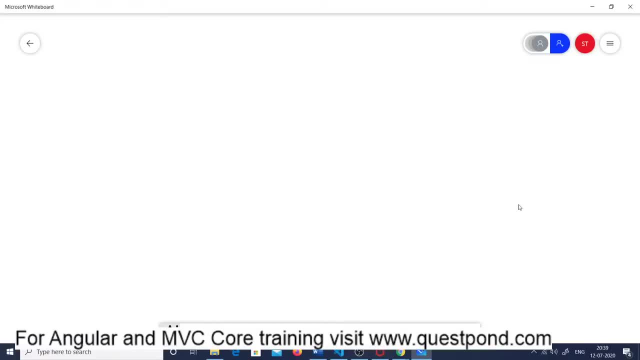 i want is: there are times, you know, when there is budget is not available. there are times when there is no problem, a perfect company out there. i know that there are big multinationals out there which budget is not an issue, deadline is not an issue, but the quality is an issue. 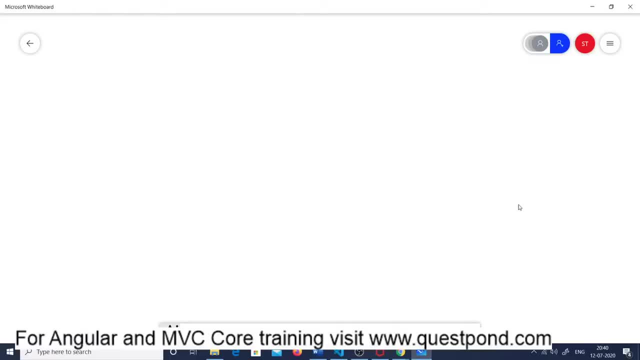 so in those kind of situations definitely you should have that thought process of designing to that extreme right. a question out here: dto must be. some people can say poco or pojo or whatever right false. where is it a service class or a domain class? see, dto is actually. 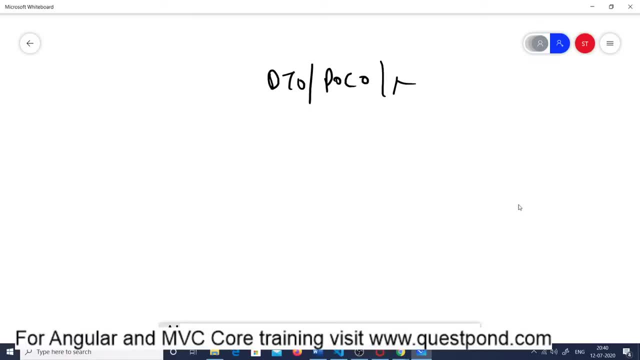 a data transfer object means when you want to send data transfer object, you have to send data from one layer to another layer or from one thing to another thing. you have a data transfer object. so, for example, if you look at the dto, it has only sets and get. for example, 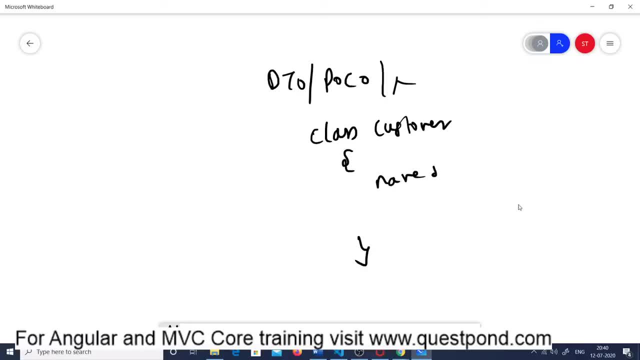 i have a customer class only, name only set. and get why? because i want to just transfer data from one layer to another layer, right? so that means that this is actually spawning layer. so you have a ui layer, let's say a middle layer, a data access layer. then your calling. 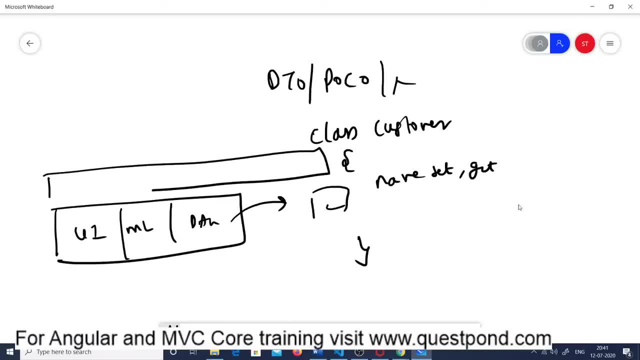 must be an api right across the layer. this is used to transfer data, so i will- i will term this as what you call. i will term it as a as a service layer. think about it. let us say that i am transferring data to online. it is using json, so at that time it is json, but let us say now it is xml. 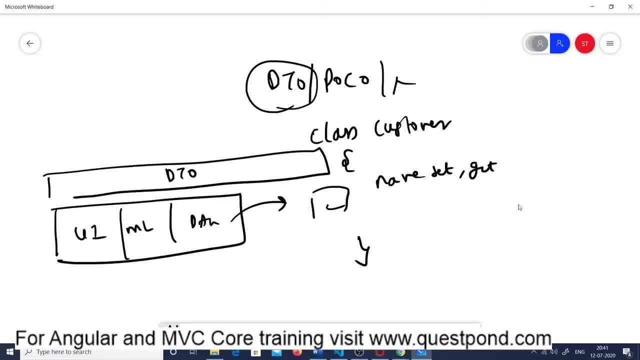 now, if it is xml right, then must be. the structure can change, so it is somewhere. this data transfer is also depends on on the type of mechanism you have, like http, or type of output you have right. so i i find that you know they are connected somewhere with the technical component of the infrastructure. 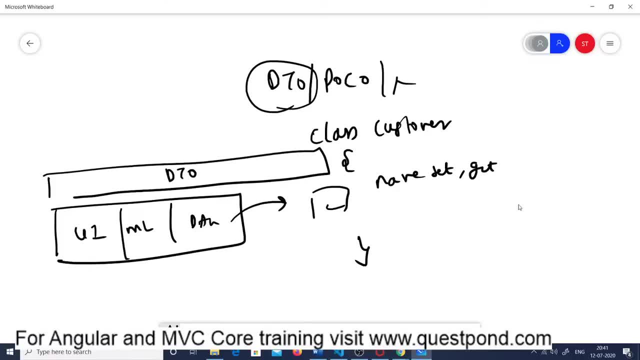 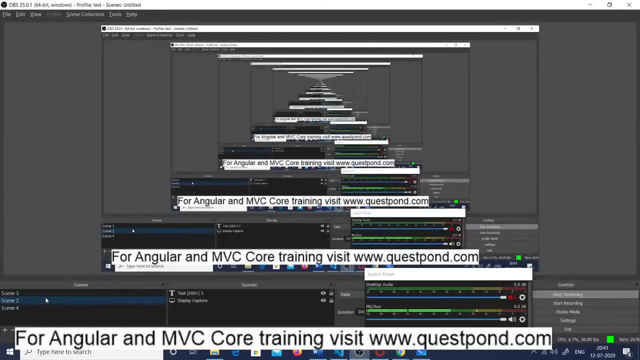 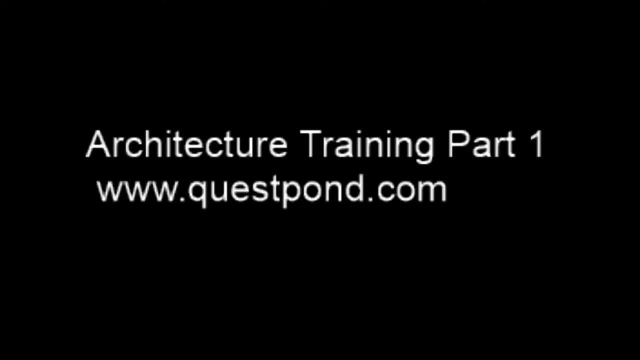 see, remember anything about infrastructure, anything about infrastructure, data access, layer, databases, logger objects, caching and also dto. that means it is a service. that means it is a service, right? so let us go back. good question out there. this one hour is so less. i think caching should be in the service category. yes, kamran, you are absolutely right, sridhar. 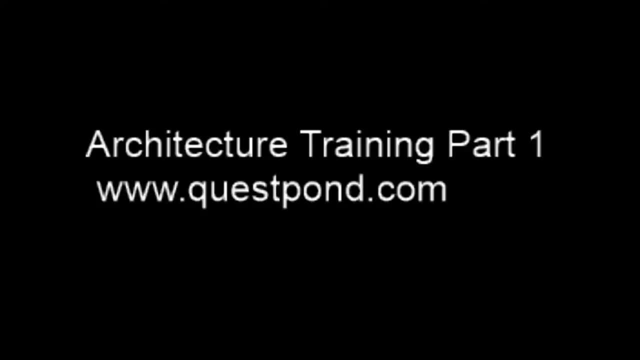 in service class use. model class reference in service class use. absolutely, it's okay, that is the way, actually, sridhar, the service class will refer the model. the model will not refer the service, right? but whenever you change the model then it reflects the service, absolutely. yes, that is right, sridhar. when the service class will refer the model, when. 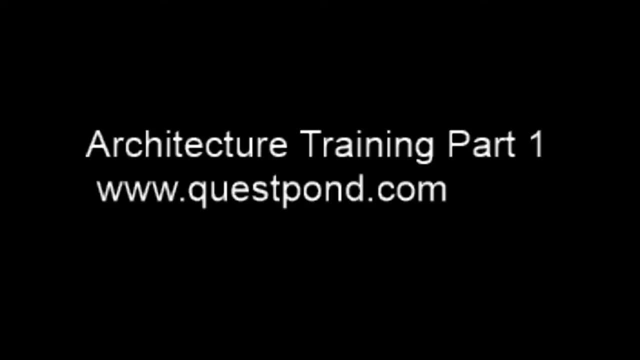 model changes, it will change the service. please note. the model does not change too much. that's where the logic is right, Sridhar. the bank has not changes working. the checks are checks, the aircrafts are aircrafts. the flight is a flight, the air host is the air hostess- right. 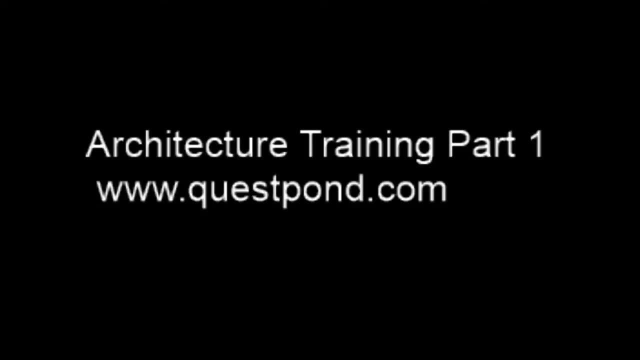 so nothing has changed. what has changed is WCA becoming a web API and web API becoming something else, XML becoming a JSON, like every night, like people are changing the technologies, you know, so that is where the maximum changes. so if that is changing and this, why is this? 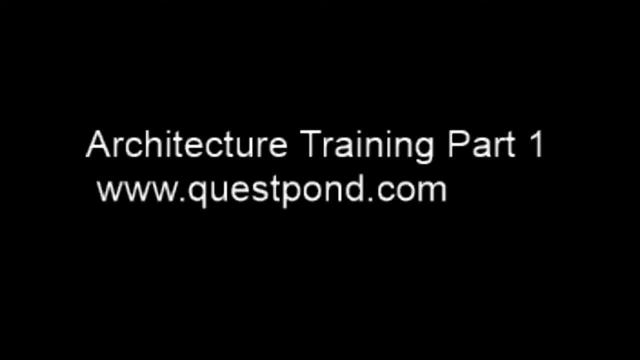 model who is very stagnant. why is he changing? why is he referencing him? so the point of this inversion of control is that a person who is changing too much should depend on others and not opposite way. right, every project should have a reference domain, but how? every project in the same circle and inner circle? would you, sir, please explain? okay, I think. 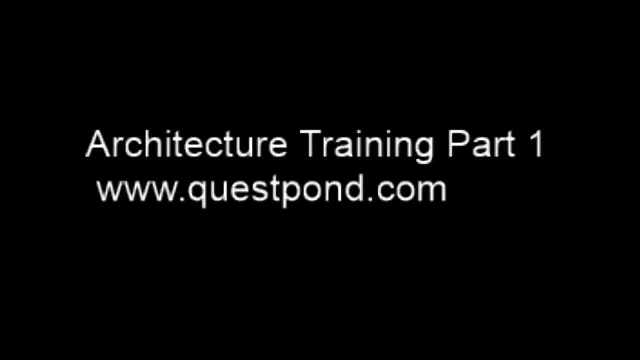 okay, let me take this question of. what I will also do is: let me open up this book out here. ebook. I know that this is the first class guys and lot of questions out there. let me open up this book out here. I don't know if I have it. I always keep that DDD book with me. there is a very good question. 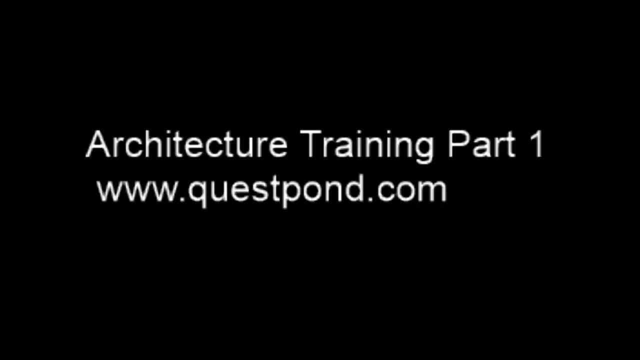 out here that from Taya every project should have a reference domain. very good, but every project in the same circle and the inner circle interact. I will tell you what that thing is. you know, and I think you know must be if we are on the same point out here, so I will go and share this document. 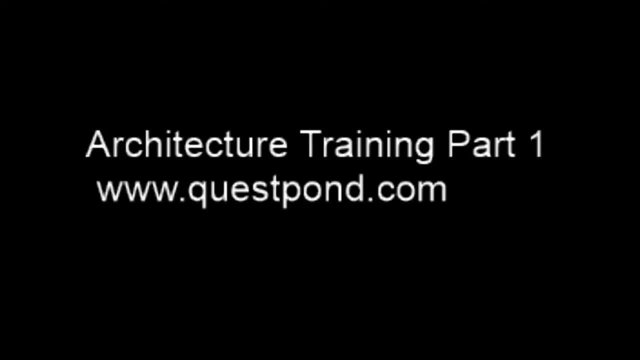 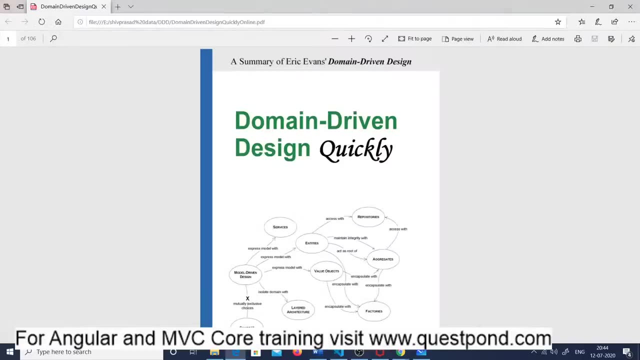 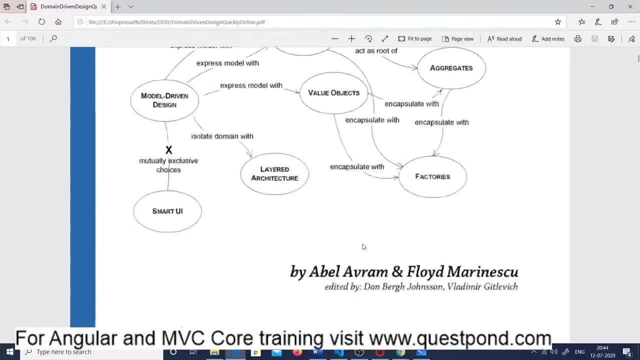 out here. I hope whatever I am sharing out here is completely legal. so this is an ebook which I would suggest everyone to have a look. domain-driven design. remember this is not the original ebook from Eric. this ebook is written, I think you know, by info queue, so 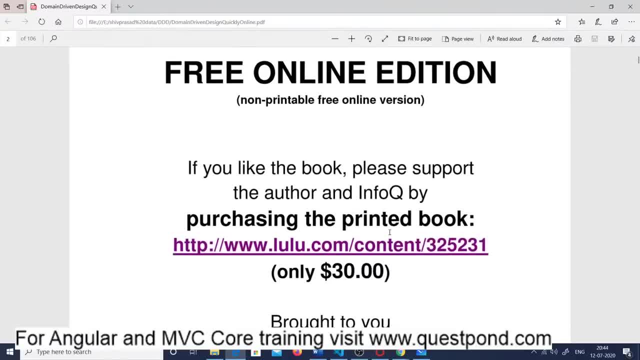 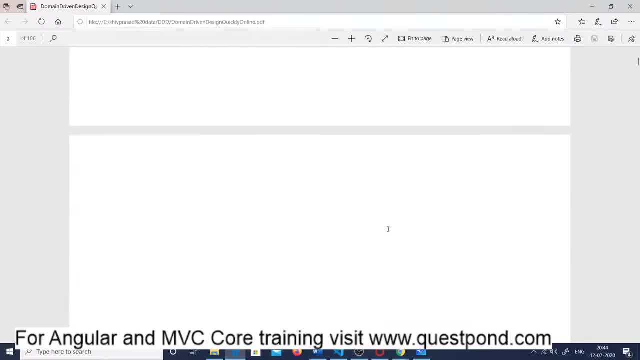 this is a free ebook. it's a non-printable free online version. if you want to go and buy Eric's book, you can go and buy from this out here, or else you can come and attend my class on Tuesday. no problem, right, but very quickly in this Eric book out here. so you 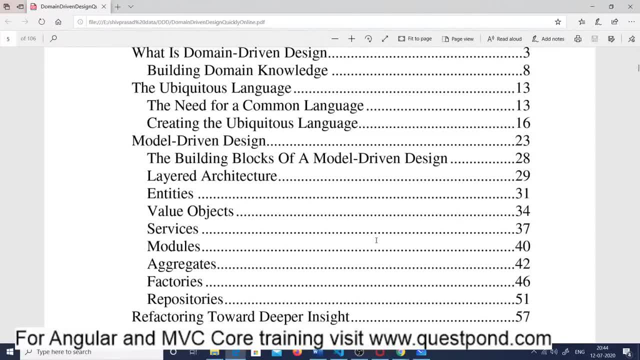 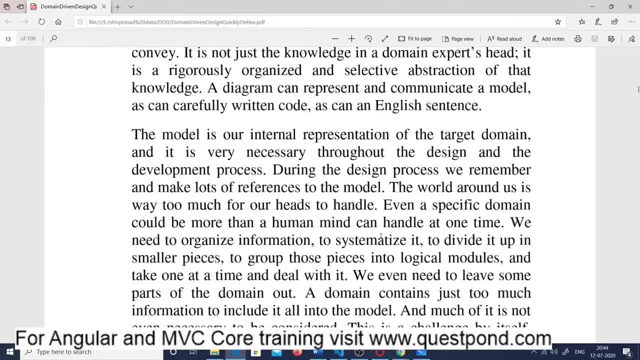 can you, can, you can see out it's a, it's awesome book, it's a story book actually. you, if you go and just see here, you will. you won't find any code. there are text and text and text and text. right, so it's. it's something you need to really get into it. but what I've done 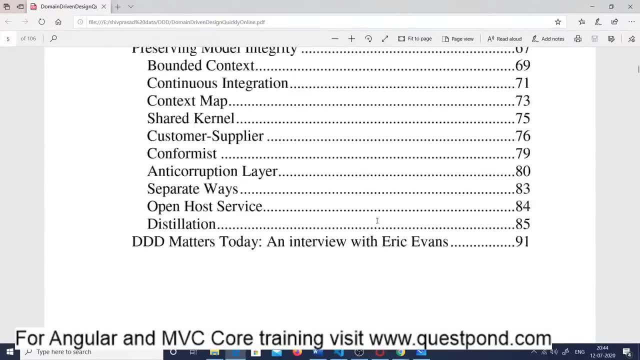 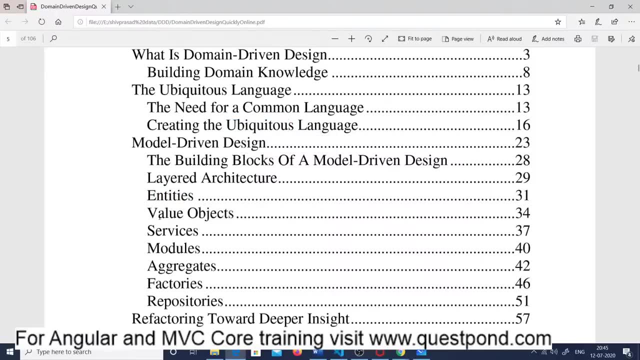 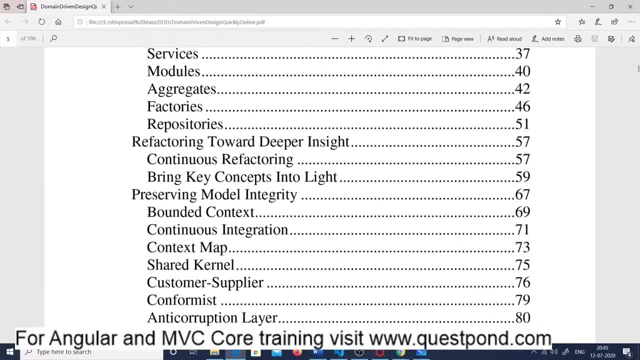 is in today's lecture out here. In my this 50-20 minutes, or one hour, I talked about the ubiquitous language, common language. I talked about entities. I talked about value objects, I talked about services. right, there is one question out here which actually pertains to something called as bounded context: bounded. 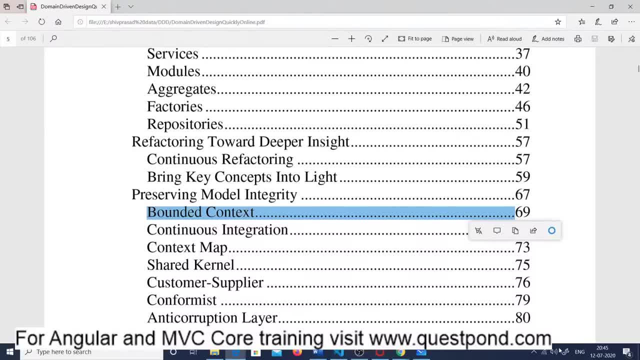 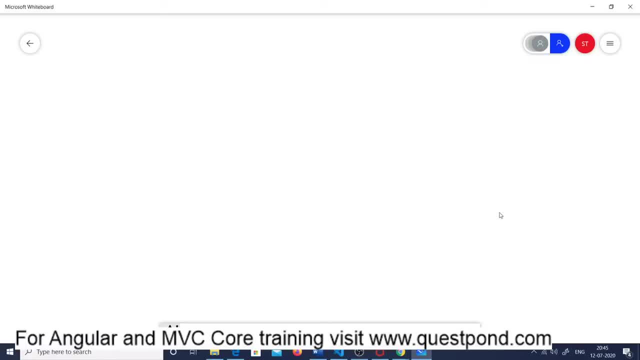 context. okay, let me talk about it. bounded context: you know this bounded context, this bounded context, Long time in history of computer architecting, if I've ever heard this. solid principles. with all respect, I don't feel that if you know solid, you are a solid architect. no, I am from. 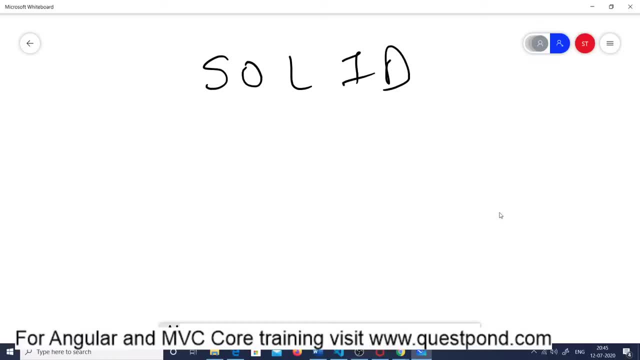 Mumbai. so I know that when person says solid here but that does not make you solid right. but in this solid, you know there is so we can learn solid sometimes, you know, in one of the classes. in this solid, you know, we have something called as Lisko principle. I'm just 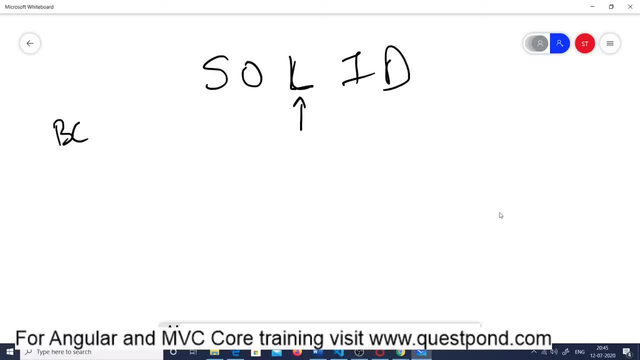 talking about this bounded context and again that question: what is out there right, this Lisko principle? I find that there's a deep connection between this Lisko principle and what Eric discussed about bounded context, what the Lisko principle. Lisko principle says that it looks like a duck, it quacks like a duck, but it is not a. 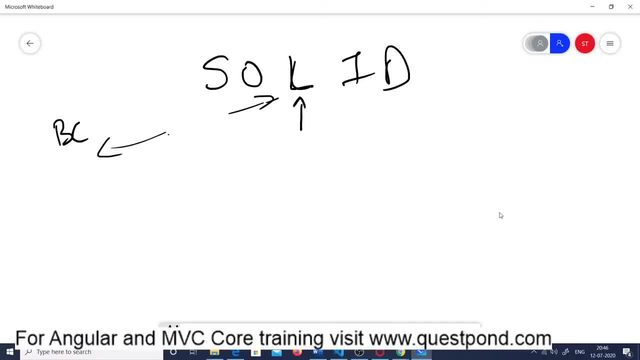 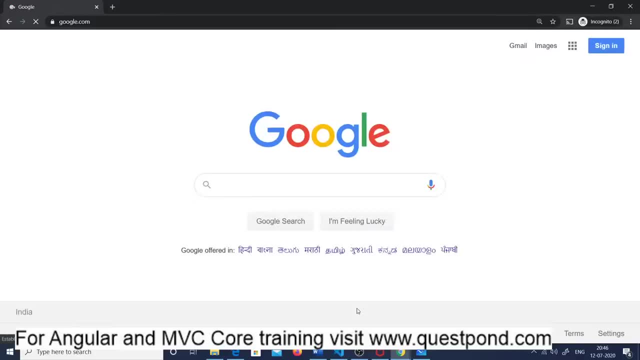 duck. Again, I repeat, it looks like a duck, it quacks like a duck. so if you look at it out here very quickly, to just too sure to everyone, if you ever go and search Lisko subscription principle, which is the L part of your según三 Wisko quoted Etc. 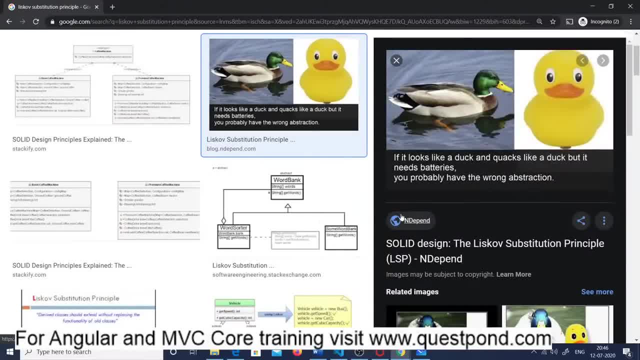 And if you search in images, that's what that famous image is. This looks like a duck. It quacks like a duck, But damn, this duck has a battery. This duck has blood and feathers. It has life. So much difference, isn't it? 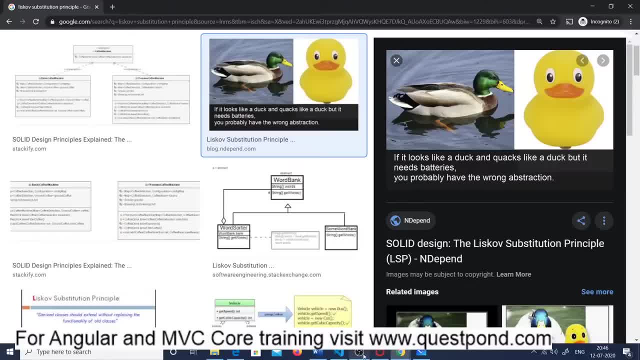 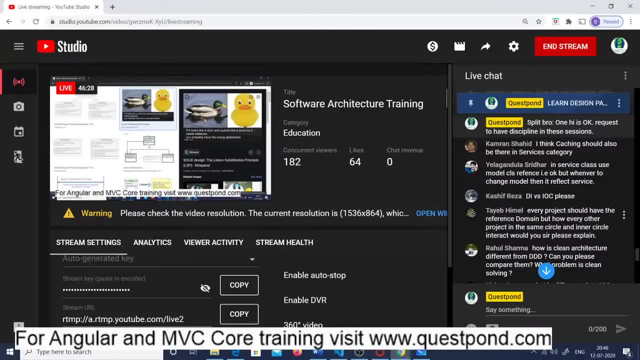 Now, coming to that question, you know which is put out there on the chat. I can just quickly go to my live streaming. Every project should have a reference domain, But in the same project, in the same circle, you can have different things. 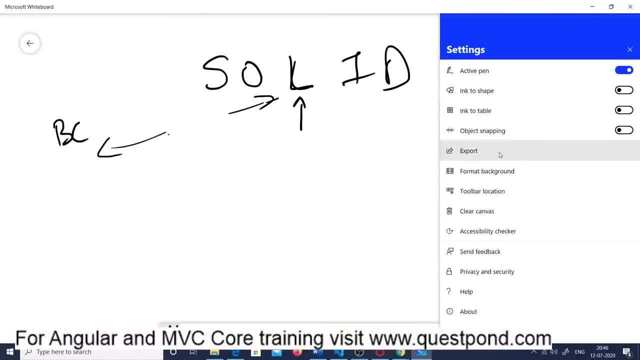 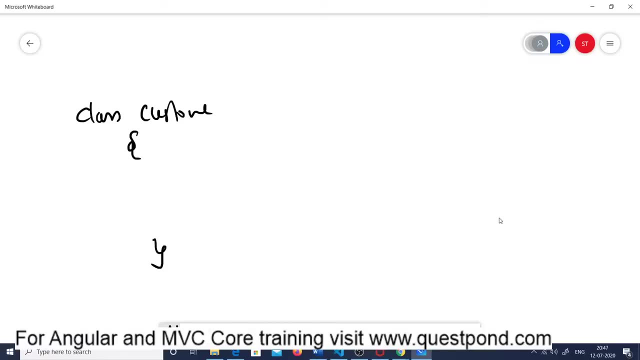 Then you know we are talking about bounded context, Like you should create a new domain altogether for it Means, let's say, you have a customer class- I'm just saying assuming customer- And then someone says, hey, this customer has to be made enter into accounting. 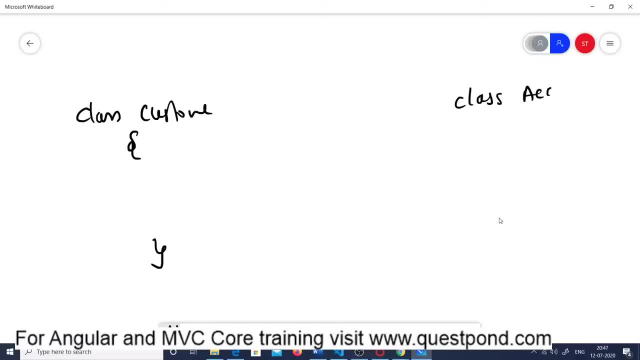 That's what you are talking about? I hope so. Accounting Fine. Now the one thing would be you will say that well, directly reference the customer, Done Awesome. But then the accounting class says that no like. 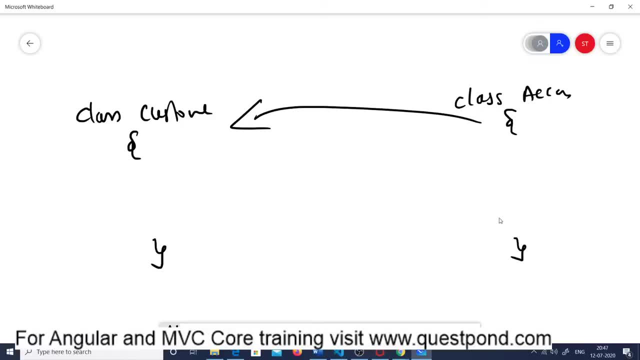 I just need the name of the customer. I just need must be the account number And that's it, Nothing else. I don't need the addresses, I don't need the phones. Now, this looks like a customer, This, so this customer. what you need out here to make a debit credit entry must be: 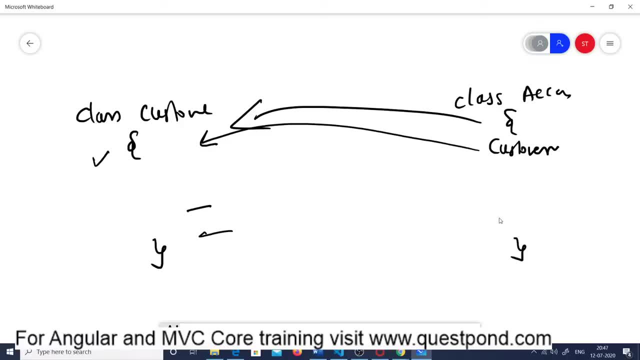 looks exactly same, but it is not same. If you try to reference this directly, believe me, your world will shake off. So what you should do is you should create. create a different class all together. Don't worry about duplicacy. 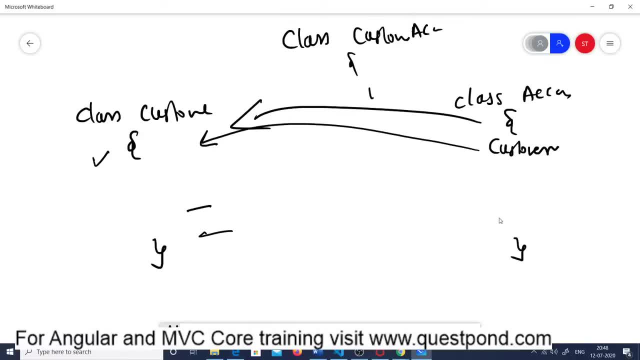 Create a class and say this class is for customer accounting, Separate, Because when the accounting starts changing, he will start changing him and then you have to start changing him. That's horrible Bounded context. There is a context between both of them which looks similar. 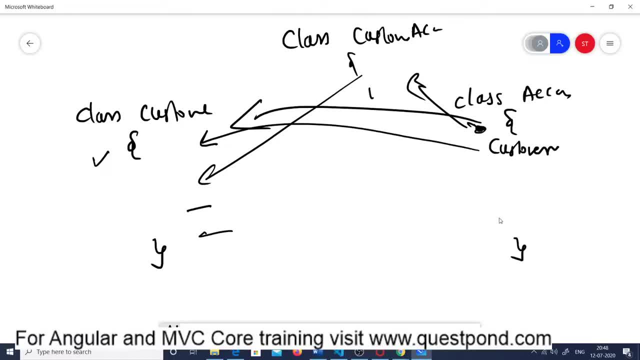 They bind it, but they are different If you look at CQRS and those kind of architecture out there, for example. let me give you one more example. This bounded context, This co-principle, these all come together right. Look at this. 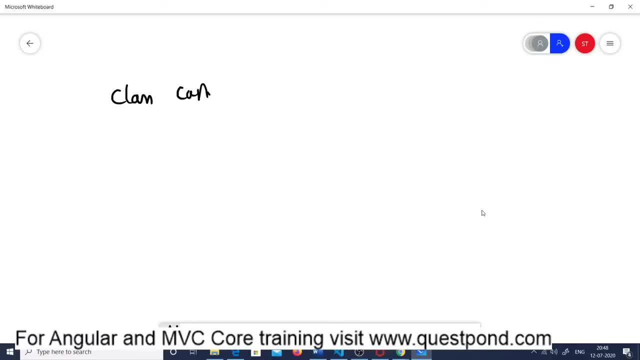 I have. I create a customer, No problem. And let's say I have another domain out there which is for lead management. So I say lead means a customer is a lead. Fine, So you make this customer as a lead. 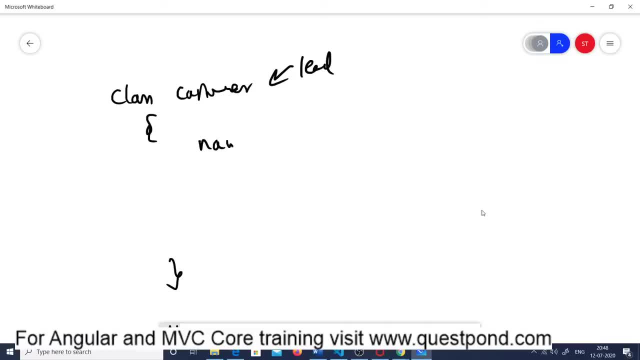 So you start treating him as a lead. So fine, The lead has a name Right. And now suddenly, let's say, this customer has amount. Now you start thinking like, hey, like this lead who comes here, he only does inquiry. 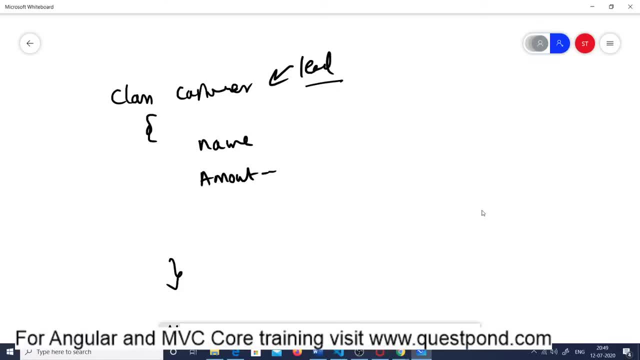 He does have a name, He can have an address, He can have a phone, but he cannot have an amount. Now, you cannot subtract from it. If you try to inherit from it or if you try to make them same, you are then confusing things together. 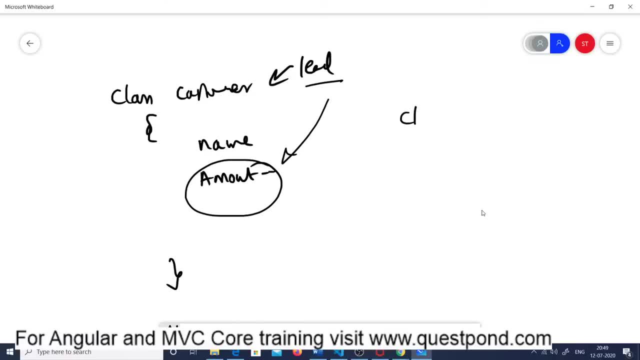 I remember, you know, when I was a junior, I used to create classes like this. I say, okay, like, this is a class customer, Awesome, Right. Then I say, oh, like, let's make it validate, Okay. 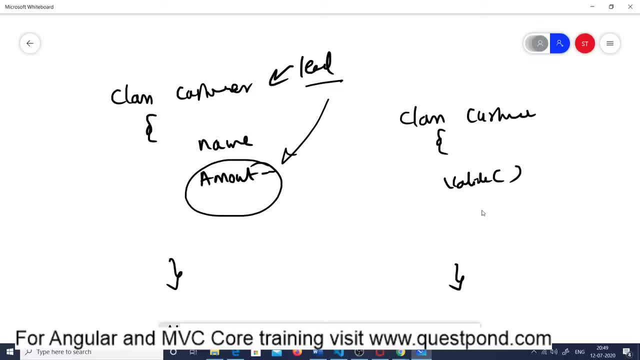 Let's create a validate Fine Function- Very good. Let's use the same customer class for adding data. Fine Add method to add data. Let's use the same class to read. Now, when I used to read out here. 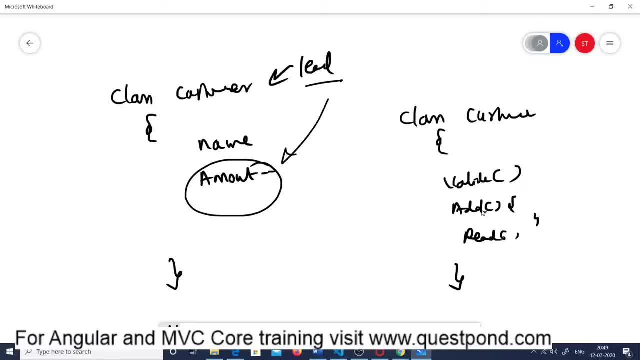 I say: oh, like. read means at that time validation will not fire. So I used to create a property: here is bypass. Then I used to see: property is new, is old, is dirty And suddenly this customer class. 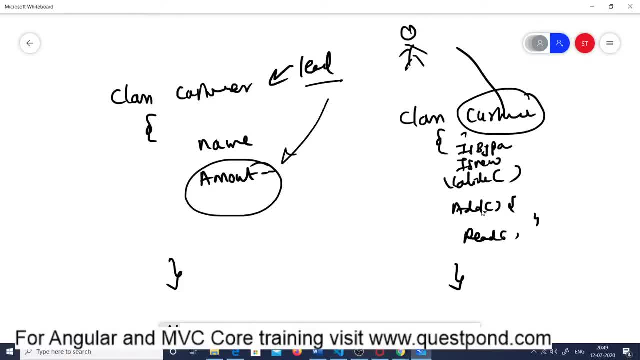 which, when I see a real world customer out here, I don't know that this is new and is bypass and is valid- is anywhere related to it- A classic example of where you are trying to overload a class with a lot of things. So remember that if you are saying that you want to, you have a different domain. 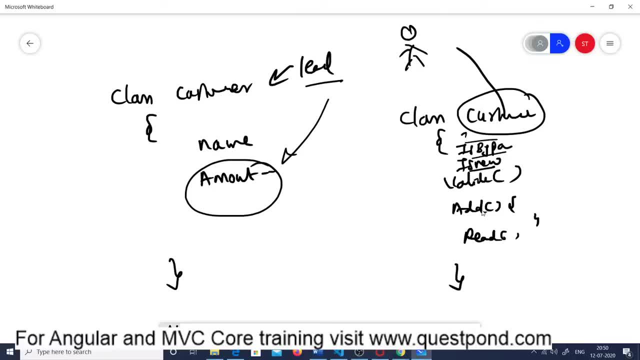 just create a separate class, Just be happy about it, Right? Don't worry about duplicacy. Don't worry about- I know that- how developers feel about duplicate coding, or you know coding again and again, but here it's a different scenario, right? 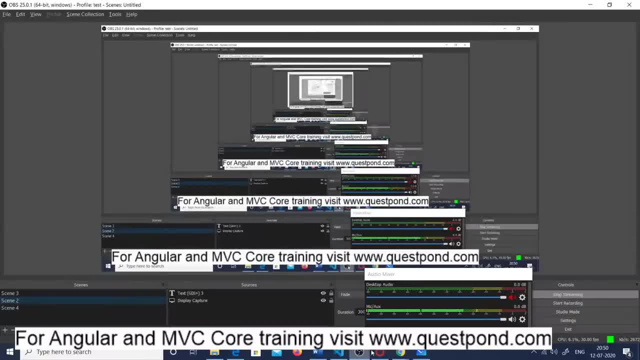 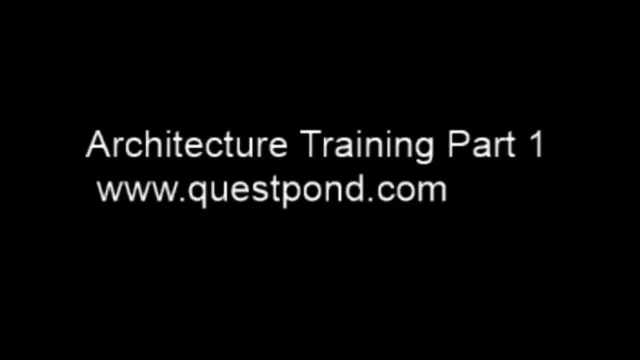 So I would create A different class: bounded context, bounded context- Whatever is the context here, that context is very different out there, right? How? Okay? Uh, I'm sorry for that string away. How is the clean architecture different from DDD? 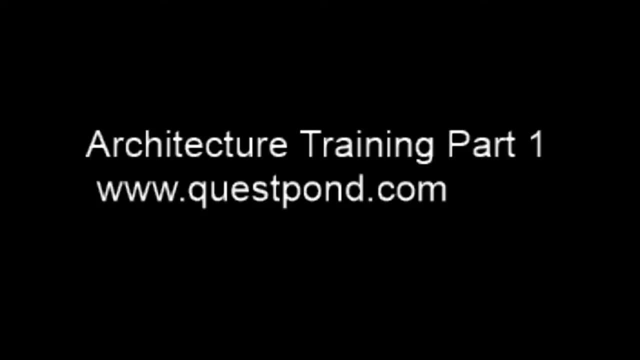 Can you explain and compare them? Uh, Raul, I did not look into clean architecture. Must be. I'll have a look. What exactly is clean architecture? So sorry for that. Uh okay, A lot of questions, guys out there. 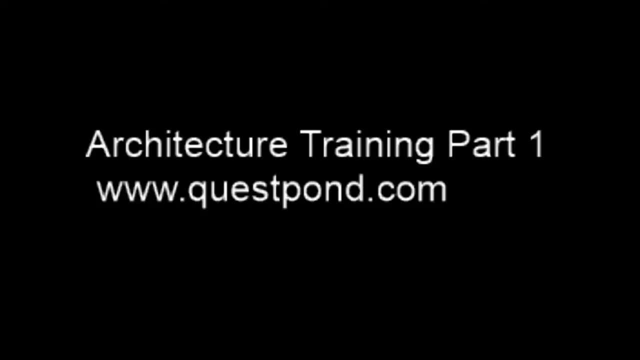 Uh, okay. So uh, I think we have just 10 minutes out here. I'll just uh, uh, take up, uh, take up some questions in which I like: uh, uh, okay, Entity classes can have get set logic. 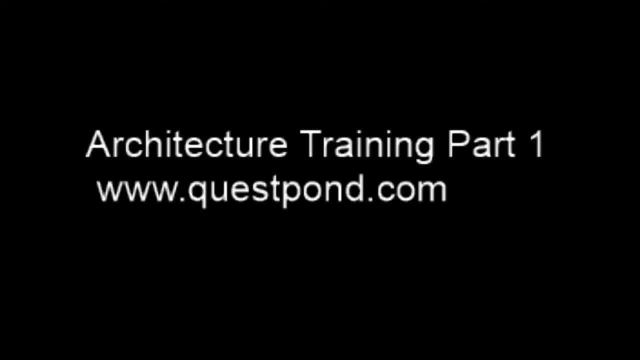 Is this a good practice or not? Very good question from uh. VPN out here, VPN for VPN The other. let me go and share my screen out here. Let us talk about it. Uh, let me again read the question. 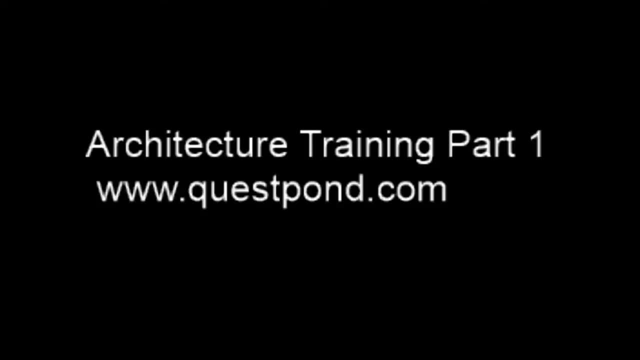 Entity classes can have get set logic. Any validation, conversion et cetera will happen in the get set logic is a good. Okay, That's, that's a very good question. Again, there are two, two differences to this. 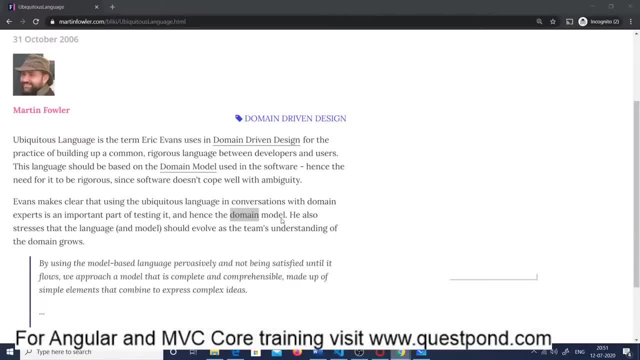 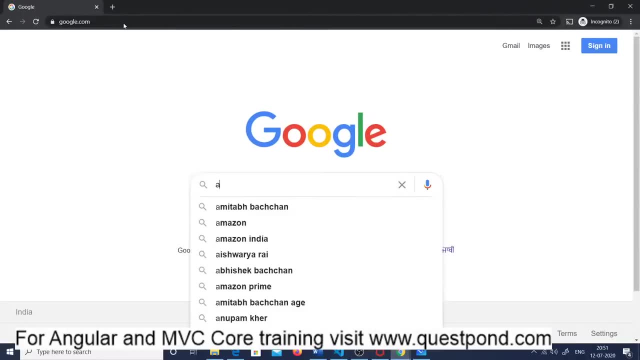 I know I would like to go and point out towards uh, one more jargon. I'll not say jargon, but uh, uh, what uh uh? VPN, sir, you are talking about here is an dynamic model. 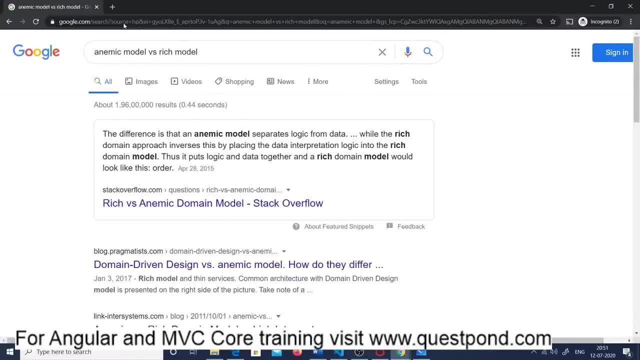 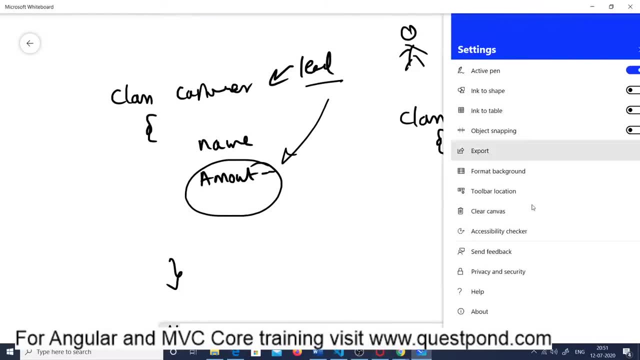 Remember, these are all words versus a rich model, Anomic versus Rich right. Let me, let me tell you guys what the question of VPN, VPN service and, uh, and please let me know, if this is your question, right- What your question is- that you have a class here. 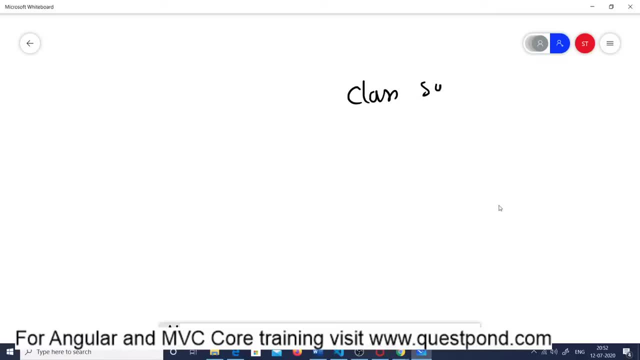 Let me not create a customer class. Now, everybody's fed up, right? A supplier class. Okay, I have a class here called a supplier in the set. Normally developers in the set of the name, they write business logic here If name is null through an exception, if this is this, through an exception, right? 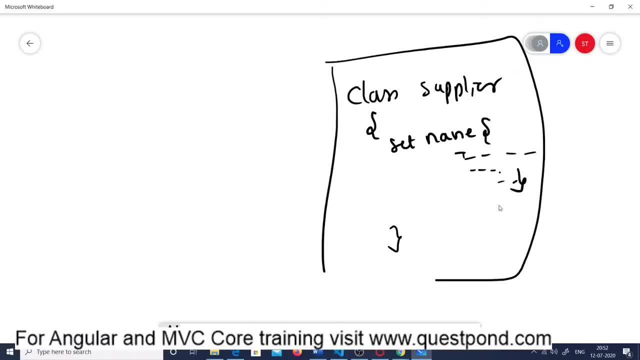 Means what This class itself has: the business logic. The class itself has a business logic. This is termed as a rich model, means your model and business logic is all together: Anomic model. In this case, you will have a class supplier. 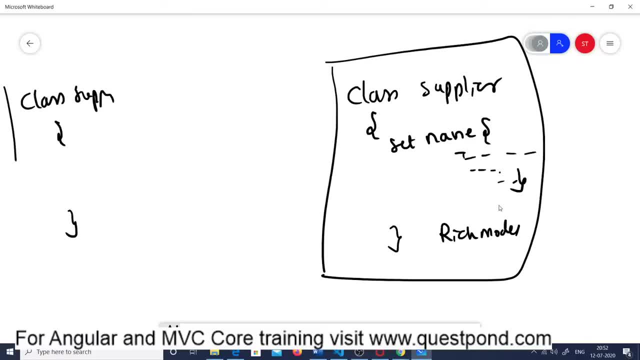 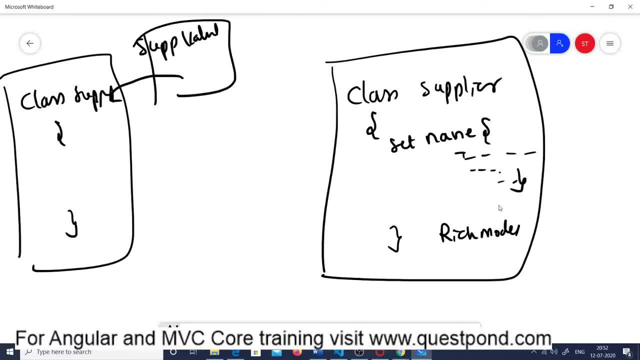 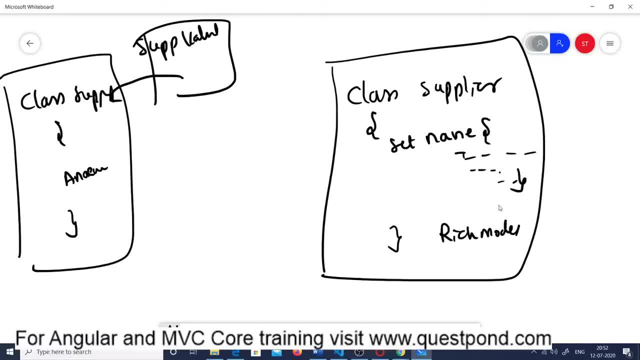 This is called as an anomic model, So means there are two kinds of developers actually out there: One who writes his code like this: supplier, OBJ equal to new supplier and OBJ- dot validate all together. There is another kind of developer, So this is the rich model. 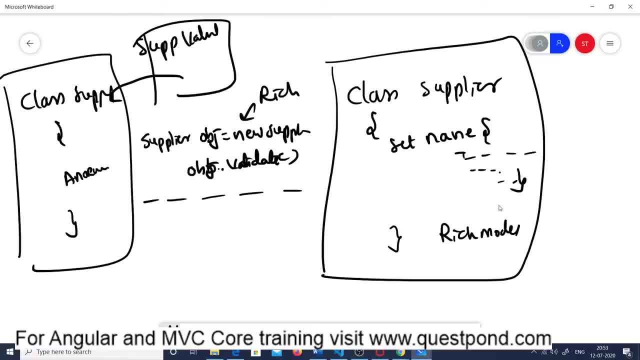 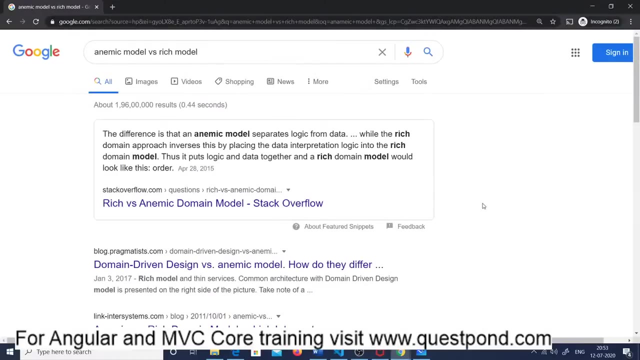 another kind of developer who says, like okay, supplier obj is all okay, but validator object v equal to new validator and v dot validate the supplier object. dynamic model means your validations and your models are separate. now i won't say that this school is nice or that school is nice. it all depends actually. 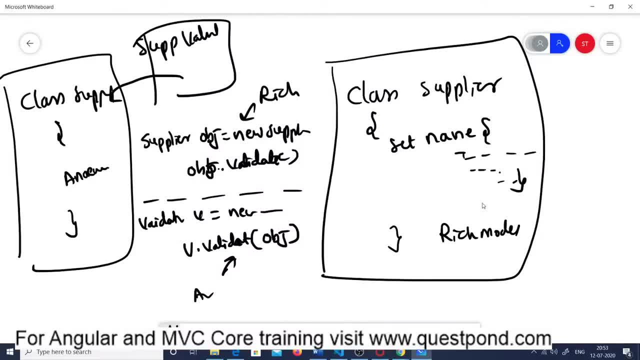 if you look, for example, if you look at your data annotations, if you've ever done data annotations right. in data annotations also, we have a separate class which actually runs on the object and does things right. so this i will leave it to you guys and you can go and you can talk, you can look at. 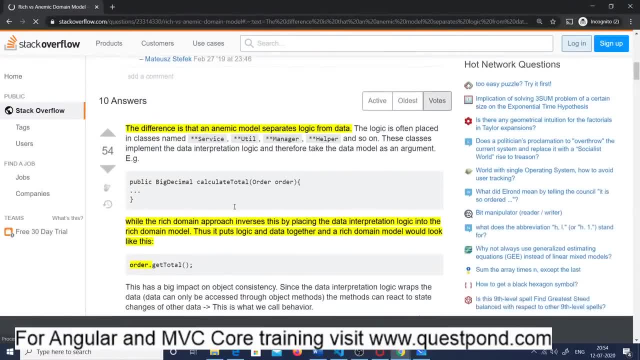 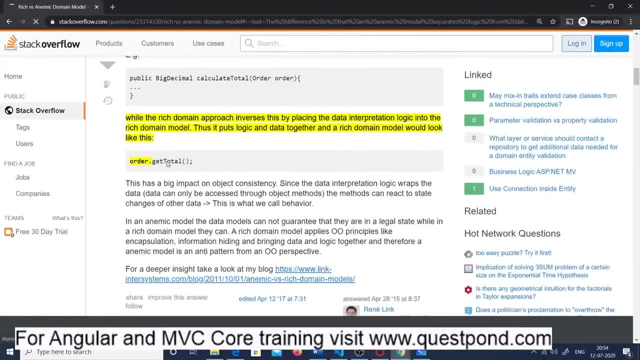 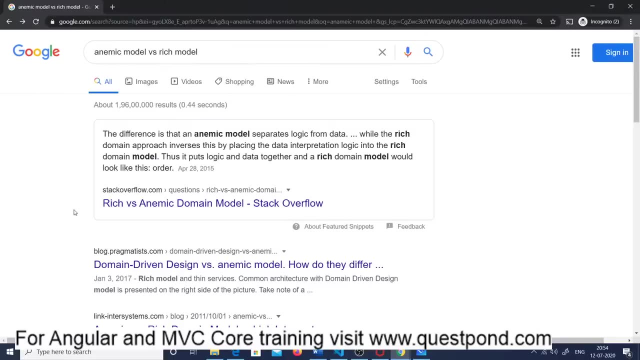 the discussion out here on stack overflow. you can see the discussion out here. the difference is that dynamic model separates the logic from the data, while the rich domain actually is out here right now. i have seen online, you know, a lot of people opposing the anemic model, which i don't go with it, like, for example: 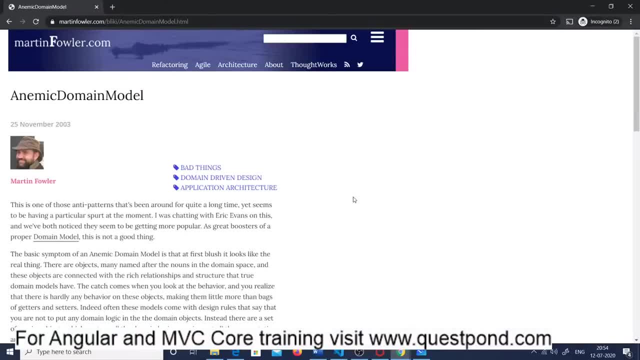 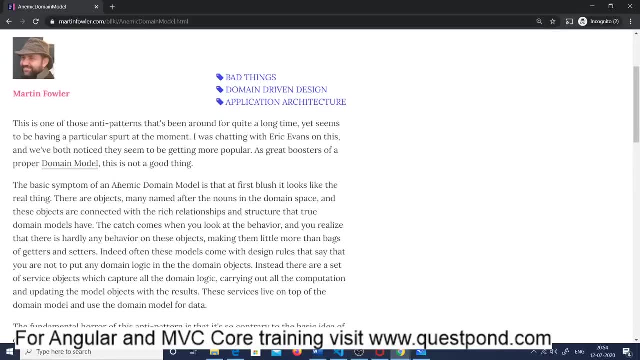 if i look at martin, or even like if i look at eric. you know, when they talk about it they say that rich model is good anemic model. you can see here is clearly said by martin. i'm not saying that whatever martin says or eric says is always the right. 99 they are right. but 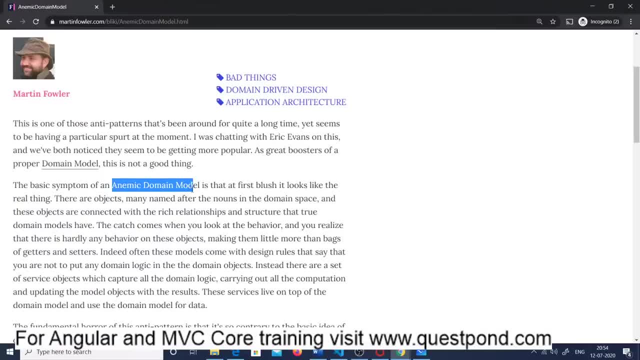 somewhere. i also feel as a developer when i'm coding, you know so, anemic model. at the first blush it looks like very real thing, but according to martin it is not right. but i feel that you know in when i look at the industry, when i work with developers out there. 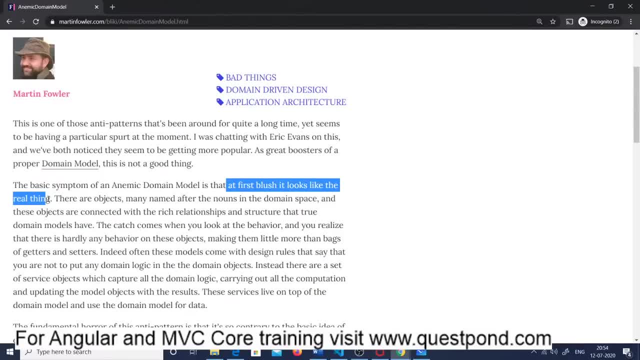 some developers really like to keep their validation logic separate from this. some developers like to write the logic inside this right. domain driven design says that you should have a rich model. domain driven design says that you should have a rich model right. but i go away from this thought process of domain driven design. i say that it is okay to have validation in a. 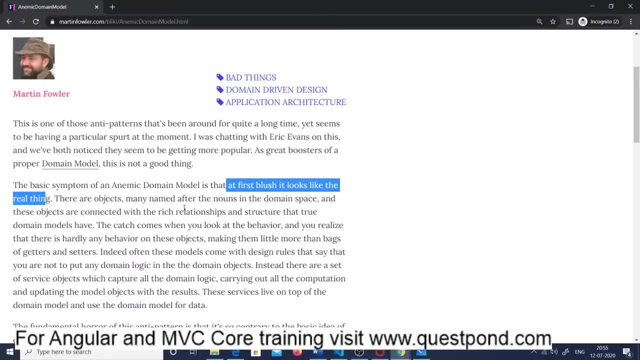 different class, right, and i i feel that it is okay to have a rich model, right, and i feel that it is that why domain driven design people think about it, because when you, when we first learn object going to program, you always says: object has model, it has state and it has logic. so they say that all. 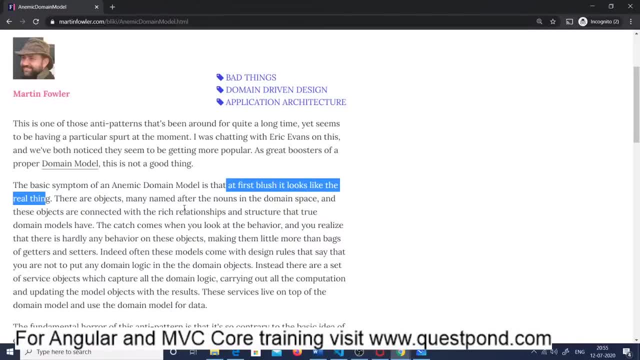 this has to be put together. you cannot have a person who is walking out there, a customer who is walking on your in your company, that the person is different and his, his name is separated right. so it's not like that. so that's why they feel that once you try to plug that logic out of the entity, 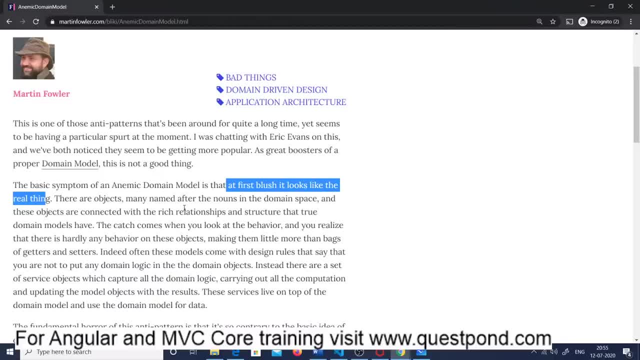 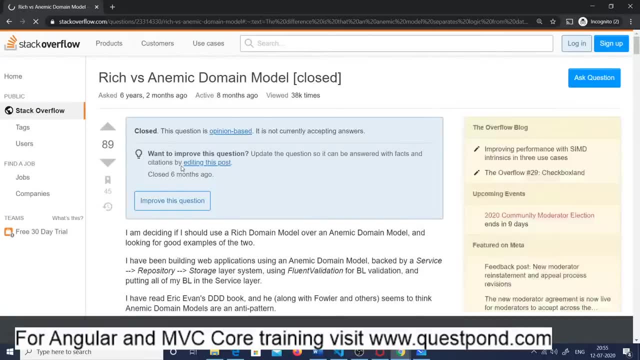 then you are talking about service classes, is it, or what, like you know? so i think you know there is a small uh thing out here, but i would suggest that please once look into the stack overflow discussion. a lot of people also support it, and i feel that where the community starts supporting, 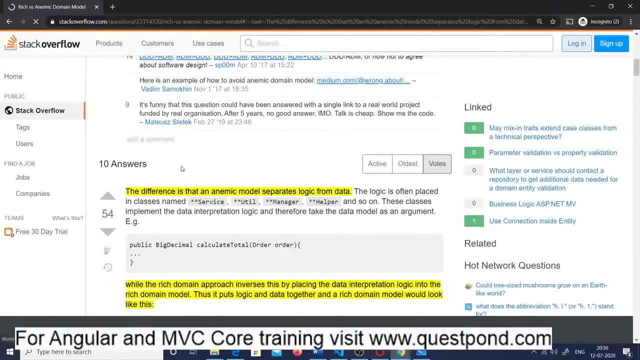 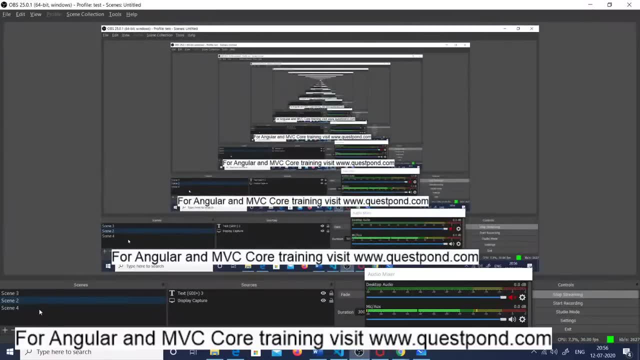 then we also need to retrospect- you know what our gurus are saying, right- and as well as retrospect you know what we have done in our project- and come to a conclusion. so this answer is very difficult out there to give, but i feel that it depends that you are an amic guy or you are a non-anemic guy. 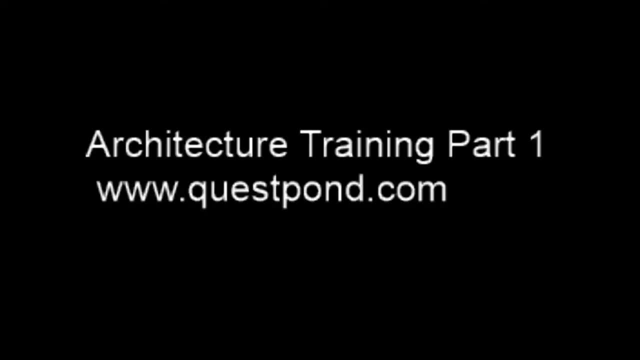 right, okay, uh, ramesh kumar, let me see your question. is fluent api a part of anamic? fluent api is a part of anemic model? uh, no, fluent, okay. fluent validation is a part of anemic model. absolutely yes, because the validations are separate and this is separate. yes, okay, that's good, harshith, you are 16 years old. 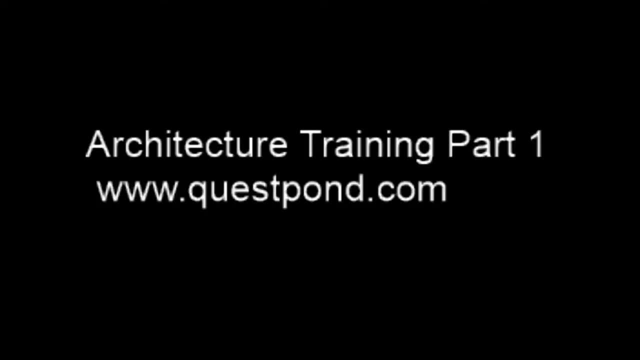 but uh, you are asking such kind of questions. i am so glad. uh, thank you very much. how come someone can identify an experience that is not the case? how can someone identify an experience that is not the case? how can someone identify an experience of fighter and is still a developer or at an? 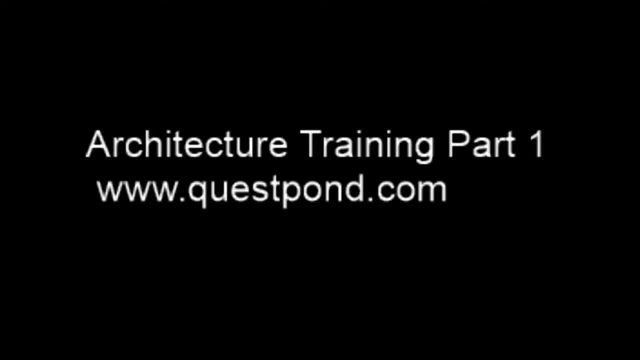 architect level. uh, a good question from rishikesh. we asked here: how can someone identify an experienced 10 years developer is still a developer or an architect? you know that's very difficult actually. so but what i found is, you know that when i see a second or two years, 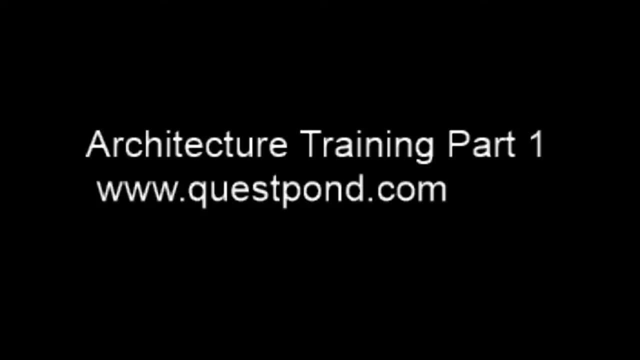 or three years, a kind of experienced person i am, if i am like in a lot of companies i have been a lead and today also i lead some small team out here. i find that the way the other developer codes and the way he codes, you know, i always find that there is kind of uh, following some rules you. 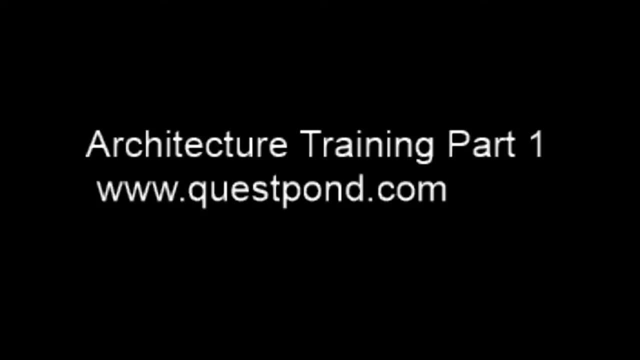 know, like the class naming convention, the way he does his aggregation, the way he does not messes with the design, the way he takes time, you know, to understand things and then codes. i think the maturity part, when you see in a developer also maturity, what is architect? architect is also. 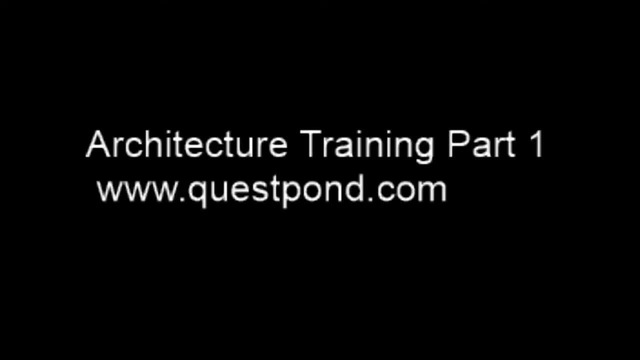 maturity right. so i feel that that developer is a good candidate to become an architect. so i look at more of maturity part in a developer, uh, okay. so, guys, i think it's almost like we have three minutes out here and so many questions. actually, i was planning to 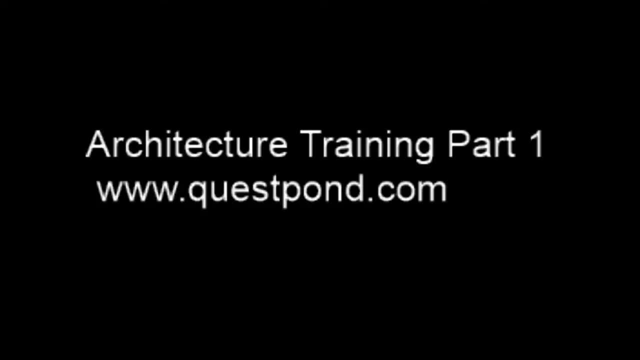 take something more out here, uh. so here it is, guys. um, uh must be. i can have one more session on quest pond on this youtube channel. must be next week. but if you are interested in the architecture sessions, what you can do is you can go and you can share this video anywhere you want on your 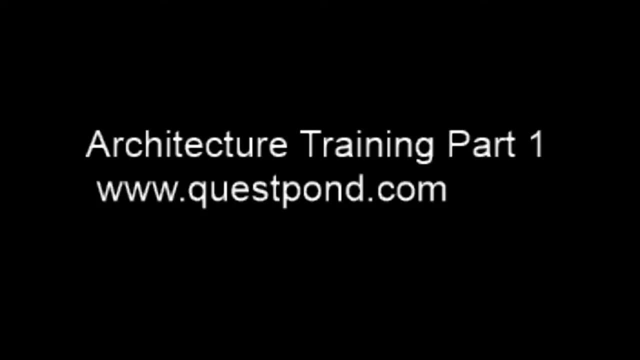 facebook, twitter, wherever right, and take the first two parts of the training free from me, right? so the on tuesday we have the basic training. i'll be repeating the same session out there, but over there i'll be taking something extra right and uh. so my, my goal here is first to start. 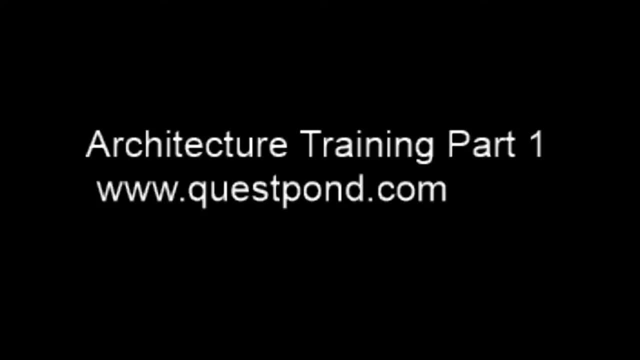 with domain driven design, then to talk about value objects, how to design it using dot net, then i will talk about iterator pattern from domain driven design. what i will do is i will pick up design patterns. so here it is, guys. here is my thought process ahead. so i feel that architecture 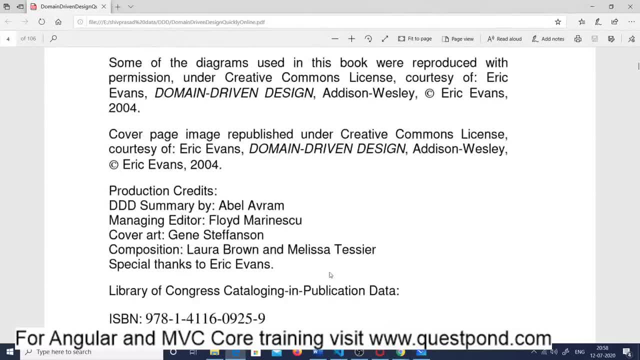 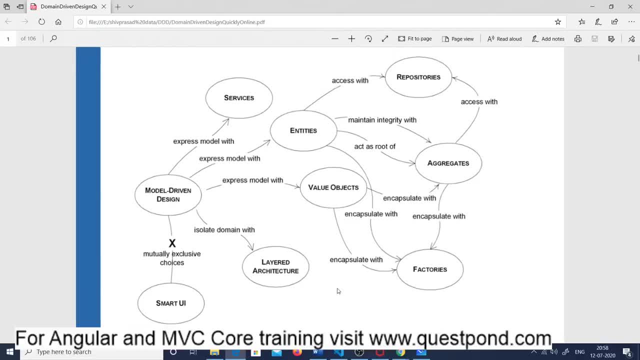 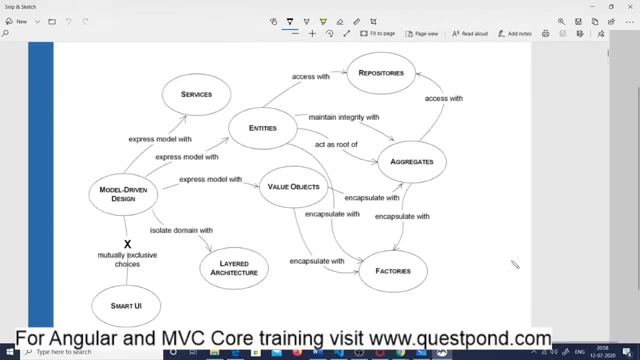 is a evolution, this book out here. i really like this book, this books. there is a design, there is a diagram at the top which really says that, see, remember, you know, when you say that somebody has to become an architect, it's an evolution. it does not happen overnight, right, and i feel that this is the evolution and this 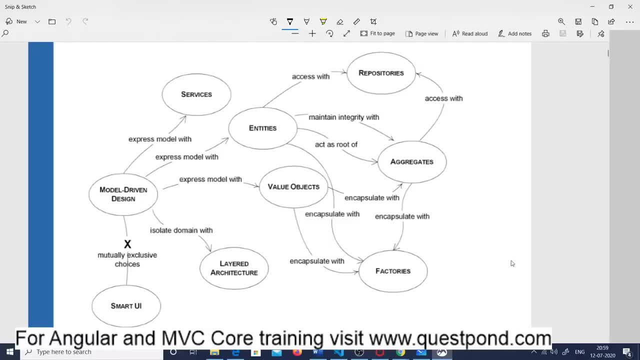 is what i will follow in my class gradually. first is that you have a requirement. out here. from this requirement, you have created entity classes. you have created value objects, you have identified your service classes, right good. now, when you say entity, you will have one too many relationship. when you say you will have one too many relationship, you will talk. 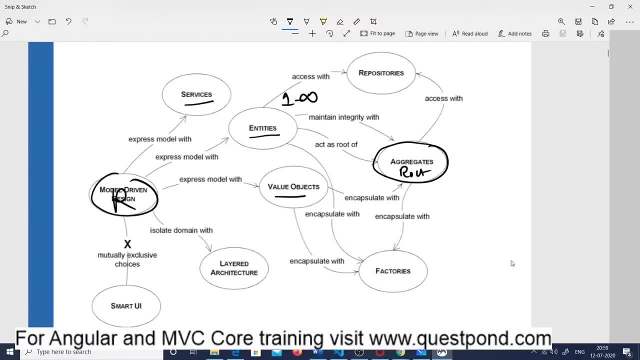 about aggregate root pattern. look at this aggregate root. when you say you have aggregate root, iterator pattern comes up automatically. right. when you say even entities- in entities you have complex object process, you will have factory patterns. right. if you are saying in services you have a cache object. 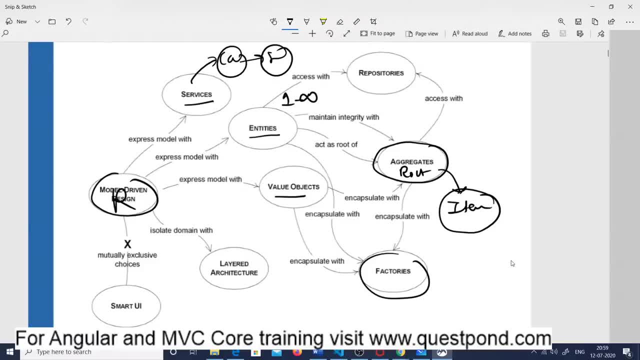 a caching object, then you are talking about singleton pattern, right. so what i feel is the: you know, when we start from domain driven design from there connects design pattern, architecture pattern. everything starts like smooth. so i really like the way area. for example, if you say entities you have to save into databases, repository pattern will come into picture. 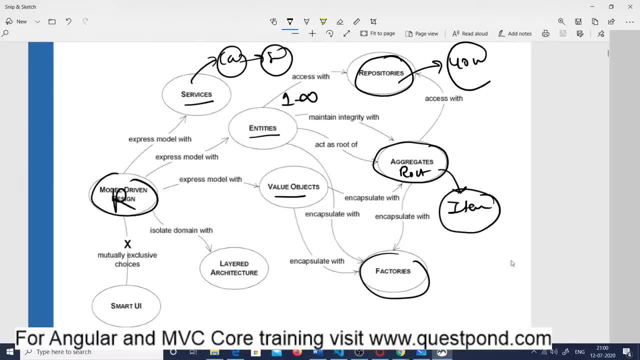 if repository pattern comes into picture, unit of work will come into picture, because unit of work is for your commit and rollback, right? so my goal here in the class is to give you this mind out here to how to think like an architect, right? so that's the goal in the class i, and and 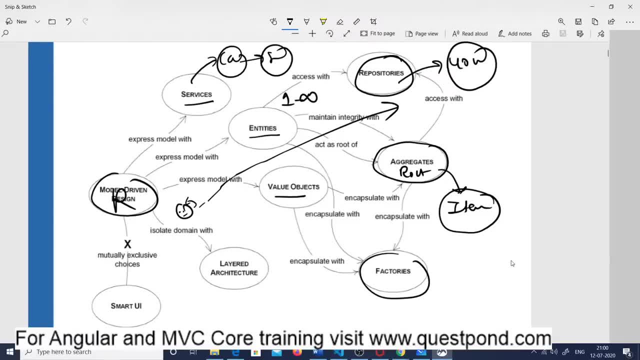 that's why i've kept this class only for one day a week. we'll continue this class for 20- 25 days, one day a week. you will see that when i go to the 15th class or 16th class, i will be just taking one. 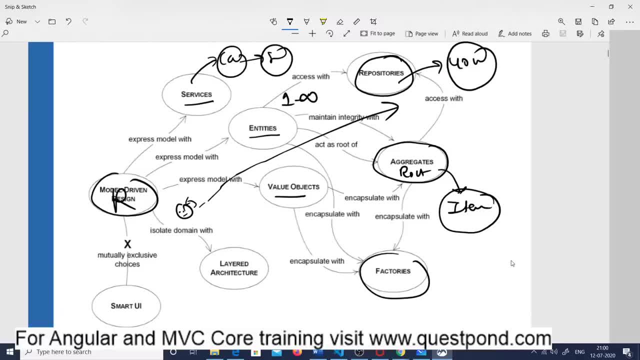 pattern: template pattern. that's the way it will go. template pattern: what are the different scenarios? aggregate root: when should i use it? anemic model versus this model, this and this cqr2 rs versus not non cqrs, right? so i think it will be more of a graduation, you know from. 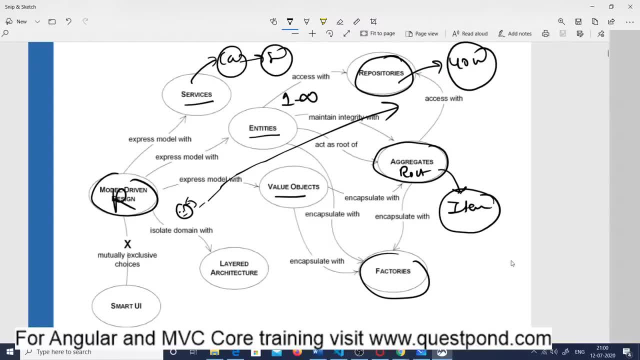 all the different design patterns and the solid principles and all that what you have learned. trying trying to make more sense what i should look as an architect, uml right, what, what diagrams are important and what i why i should not keep in my head it like, for example, as an architect, when i draw my uml diagram. i have rarely used uh, object diagrams. 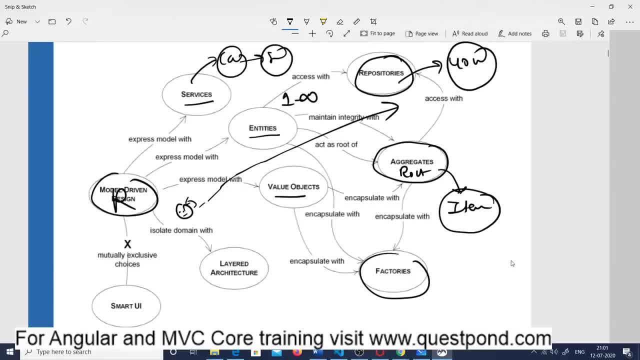 i've rarely used component diagrams. i'm not saying they're not useful. i'm just saying that i have so much in my head that i can't use everything out there. right estimation: i have been using wbs sometimes. i have been using function point sometimes- right. 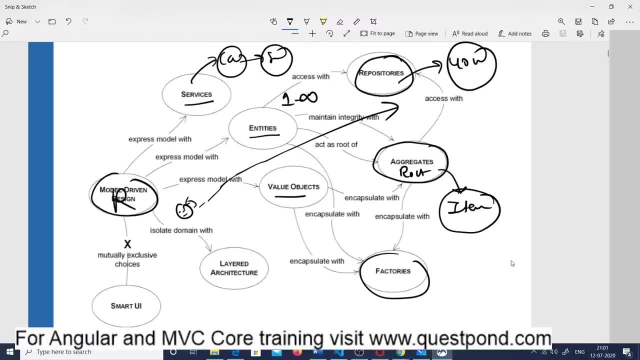 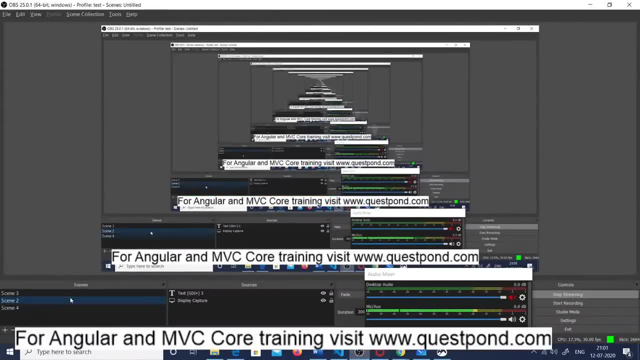 again a different way of looking at when i do agile again, like when i do scrum, how this architecture actually affects that. so i think it's an overall growth out there. so this is my thought process in the class right. so thank you very much guys. thanks a lot. 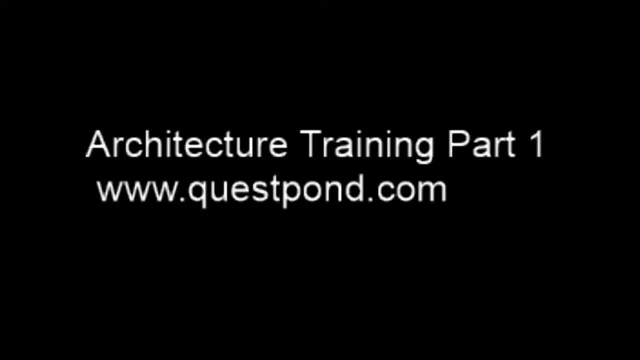 thanks to come to this class. and book name is domain driven. design by eric and from infoqcom: pankaj. from infoqcom you can get this book for free. just i can highlight that book out here, this book. just go and google. i'm sure that you are. 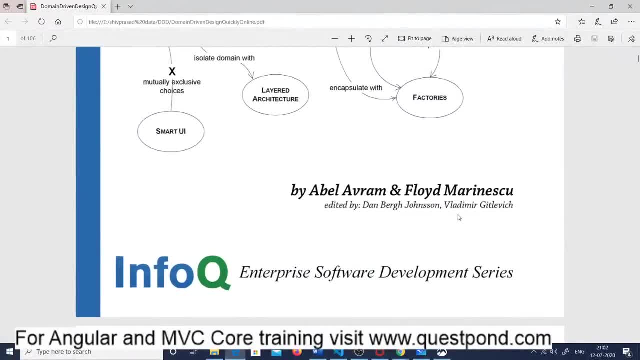 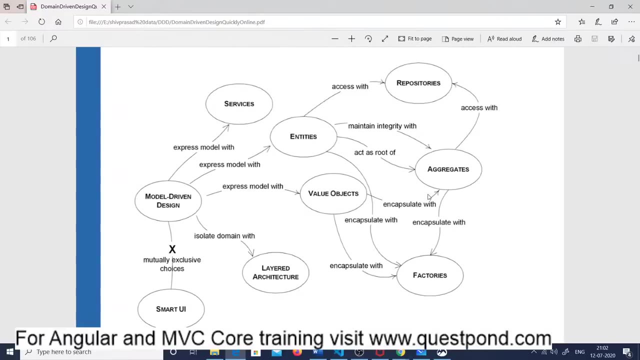 good in googling everyone, so remember that eric is the main person who coined domain driven design, but this book is actually written by, i think by abel and floyd. i think these guys must have just made it more simplified and they have really done an awesome job. i feel that eric book is definitely 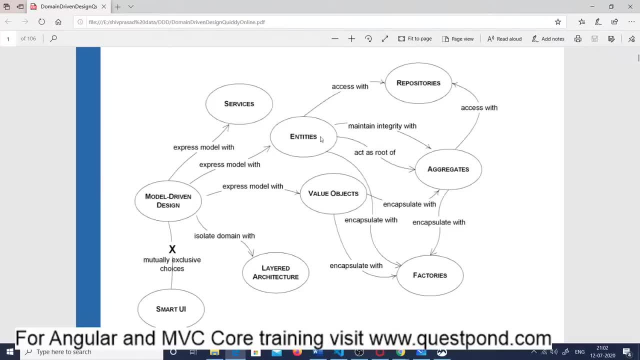 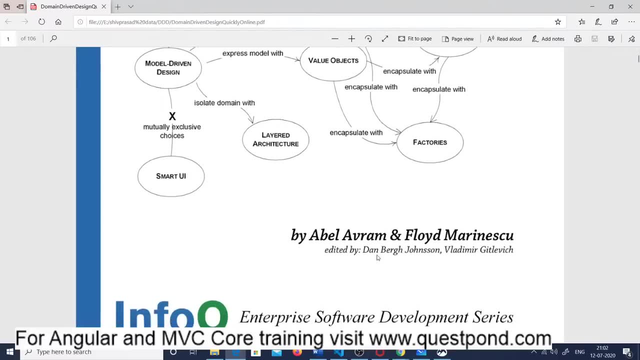 worth a read. you should read it, right, but i feel that you know even this kind of road map. if you put in my head, it makes me think like a developer, isn't it? it makes me think like an architect. so, thanks to abel and floyd, you know, and this is on infoq, it's a free online edition. 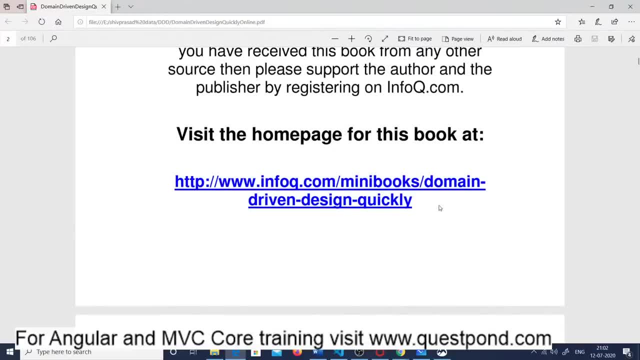 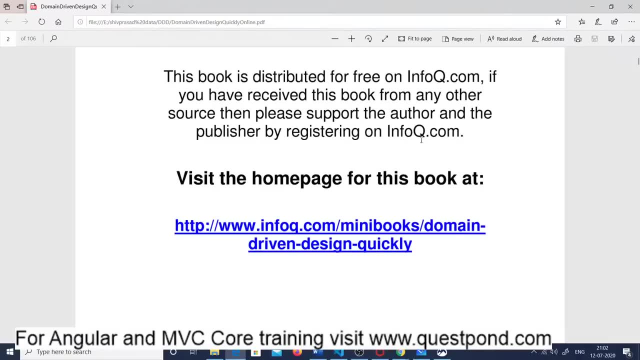 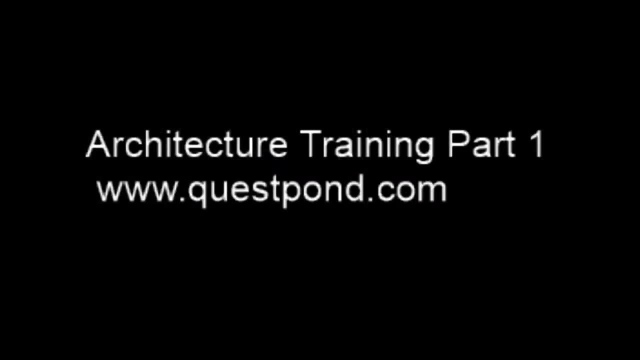 and uh. that's. that's the. you can receive this ebook from uh. please support the author by registering to infoq, so please support them. this book is distributed for free on infoq. please support the authors right, so go ahead and get that book from there. thank you very much, so, uh. thank you everyone. thanks a lot and please share.